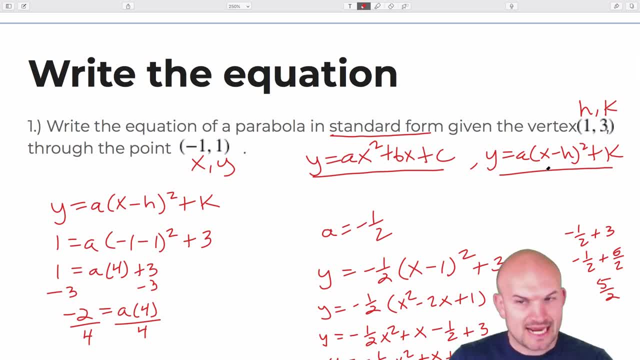 right, But the one important point was the vertex form was obviously with the name of the vertex, meaning that H and K represent your vertex. So I don't really have a way to represent my H and K in this standard form, the way that it's written. So therefore I'm going to, even though the problem is saying use. 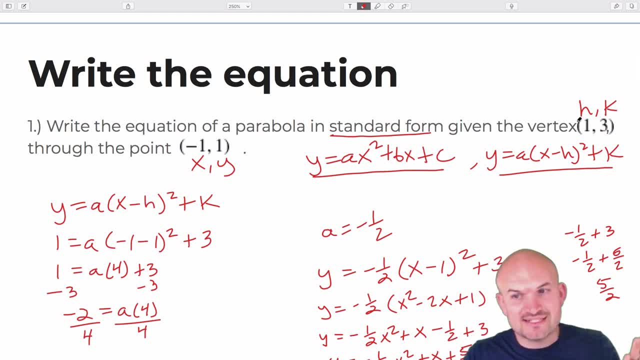 you know, find the answer in standard form. I'm going to use vertex form because I'm given the vertex. So what I'm going to do is I'm just going to kind of label the points that I have here. You can see I have one. three represents my vertex. So therefore I'm going to represent that as HK. 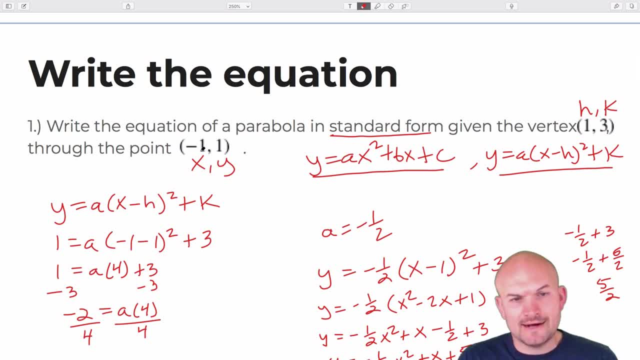 And then I have a point that the parabola runs through. And again, remember, I'm going to use a point that the parabola runs through. So I'm going to use a point that the parabola runs through. Remember, any coordinate point can be negative one one. So in this point I have an equation. 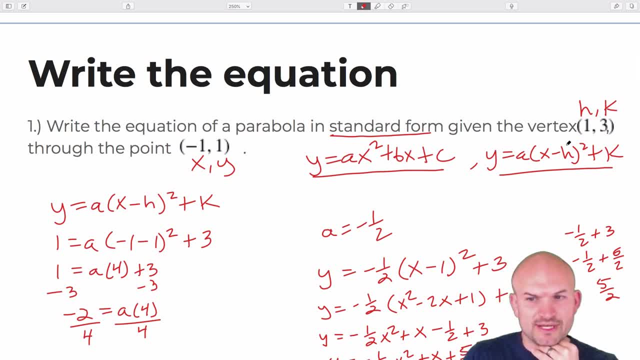 right. And if you kind of count the number of unknowns you have one, two, three, four, five. So we have five unknowns. We have Y, A, X, H and K, right. But again, look at the information we. 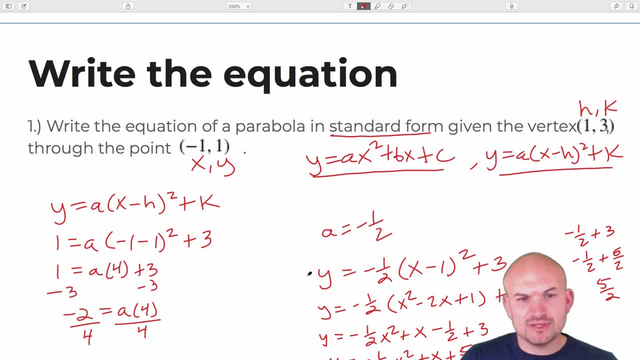 have. We have four givens. So then what I'm going to do is just going to plug in my X, my Y, my H and my K into my form And you can see that's going to allow us to solve for A. 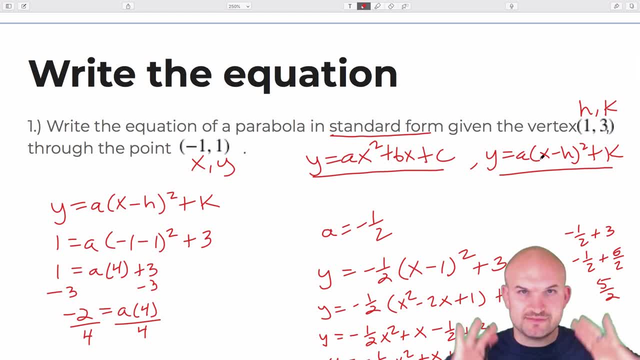 And if you recall A in the standard form, the vertex form that is going to be. you know that's going to help us determine how the, if the quadratic is going to be opening up or opening down, as well as the vertical stretch and compression. But either way, I'll just plug. 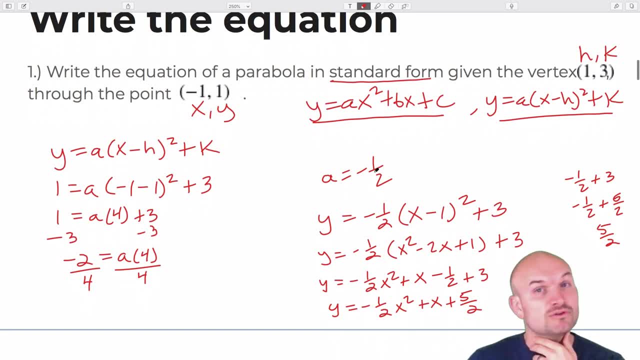 in those values and go ahead and simplify, I get A equals negative one half. So now I can write the formula in vertex form: right, So I can just plug in negative one half in for A and then just plug in my H and my K. However, the question was saying: find this in standard form? 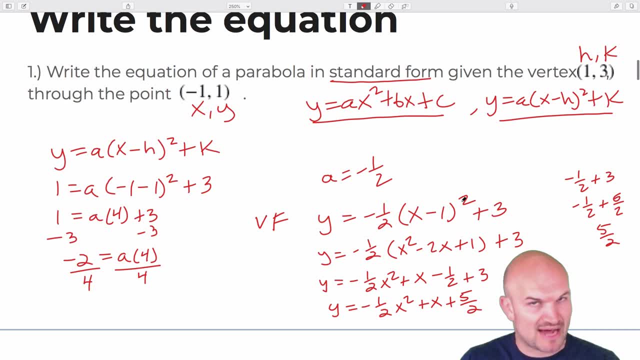 So what I'm going to need to do then is expand this And notice this binomial squared. When I expand that out, it gives me a perfect square trinomial. I distributed the negative one half, And then- the only thing that was kind of a little tricky here- 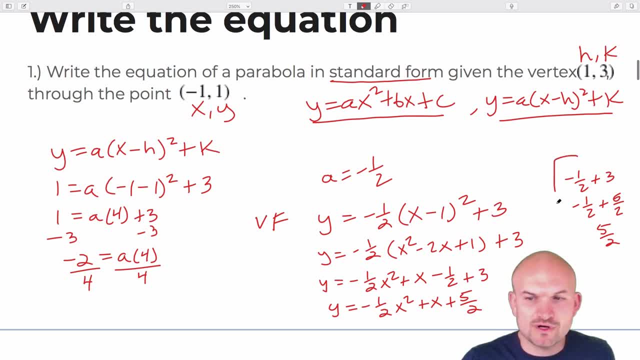 was to add a negative one half plus three. But you can see, I kind of did this work as a little sidebar over here, Just to remind you, you can write three as a six halves and then you can combine them And that's how we got to five halves. Now onto some definitions. So the vertical 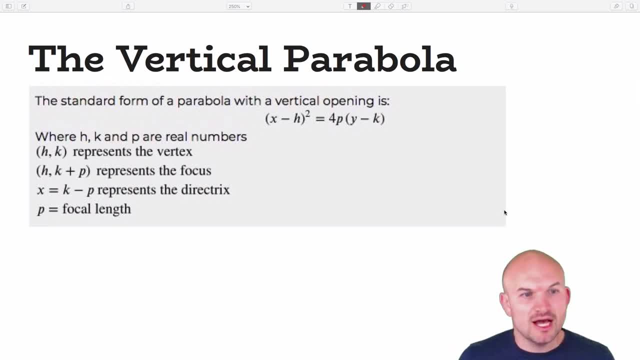 parabola- basically the quadratic that we're most familiar with- also can take on a new standard form, which is in the form of X minus H. squared equals four P times Y minus K. Now, this P is something that we talked about. 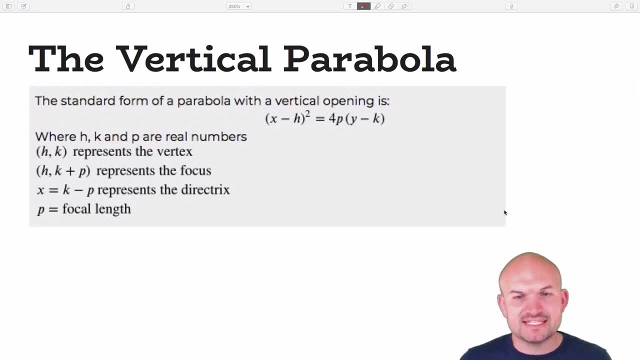 last section, We didn't really discuss what it meant, but basically what we did is we just kind of like described it as like: oh, here's this new variable or this new number that we are going, or this new variable, yeah, this new value that we are going to be incorporating. 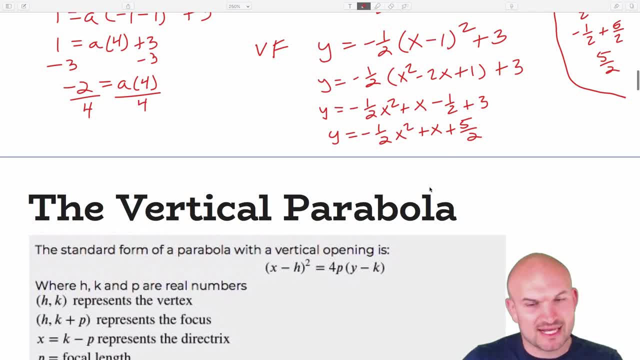 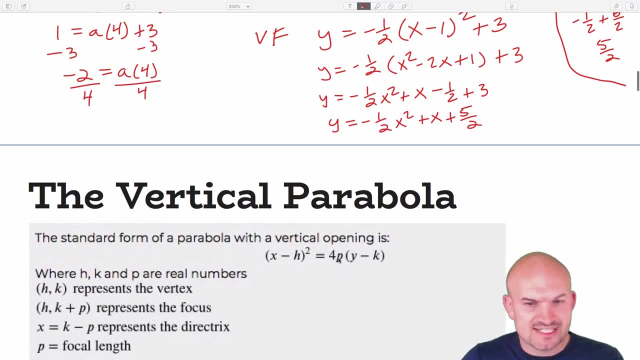 So it's very much related to these. I'm not going to get through these relationships here, but you can definitely go ahead and just rewrite this and well for Y, and therefore you can see how that four P is related with your traditional A. 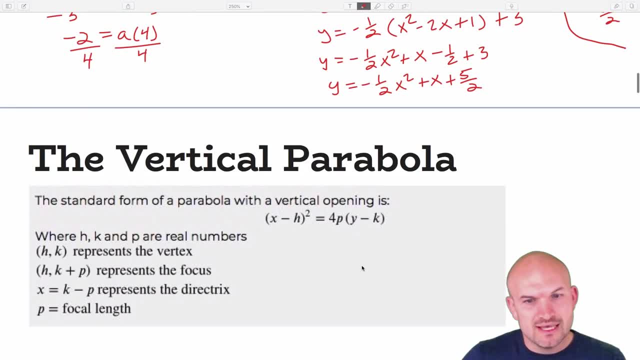 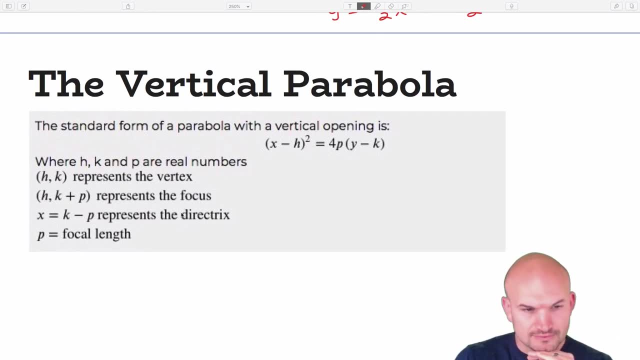 from these two equations. I'm not going to get into that for this lesson because my point that I want to go with the students is remember H and K. that's going to represent the vertex, something we are familiar with. So what P represents is our focal length. 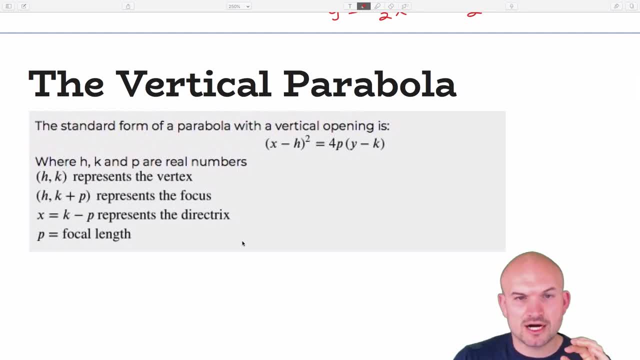 And basically the focal length is going to be the distance that our parabola or our vertex is from our focus. Now I used to do- and actually when he used to teach us in algebra two we'd actually do- to investigate this length, And it actually is a pretty nice lesson. I think it's really 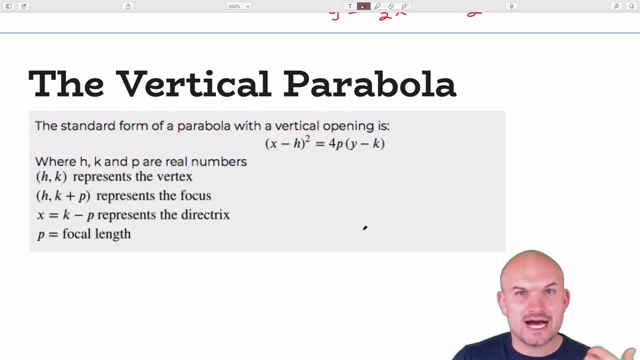 interesting for students to be able to see how that works and how to see how this value P comes together. But the general idea here is, if we have a parabola, let's just draw a parabola like this. So here's going to be your vertex, This is going to be your focus, And that distance. 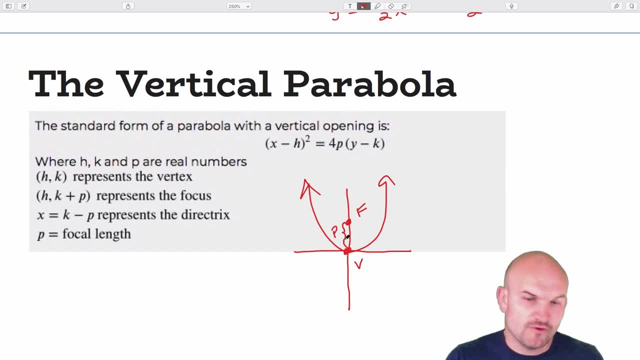 from our vertex to our focus is going to be our focal length, which in this case, is going to be P. Now, the interesting thing that happens here is we also have this line which we call the directrix. So the directrix is going to be P, but it's going to be in the opposite direction. 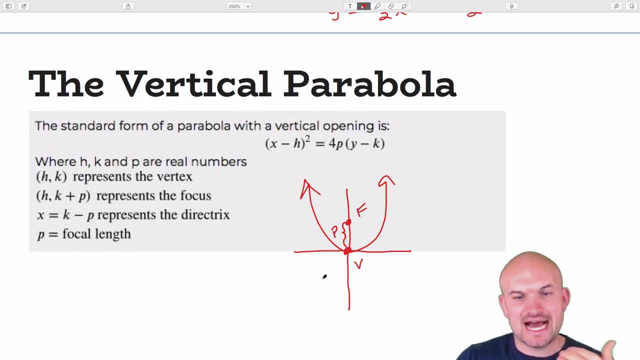 So don't think it's always negative P. Just think of this as again P in the opposite direction. Okay, So therefore we can go. P is always the distance from the vertex to the focus, which sometimes is a positive direction, Sometimes it's a negative direction. 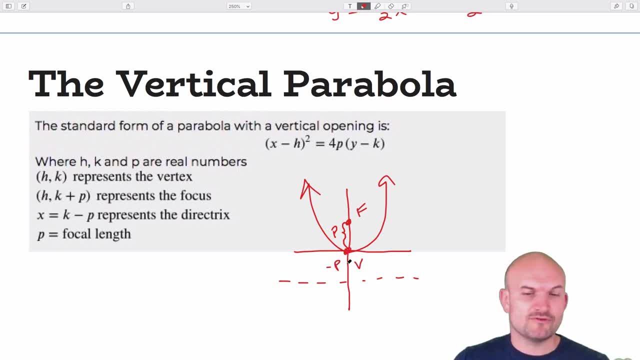 But then opposite of P is going to be from your vertex to your directrix, And actually I'll just So that's going to be my focus and that's going to be my vertex. So obviously, guys, we can have a parabola that opens up right. We are familiar with that, And that'd be when P is positive. 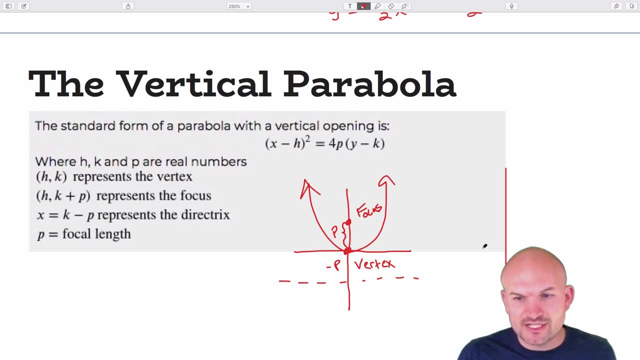 However, if P is negative, then we're going to have a parabola that's going to open down. So I'll kind of draw something like that. It's going to basically kind of take this same shape, you know, and again, we don't have to have the vertex on the origin, It can be kind of moved over. 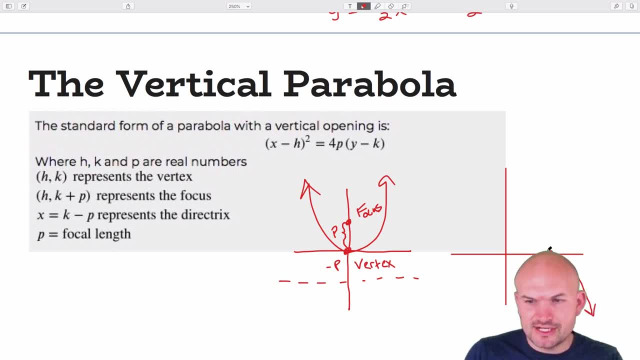 But the main important thing that I want you to kind of see here is that if you have a parabola, see here is, you know, let's say here's the vertex, now Let's say here's the focus. So now in this, 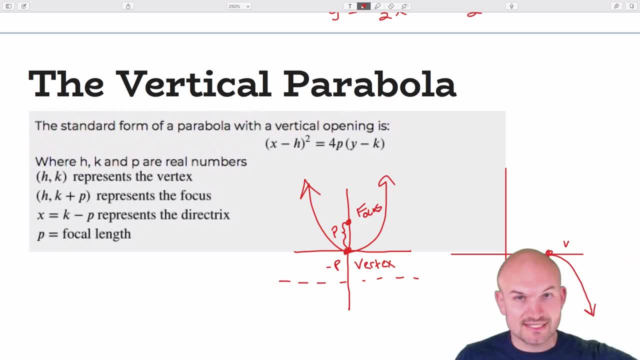 case, if we have the focus now below the vertex, what's going to be happening here is just that just P is going to be now negative, It's going to be in that negative direction, But again P is still just going to be that distance that's going to represent from the vertex. 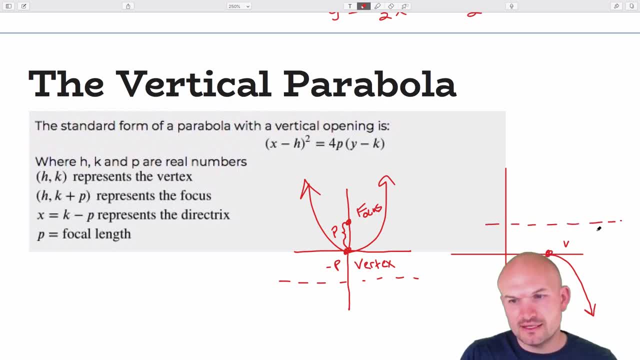 to the focus And the opposite of P is going to be going to your directrix, So I don't want to write. you know, in this case you can see that P is going to be, I guess. I guess we can just write it. 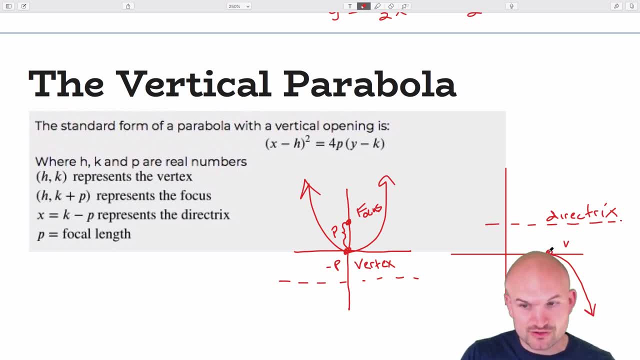 in there. From this case it's going to be a negative P, or at least it's in that opposite direction, And then from there to there is going to be P. Now let me actually just go ahead and fix that, because it really is still going to be P Actually. I'll just kind of write: 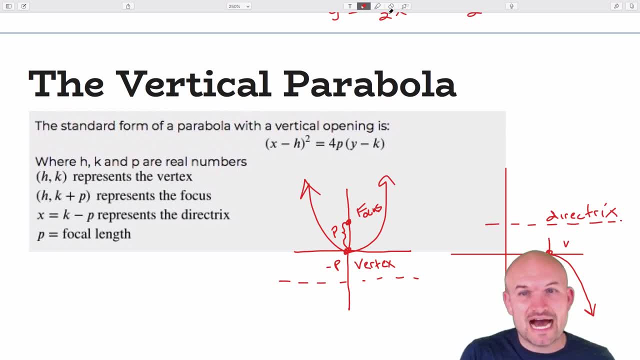 that distance is still P. It's just going to now be P in the opposite direction And this is going to be a opposite of P. So opposite of P. Okay. Now, again, P could be positive or negative, which we'll kind of talk about in a little bit, But again P is going to. 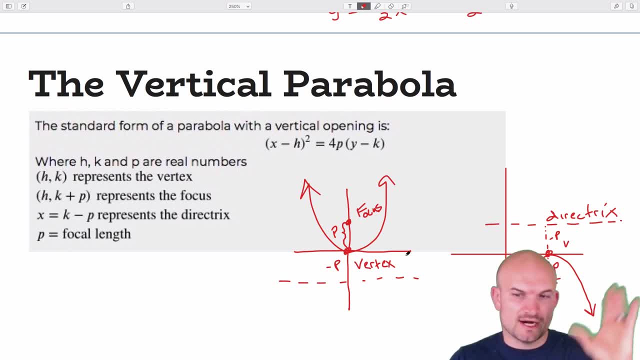 the main important thing I just want you to see is where it's going up or down, And actually you know what Let's look at. let's just change that up. I know I'm kind of starting to get a little confusing here, But now in this case we can say P is going to be negative and that's going. 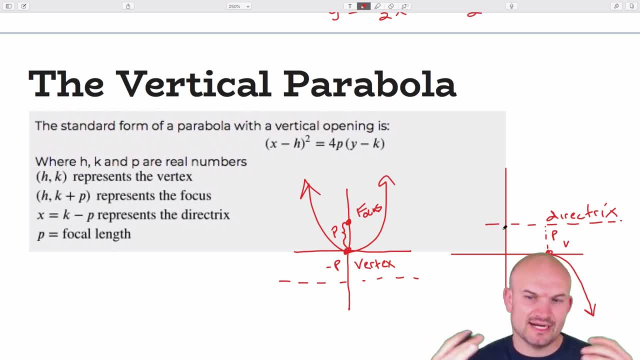 to be a positive P in that way. But again, the difference here is you can see that we have a parabola that's either going to open up or open down. The other thing I just want you to kind of recognize here is that the directrix is a line. 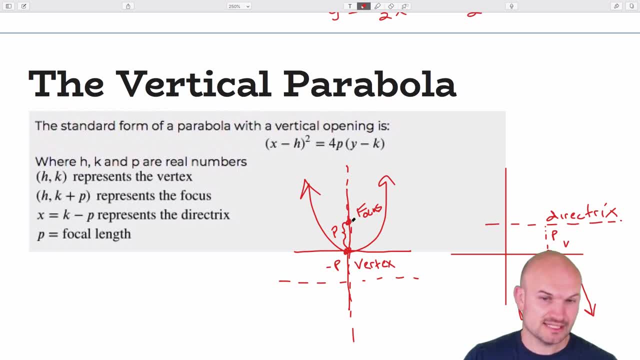 Okay, It's the same distance away from the vertex as the focus is. And then also that it's perpendicular to the line of symmetry or the axis of symmetry, right? So if I have my axis symmetry, you can see my directrix is going to be perpendicular. Now, one of the things I am 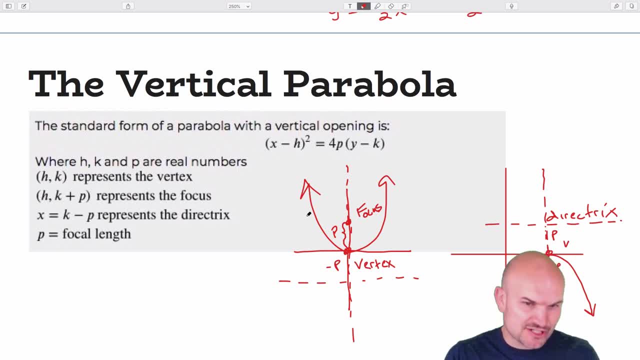 going to kind of skip over. for those of you as far as like the definition of a parabola, as far as like the set of points that the equal distance, that is one thing I kind of like bring up to students. That's the cool thing about the parabola, If you kind of look at this directrix. 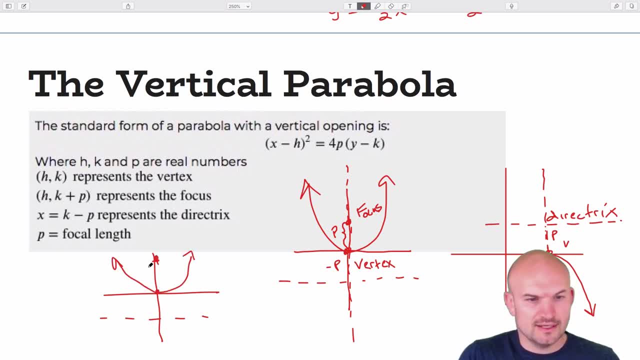 and you kind of do something that the distance here between your focus and your directrix to any point is always going to be equal. So that's kind of like where we come up with that definition of the parabola. But again a little sidebar, we're not going to get into it, or at least kind of. 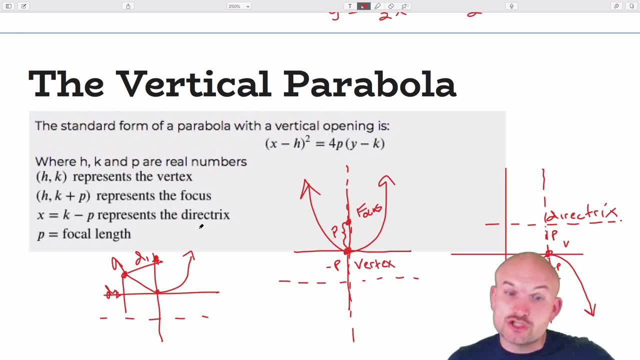 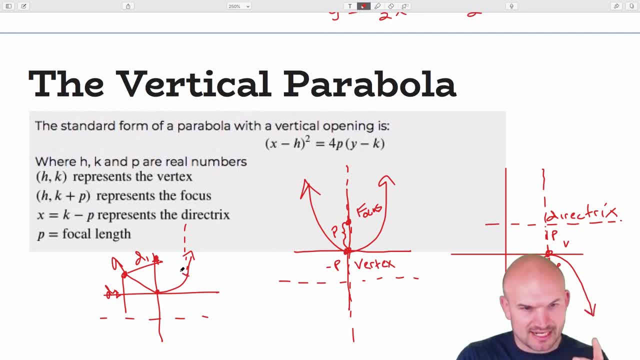 you know bifocals, you know every single time when you have something in, that's always going to direct back into the that focus. So there's a lot of applications with this as far as the focus and this parabola. But in this lesson 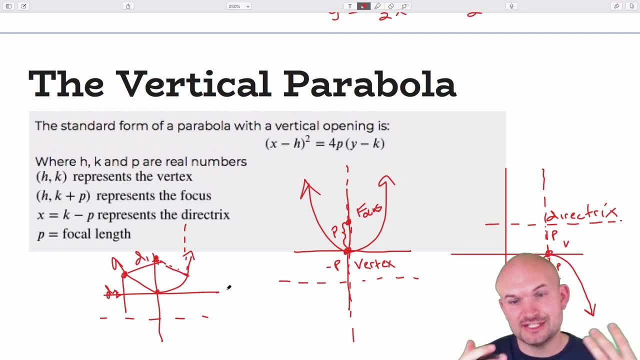 we're just going to kind of focus on identifying these certain parts. But obviously if I was in the classroom I would spend a little bit more time kind of talking and like showing students how this kind of works for different. you know shapes of parabolas, you know for like. 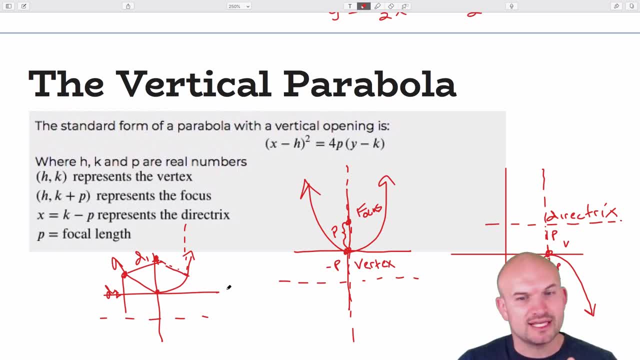 eyeglass wear or satellite dishes and all that kind of stuff, Seeing why that focus, how that is in that importance. from there, you know, flashlights or like lights, seeing how everything rays out. So it's, you know, definitely some pretty interesting stuff. 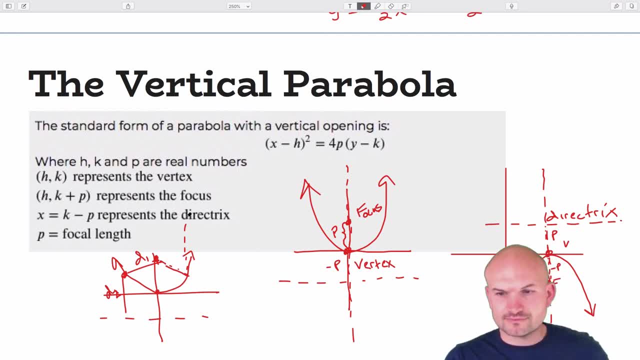 and also some applications. The one thing I want you to see is, when we have a vertical parabola, that my focus now is going to be up and down, right, So we find the vertex and then you're adding P to be your focus. Now, again, P could be negative or positive. right, If P is positive? 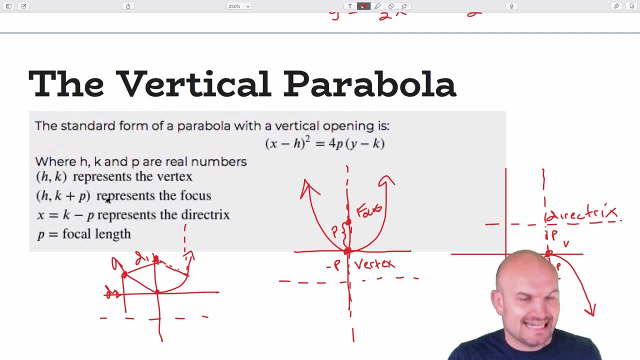 it's going up. If P is negative, though, it's going to go down, but you're just adding it Now if, to find the directrix, you're just going to subtract P. So again, it doesn't matter if P. 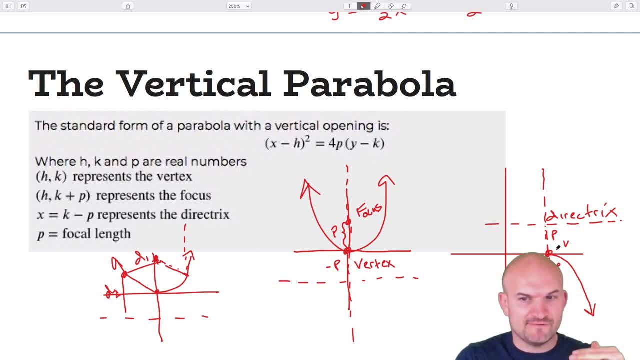 is positive or negative, because if you subtract a positive that's going down, But if you subtract a negative that's actually going to be moving it up. Okay, And then P is going to represent the focal length. Now the important thing here is we need to recognize we can have parabolas that are 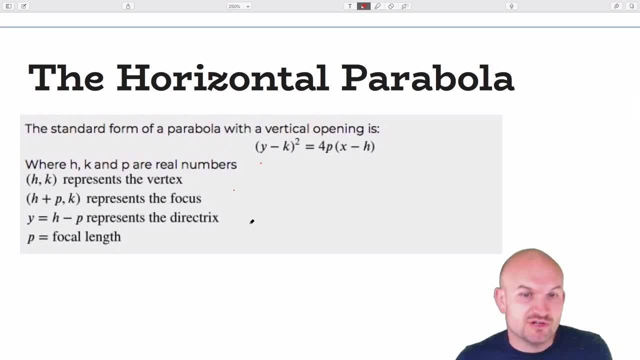 We're used to those right, But we can also have a parabola that is going to be horizontal. So if X was squared, we knew that was a vertical parabola. But now if Y is going to be squared, that means 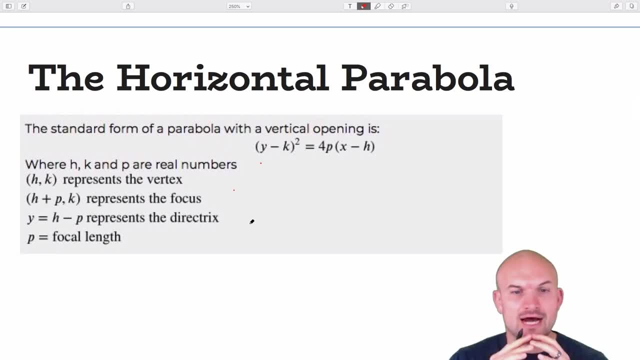 our parabola is going to open up to the left or to the right. Now, just like, if a parabola opens up, that means P is positive, Well, if it opens up to the right, that means P is going to be positive. 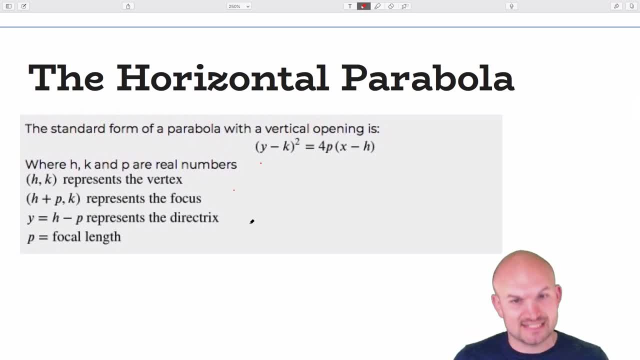 For a vertical parabola. if P was negative, that means it opens down. Well, if P is negative for a horizontal parabola, it's going to open up to the left. So, if P is negative for a horizontal parabola, it's going to be positive. Well, if P is positive for a horizontal parabola, it's going to. 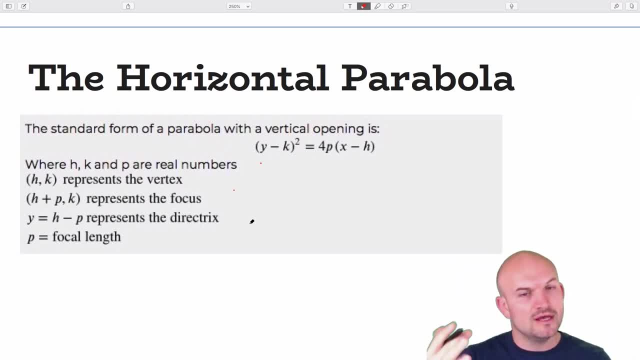 kind of think of like the X- Y axis. you know, up is positive, down is negative. Well, same thing. Y is positive, I'm sorry, going to the right is positive, Going to the left is going to be negative, But the same idea. you can see, really there's really no difference. 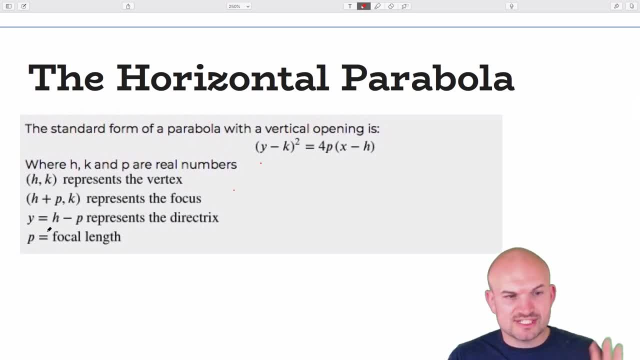 in the equations that we're using. We're still. P is still representing the focal length, It's still the distance from my vertex to my focus, And then we're going to subtract that value of P to go to the directrix. The only difference is again, now we're dealing with 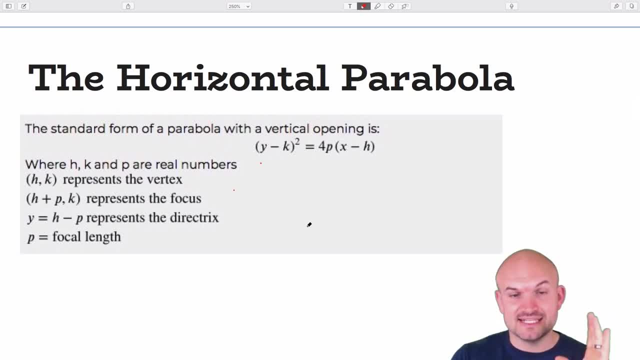 parabolas that have horizontal openings instead of vertical openings. So let's go and take a look at what that would look like in terms of a parabola here. So that's going to be kind of going. So if I'm going to have this parabola, let's here open up to the right. All right, Now again. 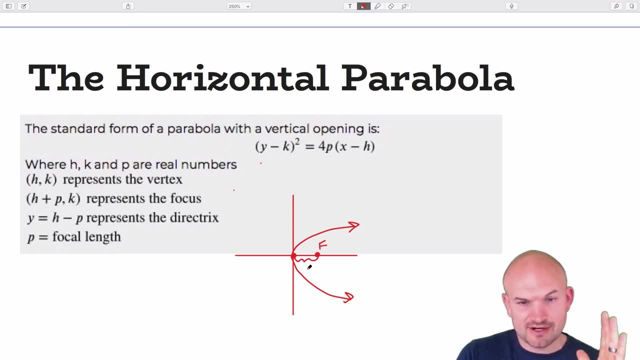 my focus here is going to be to the right, And again, this distance here is going to be P, whereas the opposite distance here is going to take me to my directrix. Now again, remember the directrix, one thing I kind of forgot to mention here. notice that the directrix. 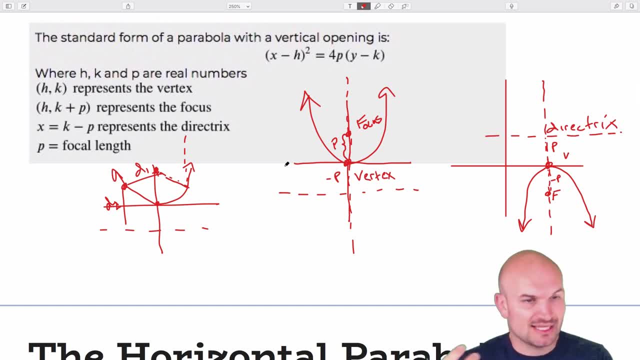 is not a point. That is one of the misconceptions a lot of students will make. They'll treat the focus as a point, the vertex as a point, but the directrix is not a point. The directrix is a horizontal line, And if something is a horizontal line, then it needs to be in the form of Y equals. 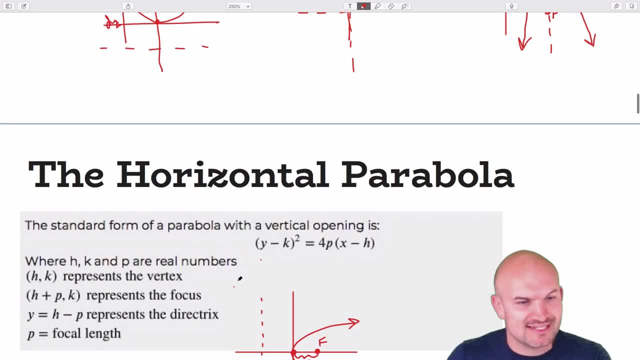 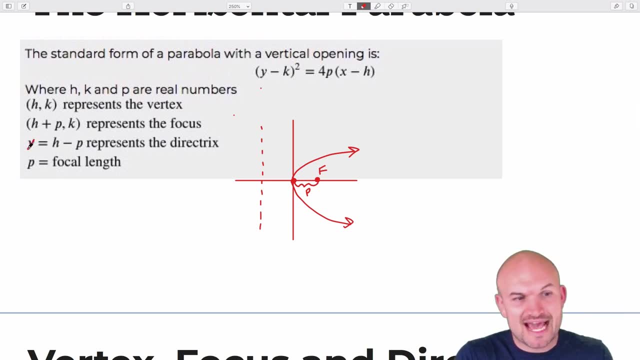 not X equals. So that was my mistake right there. I do apologize for that. I'll have to go ahead and change my notes In the same respect. over here you can see that this needs to be a vertical line, So this needs to be X equals. So I didn't kind of cover that or check myself on. 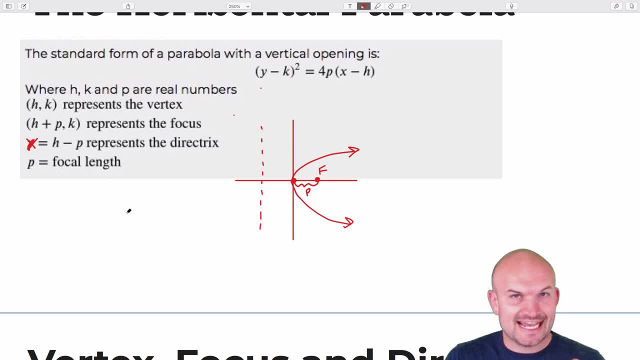 that. But you can see that X is going to equal H minus P. but that is a vertical line, It's not a coordinate point. So it's a very big distinction that we need to make sure that we are doing here. So now we're going to have P And then again that's going to be our negative P, That's our. 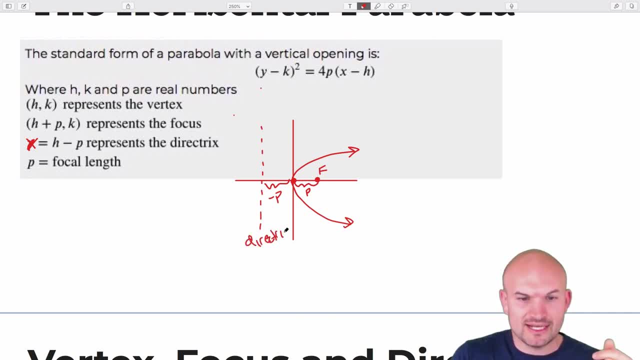 focus, And this is going to be our directrix. Now, in addition to that, we have our vertex right there. We could also do another parabola, Where it's going to have a opening now to the left, And that's going to look the exact same. 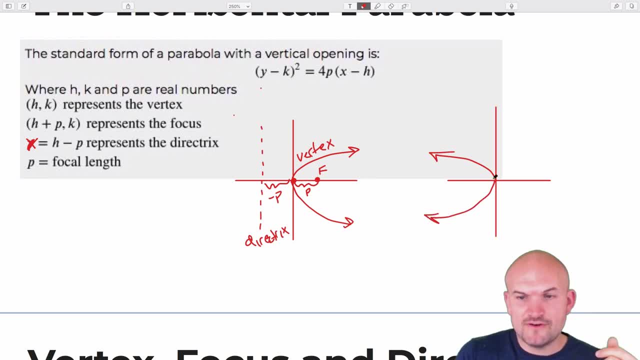 It's just that now the distance from my vertex to my focus is going to be negative P. So let's go and put our focus here, Let's put this to be our vertex. So we'll just say that's going to be negative P, That's going to be my vertex, And then P is now in the positive direction, is going to. 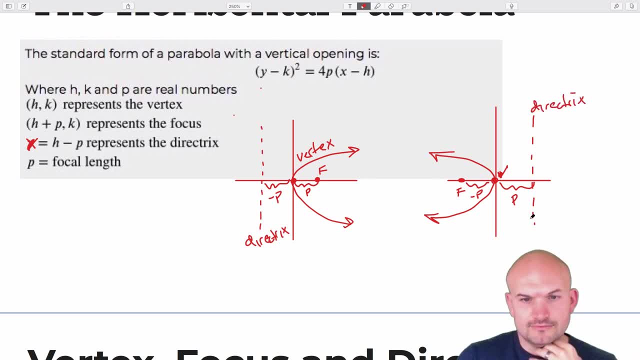 take me to my directrix. Okay, So that's going to be dealing with. we have a horizontal line, We have a horizontal parabola And again, really, the main difference is, you know, recognize what we're doing with the focus, to go from the vertex to the focus. You can see we're adding P to the 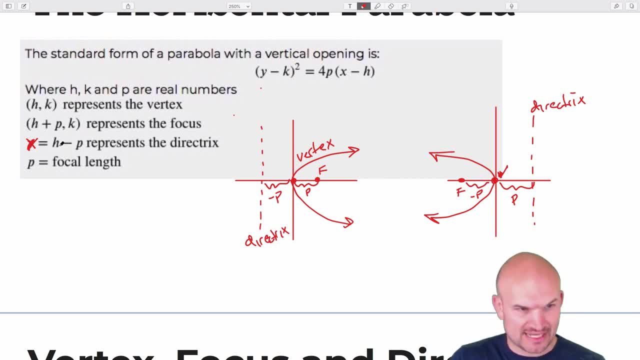 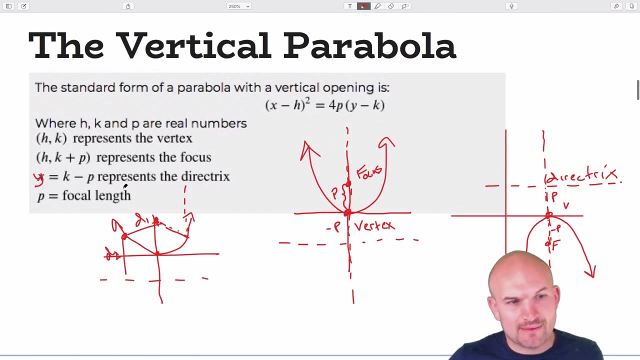 X coordinates right And to find the directrix we're subtracting P to the X coordinate H of the vertex. But just make sure you understand my correction here that the directrix is a vertical line. So therefore it's going to be X equals And for the vertical parabola it's going to be a. 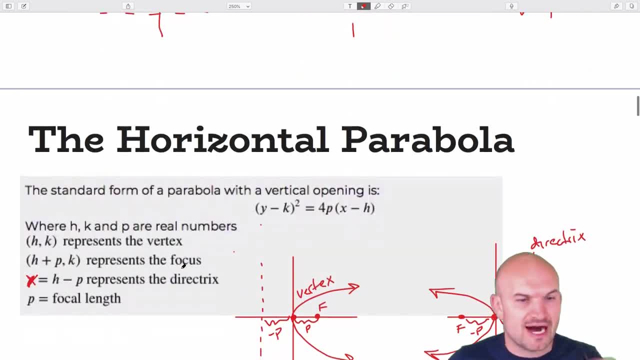 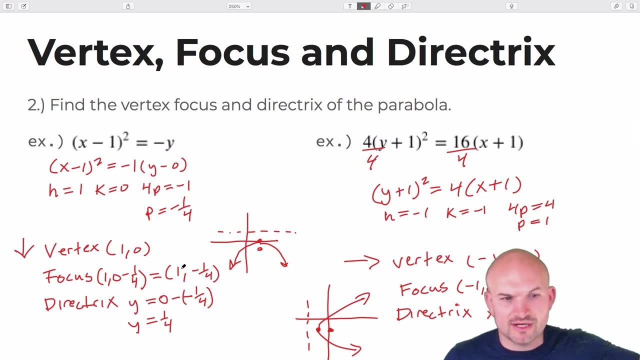 horizontal line, So it needs to be Y equals. So make sure you have on those corrections. So now let's get into the examples that I kind of covered into the class. So this is what I would have covered exactly for my students was just a simple like: all right, here's, you know, an equation: find the vertex, the focus. 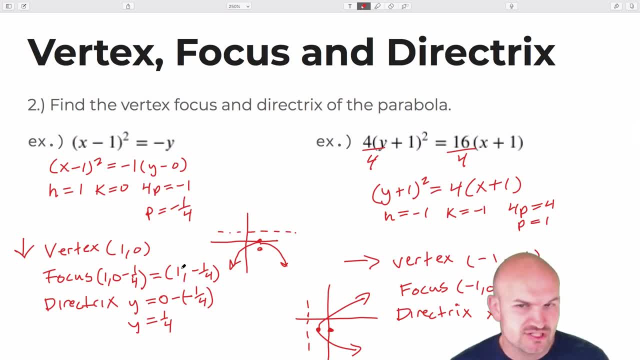 and the directrix of a parabola. Now, typically, when we're first kind of doing this, I have students just write it out. you know, for all your values, use your parentheses, put it exactly into the form that you're familiar with. So you don't technically need to do this, but it is one of 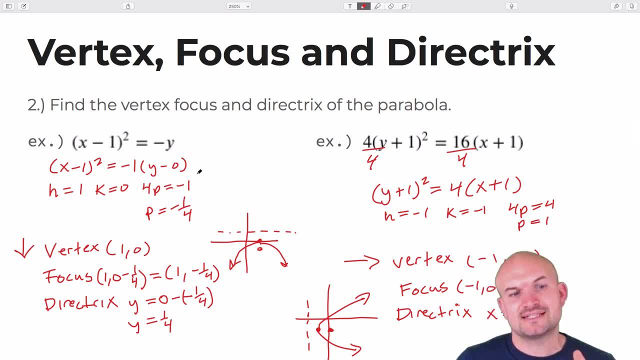 those things. I just like to show students my work and my thinking process, So therefore they can kind of see how I'm getting my answers. So in this case I have X minus one quantity squared equals negative Y, And all I did is I. 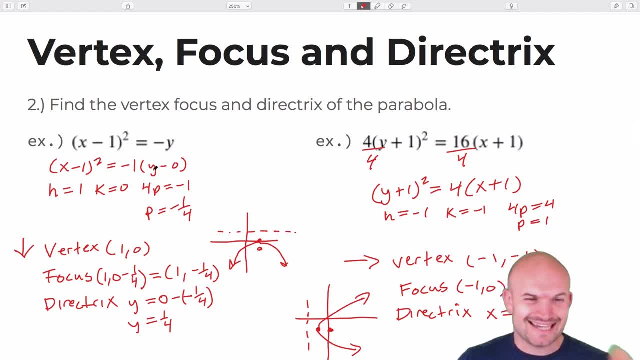 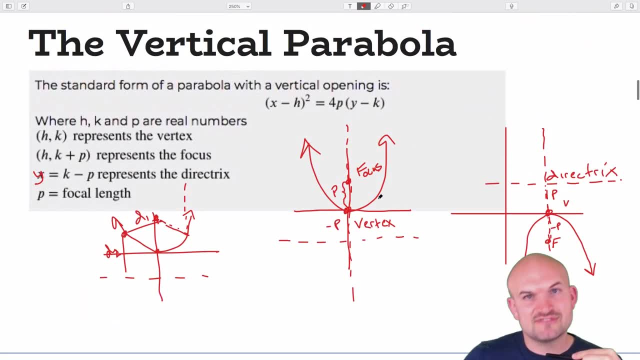 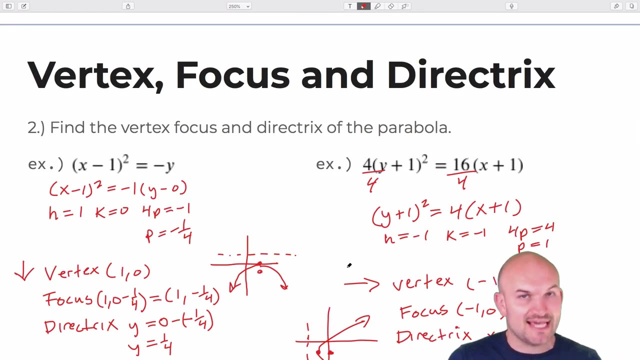 just rewrote this left right-hand side as negative one times Y minus zero. So it's just a little bit cleaner approach for me to be able to kind of see it now in this format And again to really all I need to identify my vertex, my focus and my directrix. I need to know my H and my K as well. 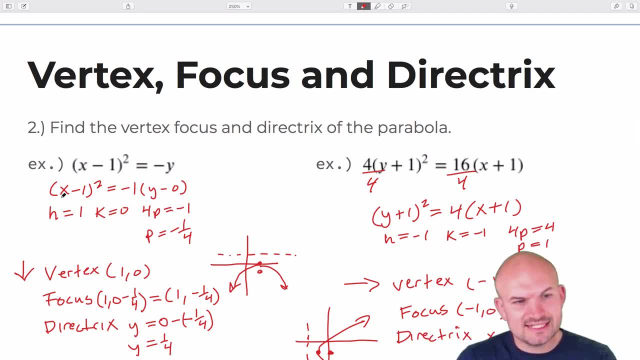 as my P. okay, So in this case, I can see my H is one, my K is going to be zero and then my P is going to be well, four. P is equal to negative one, So therefore, P equals a negative one-fourth. 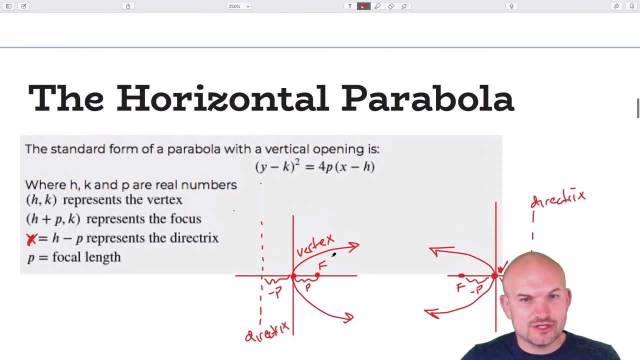 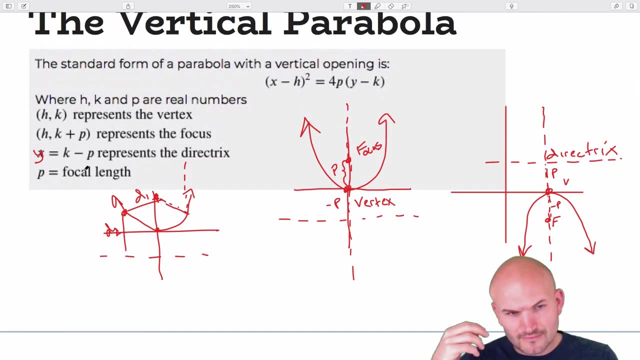 Now one of the misconceptions a lot of students will do is they'll want to go ahead and use these formulas. right, And you can definitely use the formulas. I just think your students a lot of times they kind of forget, you know, my adding, subtracting and like which variable. 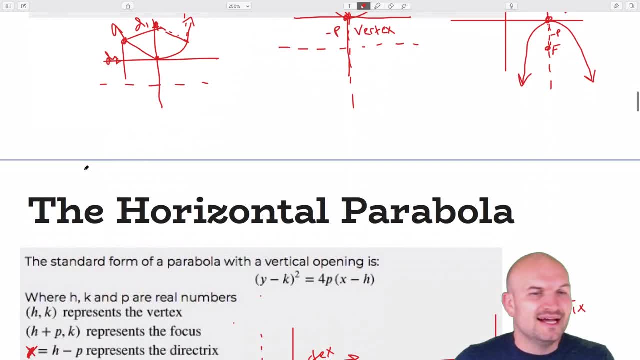 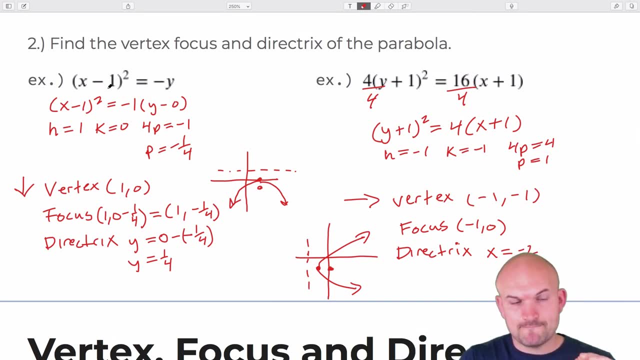 adding to the positive, my adding to the negative, like to the Y or the Y, And they just get confused and they get it mixed up. So what I recommend the students to do is: you know, you see, that the X is squared, So therefore, you know it's going to be opening up left or right, right, So what I'm 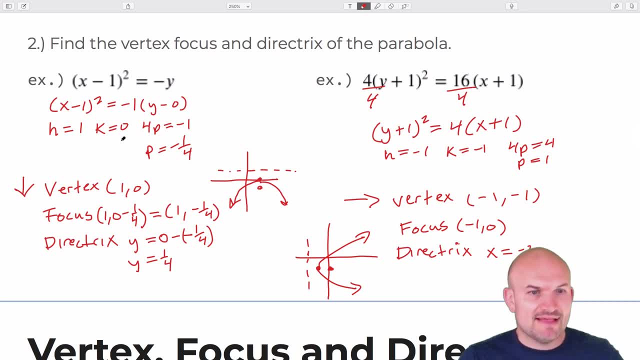 going to do is I'm going to plot the vertex And then. so once I plot the vertex, then I'm going to say, all right, P is negative. So that means remember, if you think of P as that distance from 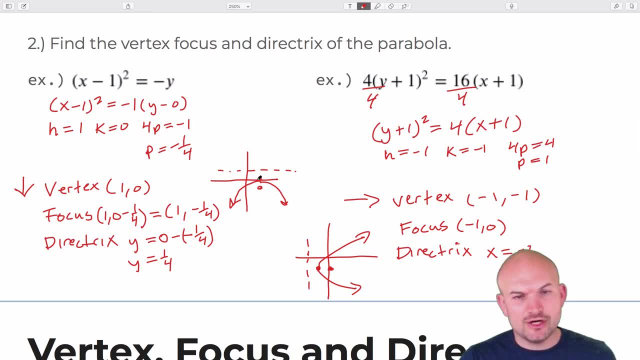 the vertex to the focus, that means I have to go down negative one And notice that the parabola opens up towards the focus right And again. the directrix is going to be perpendicular to that axis of symmetry. So if I have my vertex is one zero, then if I have the focus is down, negative. 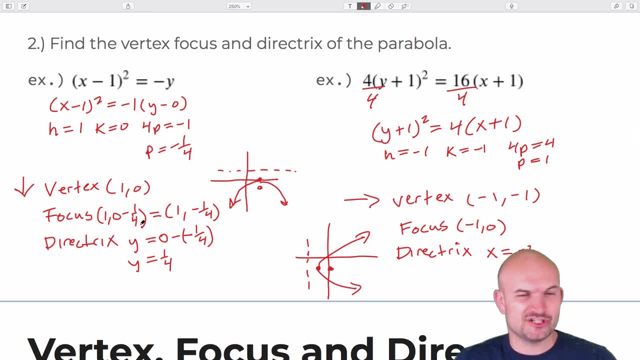 one fourth. yeah, you could do zero minus one fourth, but you don't really need to show the work. Hopefully you just recognize it's still going to be over one, but it's just going to be down negative one fourth. And then remember the directrix is going to be minus P. Well, since P, 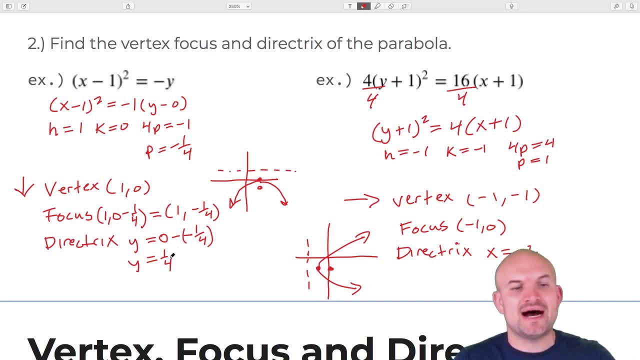 is negative, you're subtracting a negative P, So that's actually going to give us a positive one fourth And you can see that Y equals one fourth. You can see how that's going to create that equation of the line. So I typically like to just look at this graphically, but I do understand that. 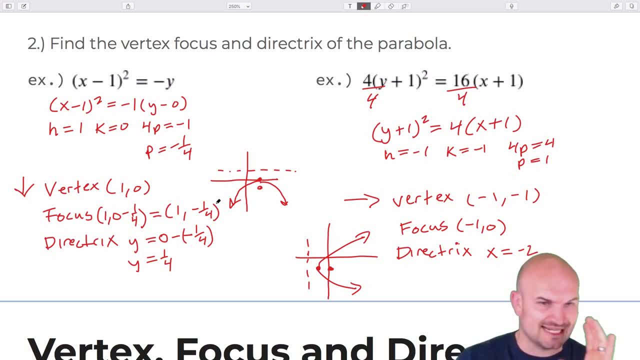 some students just like to remember the kind of rules like adding, subtracting to which coordinates. I just think it's very easy to get those kind of confused if you're not looking at where these values are. Now in this next example, this one's kind of confusing because 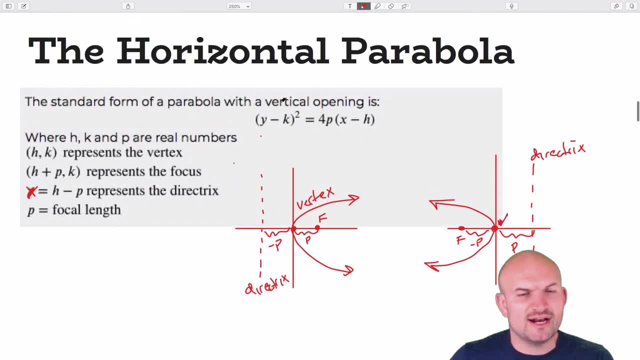 in all of our standard forms, whatever quadratic we have. we don't actually know what we're going to do with this. So what we're going to do is we're going to divide it by P in both sides. Now, in the last example, we were going to have the formula. 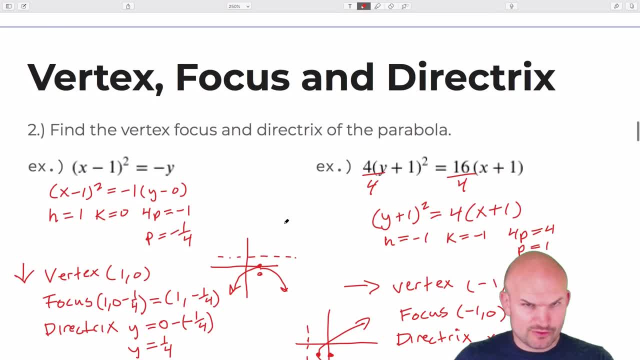 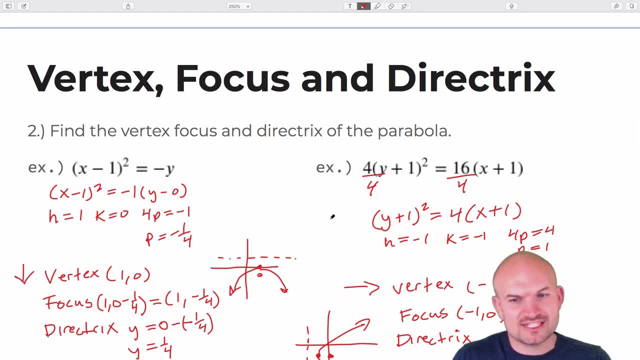 that's what we had here. This binomial squared did not have any coefficients in front of it. Right, There was no coefficients in front of there. So what are we? so? what should we do? Well, we should get rid of that coefficient. So what I'm going to do, the first step is divide by four on. 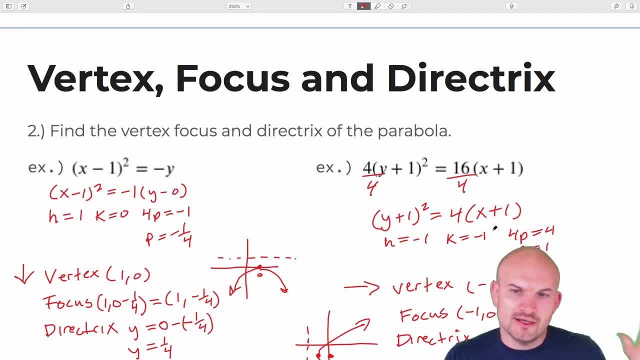 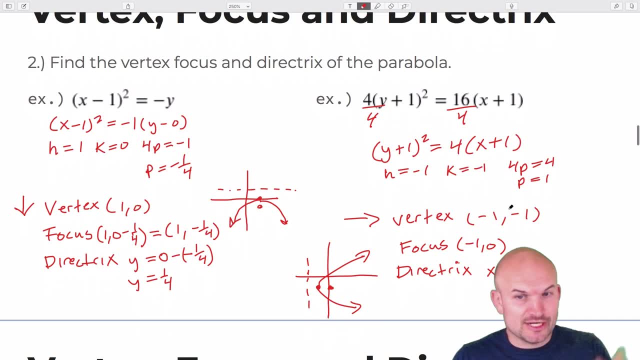 both sides. Now I have it in this more form that I'm a little bit more familiar with. Now I can identify: my H is negative one, My K is negative one and my four P is equal to four. Therefore, divide by four on both sides I can see P is equal to one. 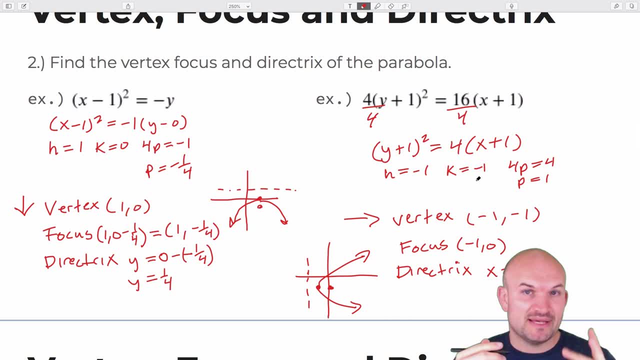 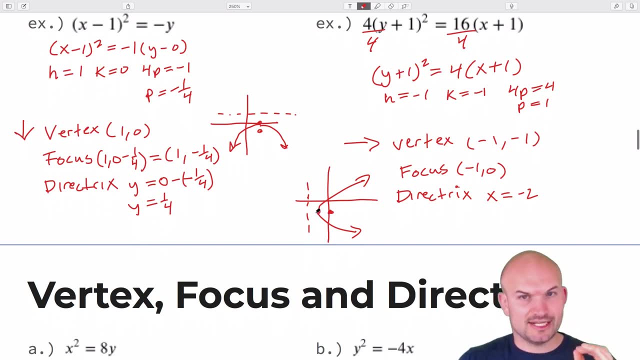 know it's going to be opening left or right, And since my P is positive, I know my focus is going to be going to the right. So, therefore, if you kind of look at this equation, you can say: all right, here's the vertex. My focus, though, is going to be to the right of that right, And so, if I 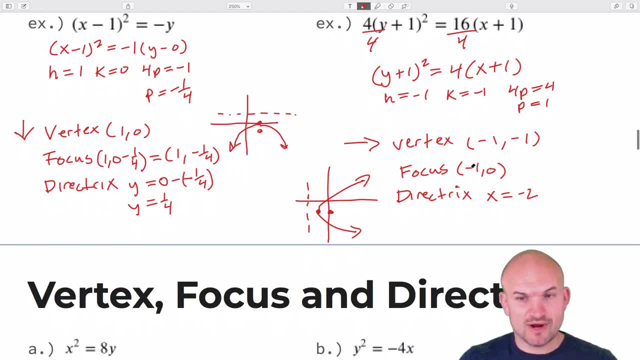 take this vertex which is: at what negative one? zero, and I move that to the right. that's going to give me a new point of that's wrong. negative one, negative one. That's going to give me a new. 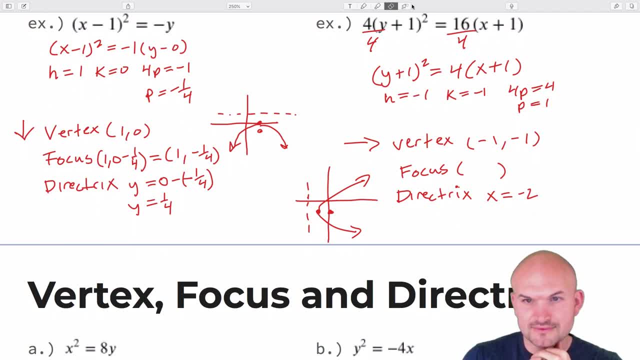 point of: actually- and I can see this, I switch those around to- the right is going to be zero comma, negative one right Because- and again, you can look at that like I graphed it correctly- I just wrote down the answer incorrectly, So that's why I like looking at this graphical approach. 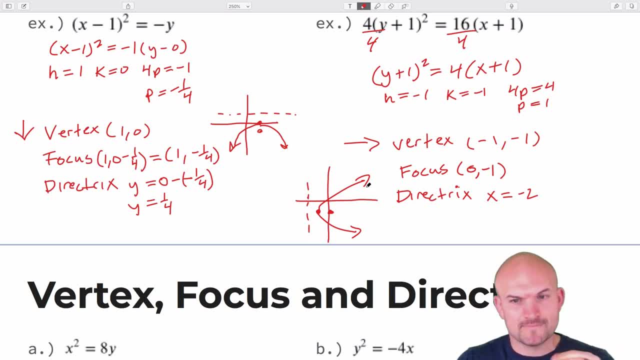 because I was able to quickly audit my answer and say, oops, I did something wrong. But again, like, here's the point, If you're going to move this one unit to the right, you're going to add a one to the X quarter, right, You don't add a one to the Y coordinate. That doesn't make any sense. 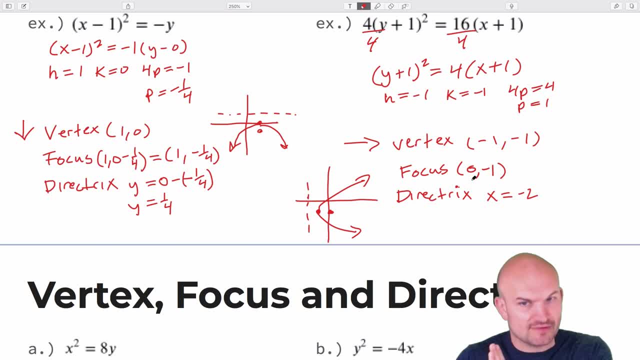 Adding a one to the Y coordinate is going to shift it up. We're trying to go to the right of the vertex And then remember to find the directrix. we're going to take our X coordinate and we're going to subtract one. So therefore, you can see, that's why that's at. 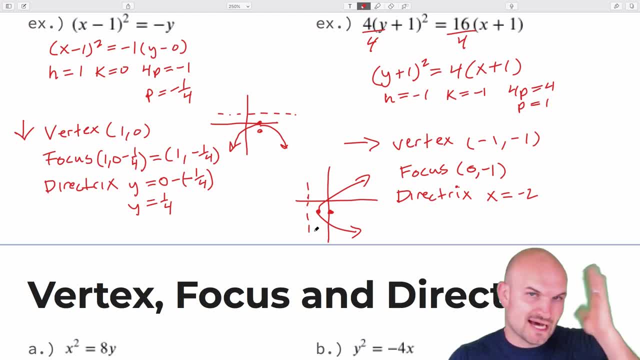 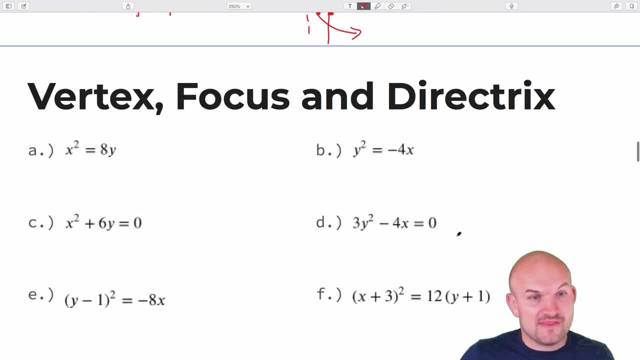 negative two, but remember it's a line and a vertical lines is going to be in the form of X equals negative two. All right, So that was all the problems that we have, And then, typically, what I would have done in the classroom is I would have said: all right, guys, now it's your turn. 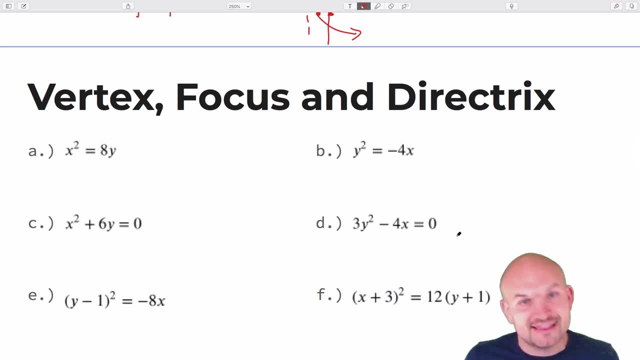 to go ahead and to do these problems And my students at this point would be going up to the board and or working with them in their groups and then go ahead and presenting their answers. Now, since I kind of spent some time, at least in depth, going through these answers, 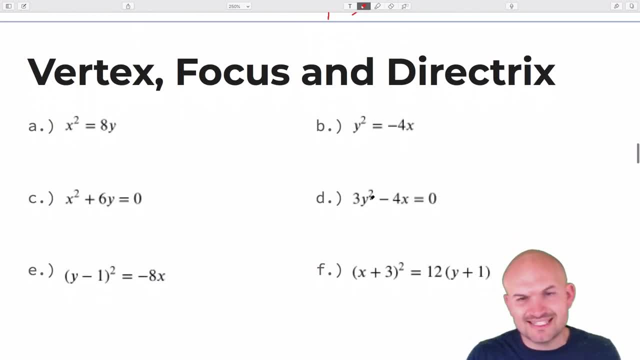 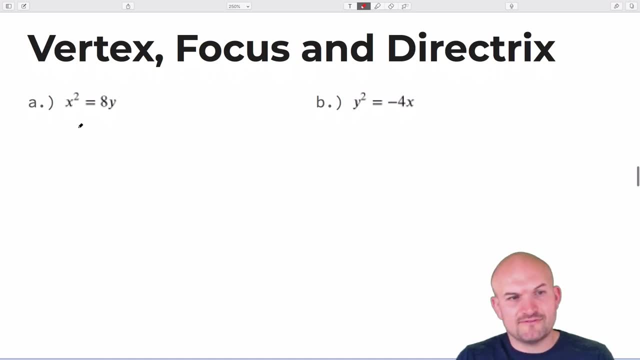 I'm just going to kind of work through these a little bit quicker and just at least not go through, as you know, as much in depth as far as my explanations here. So, but I would just say the first thing, guys, is just to identify the vertex, So in this case, the vertex or the H. 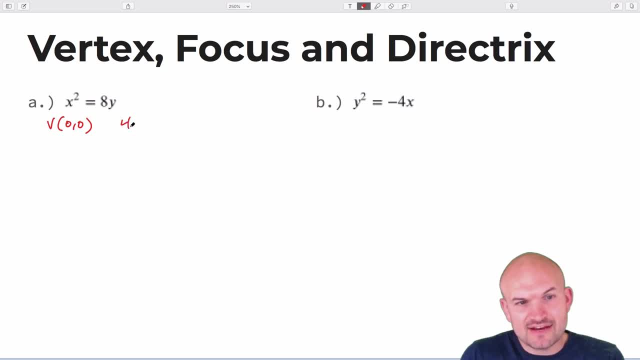 and the K right is going to be zero, comma zero. And then we can say that four P is equal to eight right, Cause that's the coefficient of the Y. So I'll divide by four on both sides and I can say P is equal to two. Now again, 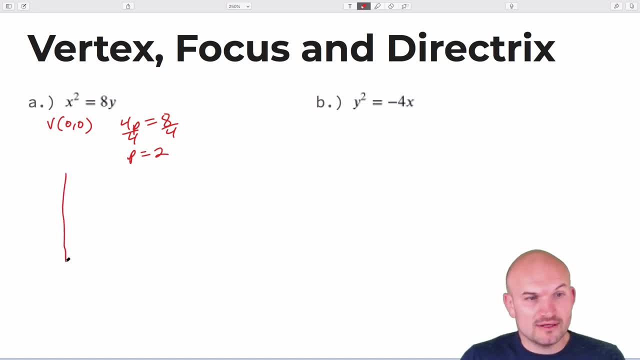 I recognize this to be an X squared. So therefore, if I have my vertex here, right, So I'll just plot the vertex at zero zero. I see that X squared, So I know it's going to open up or down. And since 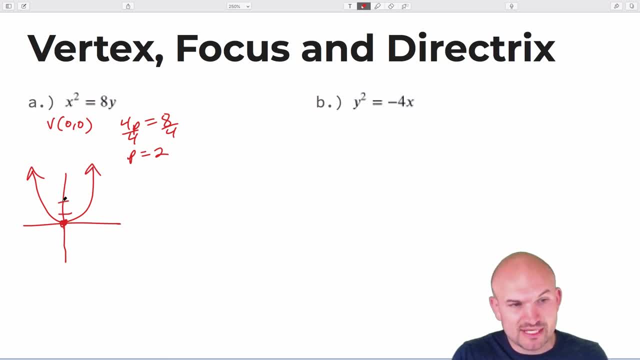 P is going to be up to or positive two. I know it's going to be going up too. So really, just from this information here, I can just go ahead and plot it and say: all right, the vertex, I'll get the information. The vertex is zero comma zero. The focus is going to be zero, two right. 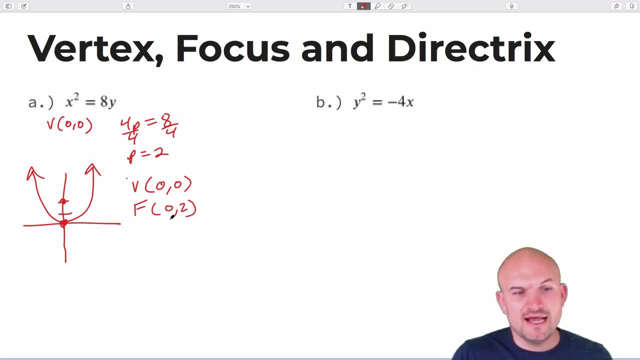 Cause I need to move up two units from my focus, from my vertex, And my directrix is going to be down two. but just remember, guys, it's a horizontal line. So we write a horizontal line as Y equals negative two. And again, you could follow the formulas if you like. I just think this is a. 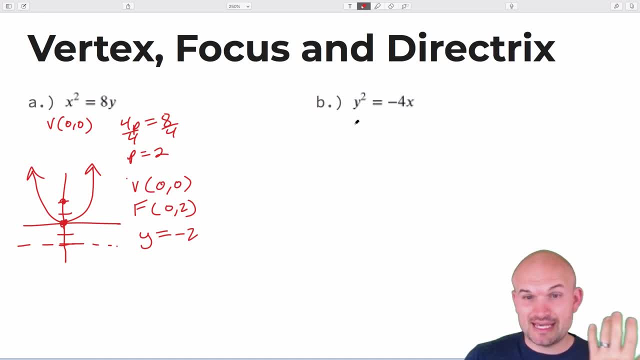 little bit easier of approach. The next one's going to be the same thing. As far as the vertex goes, we have zero comma, zero Um. in this case, though, my four P is equal to negative four, So now we're going to have a negative P. All right, And that's perfectly fine. I don't. 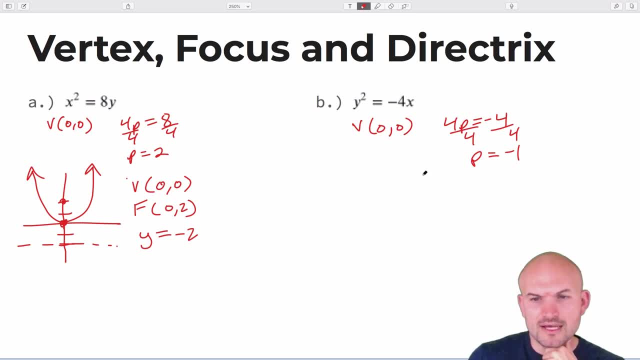 know why I'm dividing by negative four. maybe because I said it, Um. and we also know that my Y is squared in this case. So, since my Y is squared, um, that means my graph is going to open up to the right or left. Since P is negative, the next thing we need to identify is going to be our. 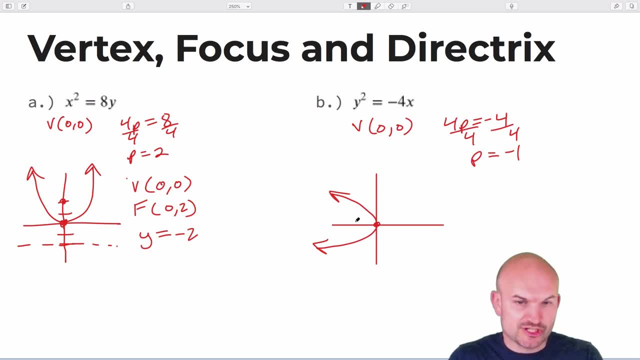 focus. So again, since P is negative, that means we're going to be moving to the left one. So our focus is going to be this way: If my vertex is at zero, comma zero, and I'm moving to the left one, that means, um, my focus is going to be negative one, Um, so focus is going to be 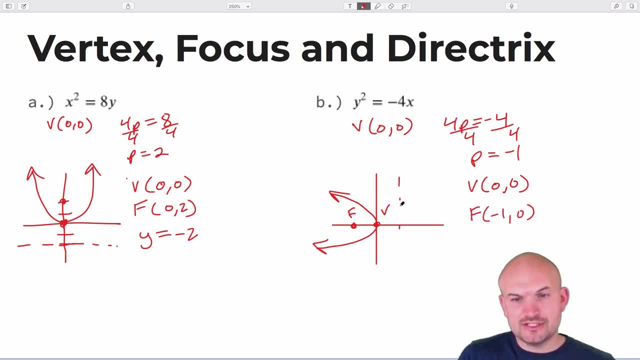 negative one comma zero, And then my directrix is going to be to the right one, And again that's a vertical line. So that's going to be: X equals positive one, And again they didn't need to sketch the graph, but I think just sketching this graph, I think, makes everything a lot more. 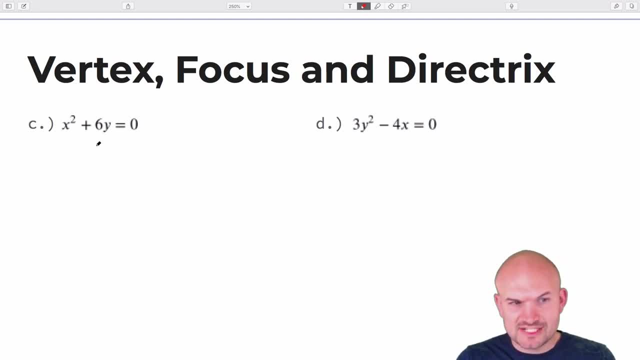 sense. So onto the next one. um, you can see that in this case we have our X and our Y are not on the same, are on the same side. We need them to be on opposite sides. So the first thing I'm. 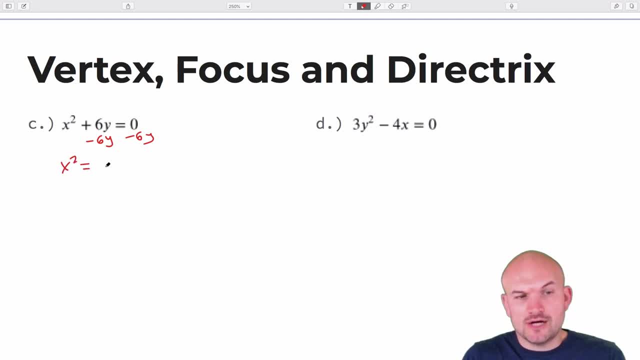 going to do is I'm going to subtract a six Y on both sides. Therefore I'll obtain an X squared equals a negative six Y. All right, Now, um, again, you can see that my vertex is again at zero comma zero. but my four P is now not as nice. Four P is going to equal a negative six. 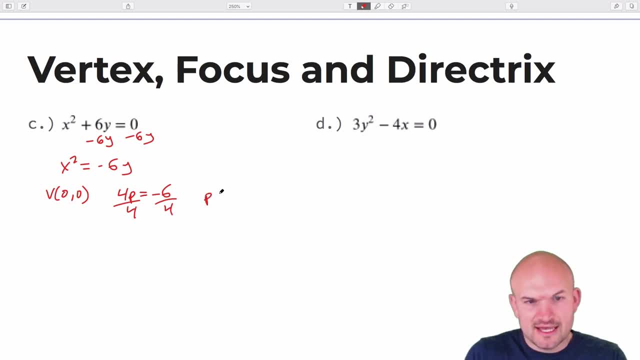 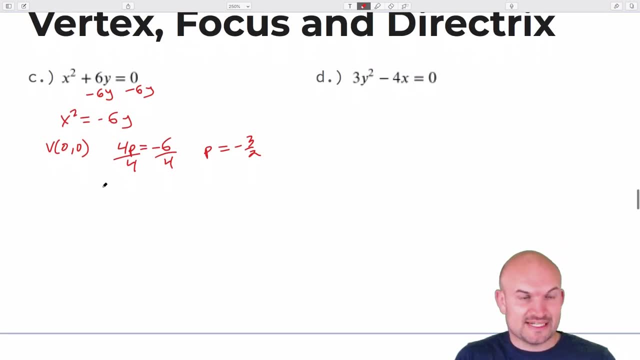 but again, I'll still follow the same process. I'll divide by four on both sides, and P is going to equal a negative three halves. All right, Um. now the next thing we're going to need to do is again, like plot this information. I recognize that my X is squared, So I know my graph opens. 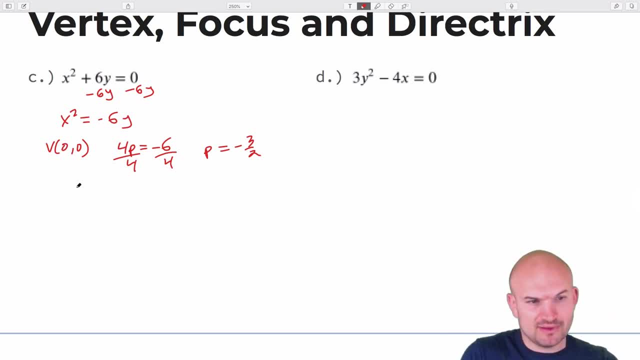 but since P is negative, I know it's going to be opening down. So I'm just going to plot this graph, All right, And I know it's going to open down. Now again, if my vertex here is at zero comma, zero right, Because I'm not adding or subtracting anything from the X or the Y, there's. 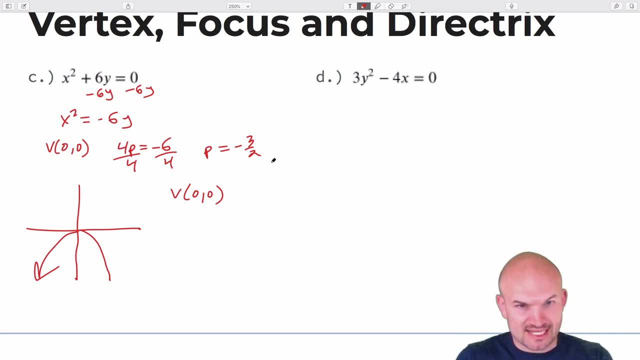 no H or K. If I need to go down from my vertex, a negative three halves- right, Because it's basically my vertex- plus a negative three halves, That's going to be the Y coordinates. So I can say my focus here is zero comma, negative three halves, And the directrix is: 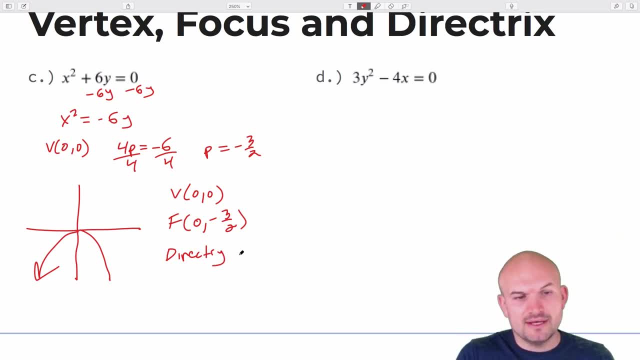 is going to be minus a negative, So that's going to be up, And again, that's a horizontal line. So that'd be: Y equals a positive three halves. All right Into the next equation. Um, again same kind of idea. We're going to want to get the X's and Y's on opposite sides. So the first. 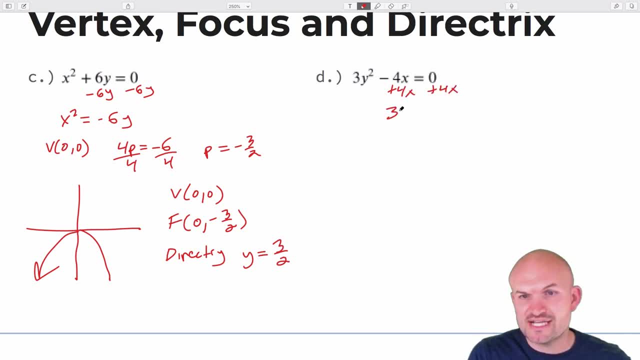 thing I'm going to do is a add a four X to both sides. Then I have a three Y squared equals a four X Um. however, remember that we do not have anything with coefficients for the quadratic um expression, So I'm going to divide by a three on both sides. That'll give me a Y squared equals. 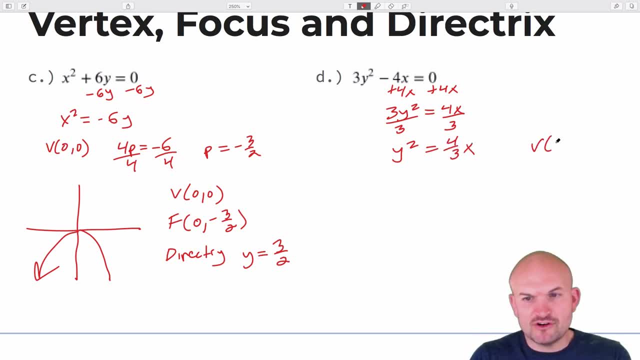 a four thirds X. So again, nice thing is, we know our vertex is again at zero, zero. We know that. we see that Y squared. So we know my parabola opens up to the left or to the right. but since my P is going to be positive, I know it's going to open up to the right. 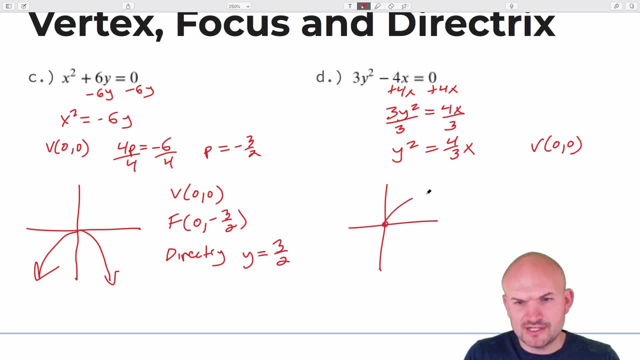 All right. So again, I just like to kind of do a quick little sketch here. All right, So it's going to open up to the right. Well, how far is it going to open up to the right? So, four P in this case is equal to four thirds. So I'm going to divide by four, but remember: 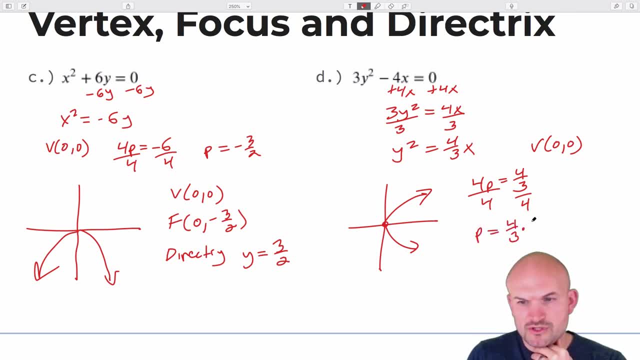 dividing by four is the same thing as multiplying by the reciprocal, which would be one fourth. So therefore, you can see my P is going to be one third. So if I'm going to add one third and I'm going to go to the right, my new focus here is going to be at one third, comma zero. 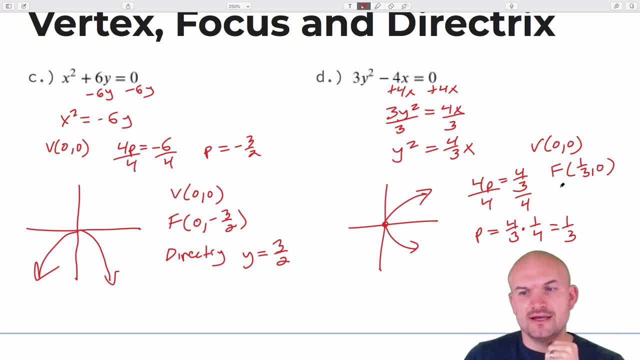 right, Because I'm going to need to add one third to the X coordinate, And then my directrix then is going to be a vertical line one third to the left of my vertex. So that would be, X equals a negative one third. 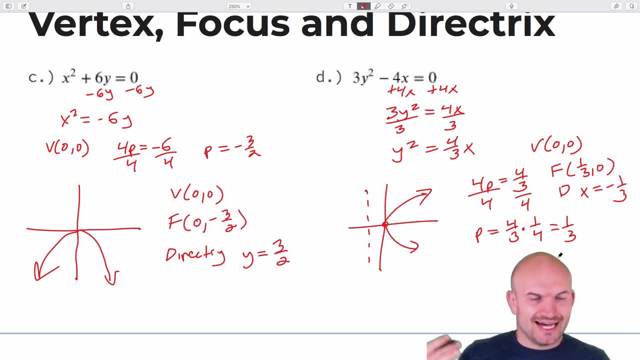 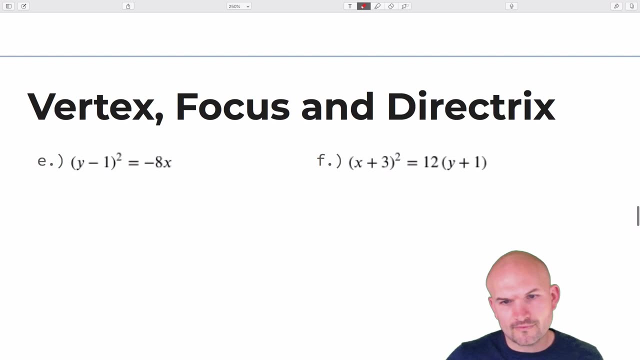 So hopefully you can kind of see, even though these have some fractions again- just understanding the orientation of the parabola and you can easily kind of just work your way through adding and subtracting and to identify the focus and the directrix. All right, So now. 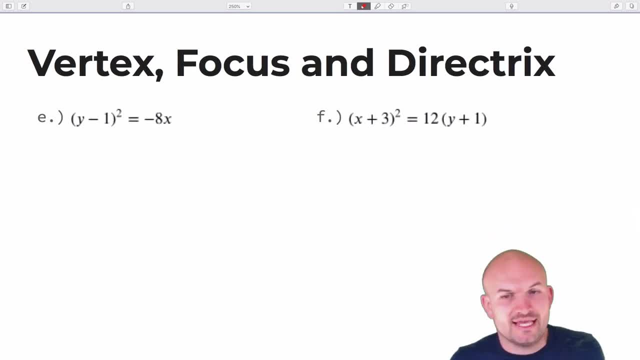 we're going to work on just a couple more problems where we do not have a, where the vertex is not going to be at the origin. So you can see here now I am adding and subtracting to my X and my Y. Okay, 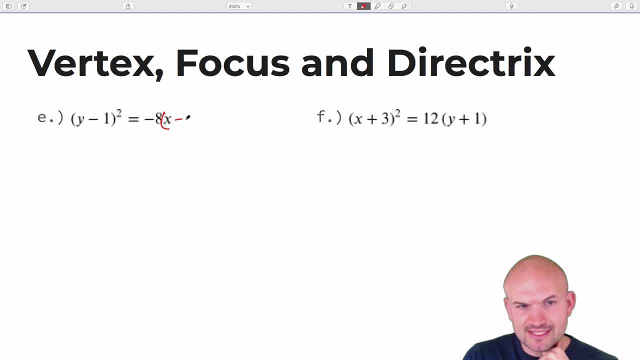 Again. for this case, kind of like the problem I did, we could easily just kind of rewrite this as X minus zero. You don't need to, but you know, sometimes it's just helpful for students to see that Now one of the main issues that students have, or one of the problems. 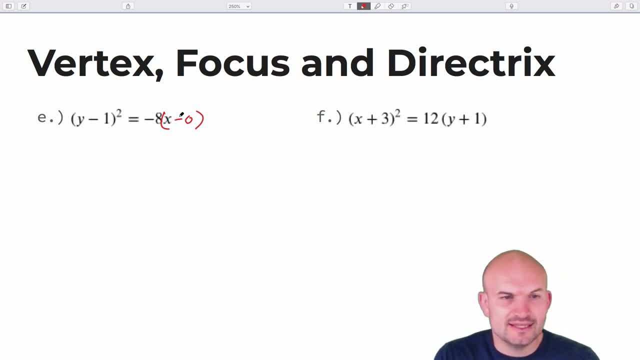 that a lot of them will do is they'll confuse the H and the K. Remember H is always with X, K is always with Y. So in this case my vertex is going to be zero comma one. Make sure you remember that. And again I'm going to plot that. So zero one is going to be up. 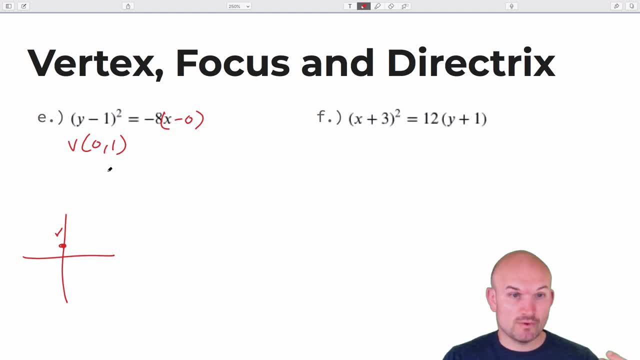 one, and that'll be my vertex. Now I see my Y is squared, So therefore my parabola's is going to open up to the left or to the right, And I see my P, whatever it is, it's going to be negative. So therefore, 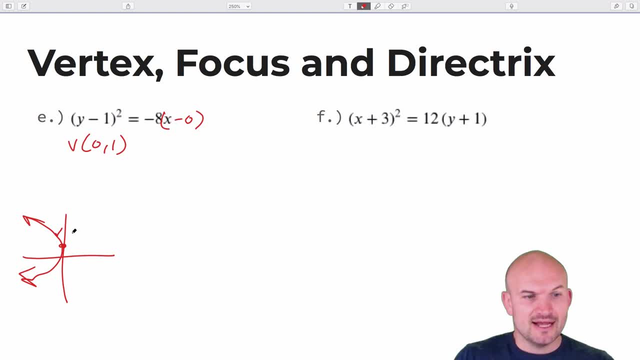 I know my parabola is going to open up to the left. Okay, And that's going to be very important because I don't like following those formulas I gave in the notes. I like to just visualize based on this information. I know my parabola has a vertex of zero, one rather. 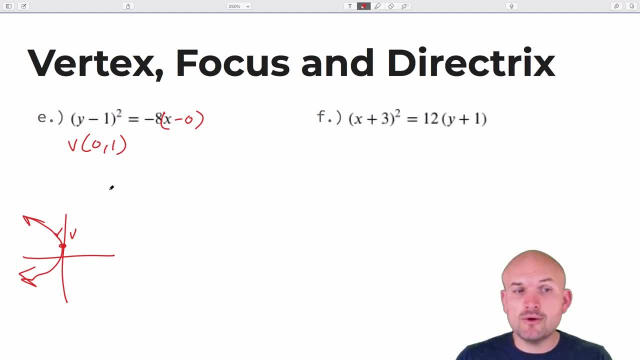 simple and it's going to open up to the left. Now what I need to do is identify my P. So I have my: 4P is equal to negative 8, divide by 4 on both sides, P is equal to negative 2. You. 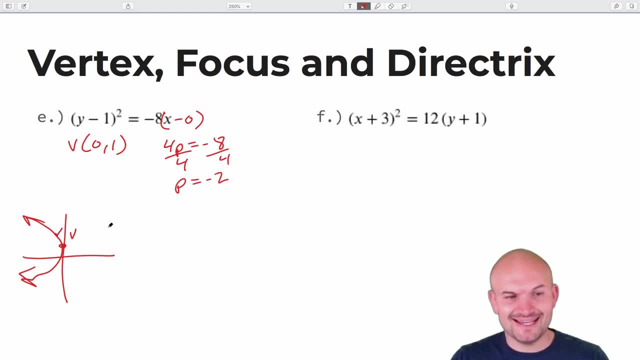 could probably have done that in your head, but it's okay. So if I have my vertex at 0,, 1, and I'm moving it to the left- 2,- I can now say my focus is going to be negative 2,, 1, and my directrix. 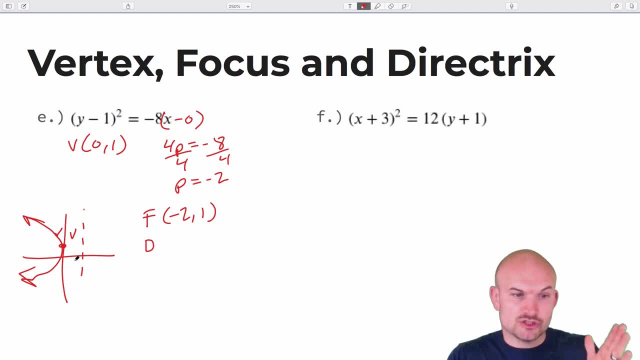 is going to be a vertical line right, Two units to the right of that vertex. So that's going to be: x equals a positive 2, right. Or you know, it'd be 0 minus a negative 2, which would give you. 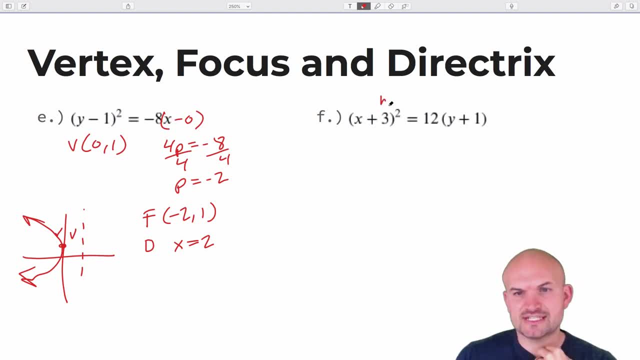 a positive. 2. In the next equation you can see that this is my h and this is my k, but notice how they're positives right. So again, like x minus negative, 3 quantity squared equals 12 times y minus a negative 1. Students still get confused with that. as far as identifying, 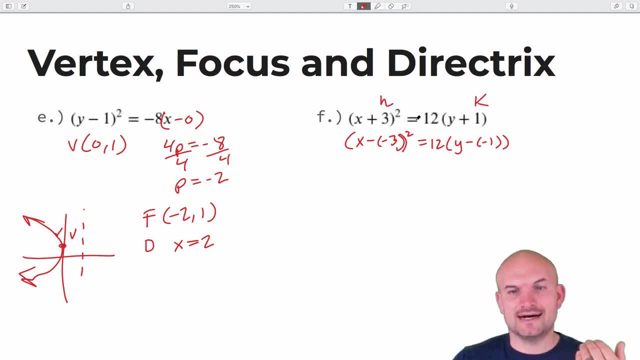 the h and the k. You know they want to take h as negative 1. But again you could, if you can see the formula remember is x minus h, y minus k. So you have your h and your k in. 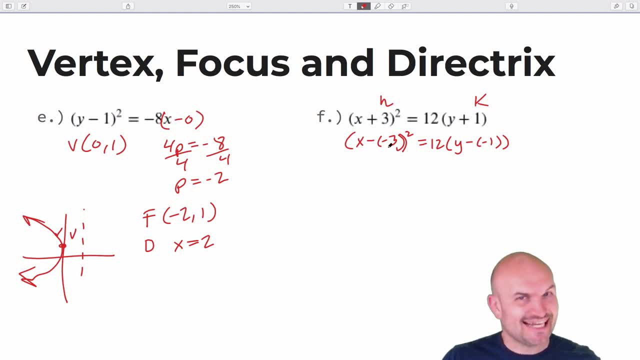 that regard. And so when you have the positive it's really minus a negative. So my vertex again: my h is with x, my k is with y. In this case it's going to be a negative 3,, negative 1,. 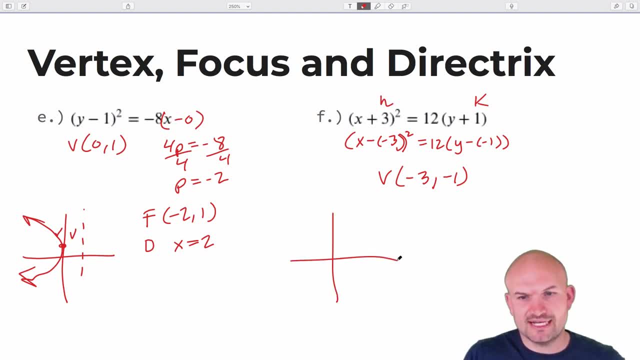 all right. So I'm going to go ahead and plot that just real quick to kind of get an idea. So negative 1, 2, 3, negative 1, all right. And now what we're going to do is: I see it's an x squared, So therefore I know it's going to go open up or down, But since my p 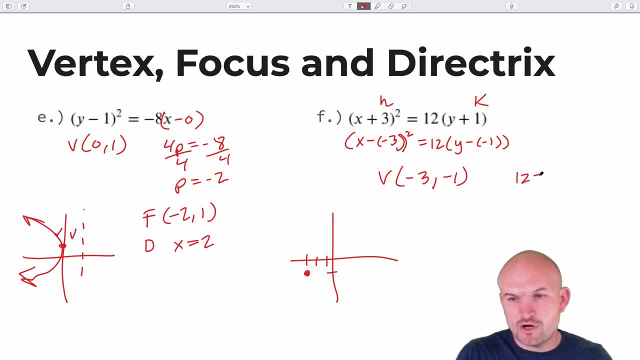 I know is going to be positive, right? So 12 equals 4p. We could just say p is equal to 3.. So therefore it's going to be up. So I know my parabola is going to open up And again, 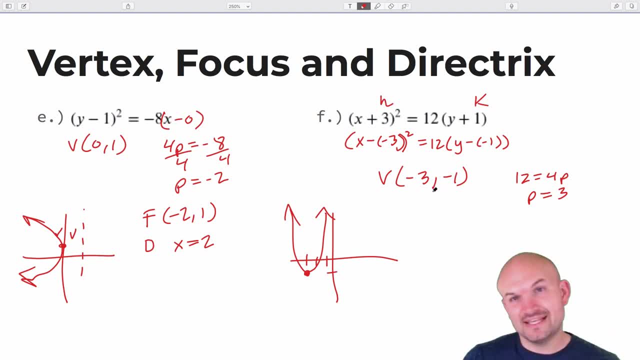 if I was trying to identify this now, here's where the formulas probably be helpful. right, You could easily count three units over. Hopefully you recognize that the x coordinate's not changing, Like if I'm just trying to find this focus, I'm just going up, right, So my focus is: 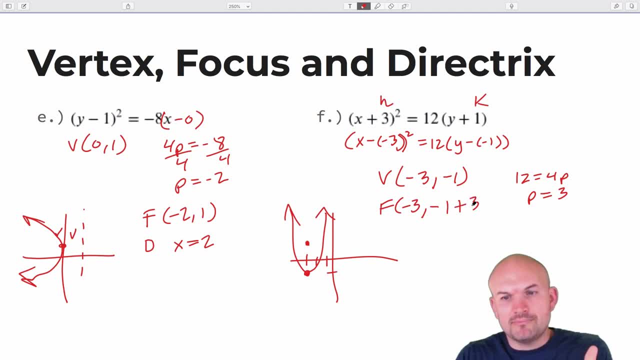 going to keep that x coordinate the same, but now it's going to be negative 1 plus 3.. So if I just take negative 3, and if I just move it up two units here, you can see that's going to be a. 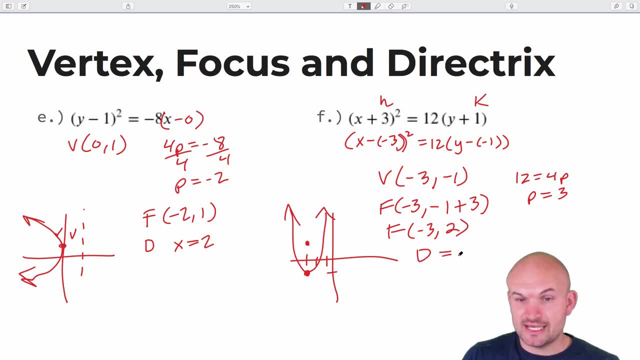 positive 2.. As far as my directrix, it's going to be the exact same thing. I have this value of negative 1.. So I'm going to have my directrix. I'll just write that. So it's going to be x equals. 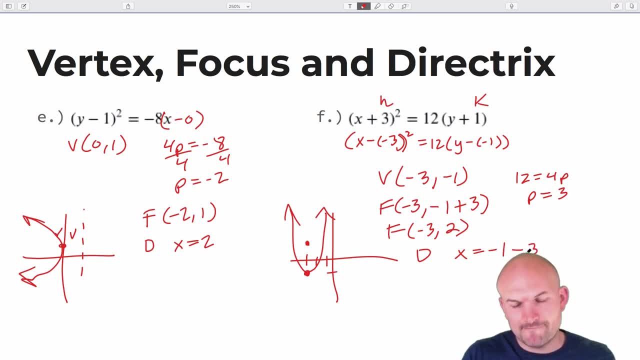 negative 1,, but it's going to be minus my value p, which is 3,. okay, So it's always going to be y coordinate, not minus. So I'm going to have x equals negative 1, but it's going to be minus my. 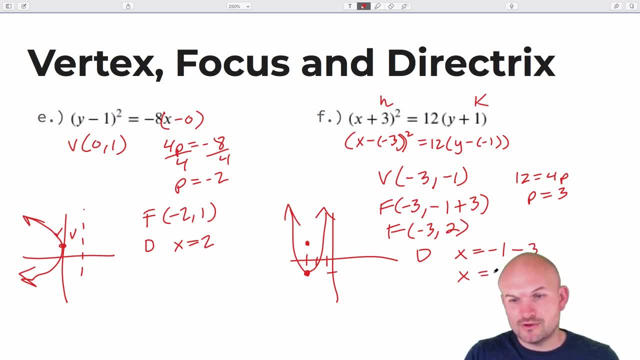 value minus that. So x equals negative, 1 minus 3 is going to equal a negative 4.. 1, 2,, 3, 4, which again would make sense here. right And again, that's going to be a, not an x, that is a. 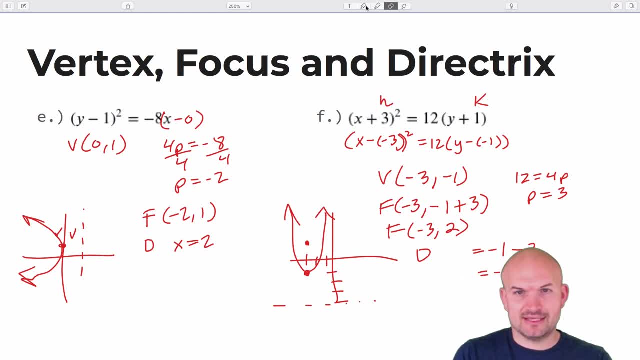 y Ah, see, you can see me making these mistakes. Jeez, slow down, Okay. So that's basically the idea when you have something in standard form, But typically students, once they kind of get the practice of that, they're like: all right, I feel kind of comfortable with that material. 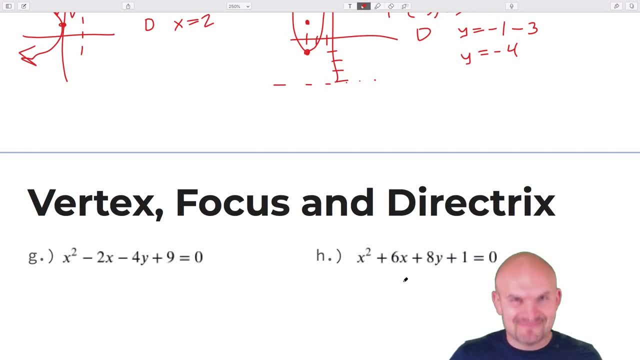 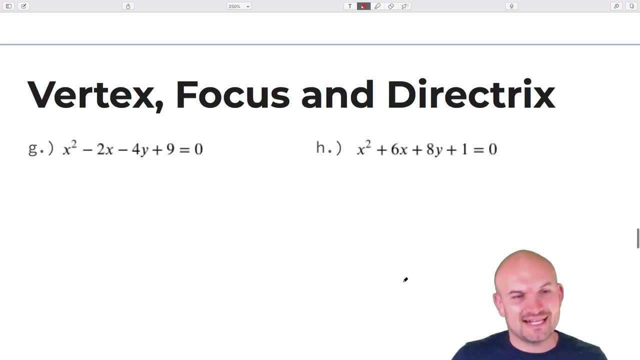 What else do you got? And that's where we bring into completing the square And that's where a lot of students are like, ah man, we spent all that time and now I got to go back and remember all of that completing the square stuff. 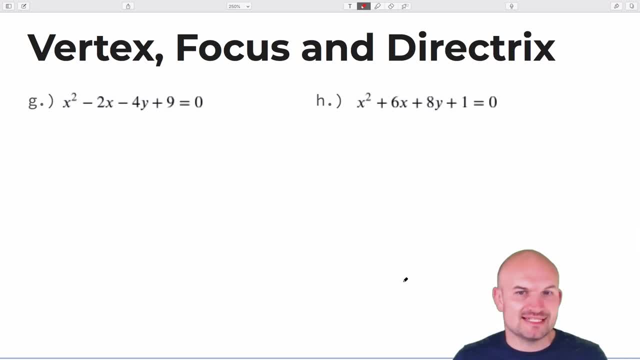 So really, the only difference with these problems, guys, is you're just going to have to complete the square first and then work to it. I think I gave four problems just because students still just need more practice with this. So what I'm going to do is just do these completing the square. 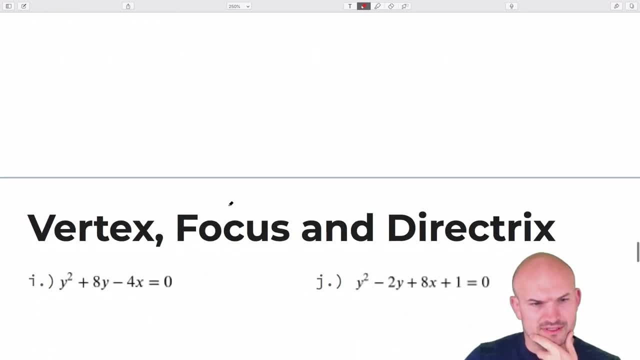 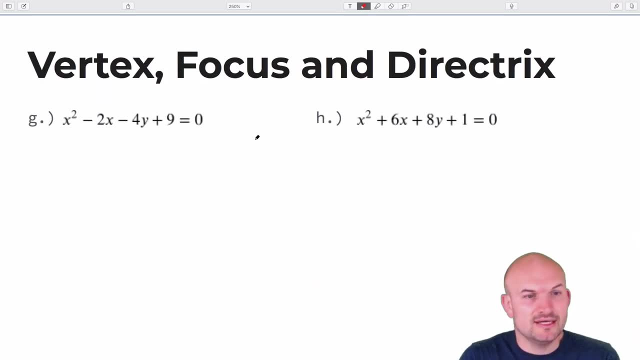 Do these have coefficients? No, they don't. So, hmm, all right. So what I'm going to do is I'm just going to kind of work through these rather kind of quickly. I'm not going to go through the completing the square process just because we have already done. 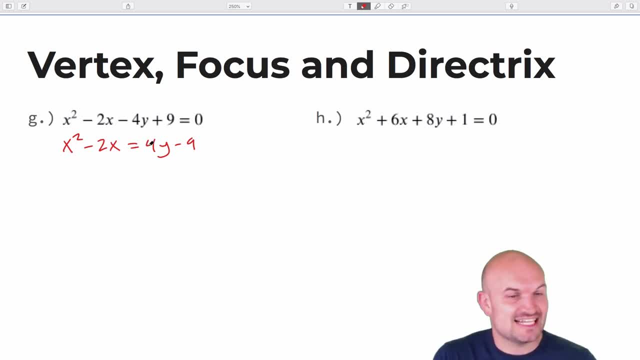 that kind of extensively in this class, or in the last chapter at least. So first thing I'm going to do is I'm going to separate the x's and the y's to get them on opposite sides, And then I'm going to complete the square here. Hopefully you recognize, to complete the square I'm going to. 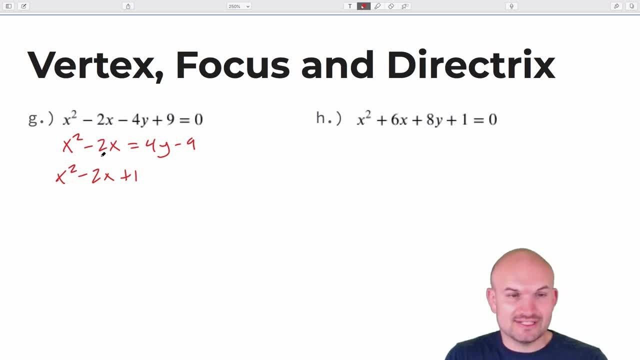 want to add a one. Or you could take the b divided by two and square it: Negative two divided by two is negative one. Negative squared is one. But remember, if you add a one to the left-hand side, you need to add a one. 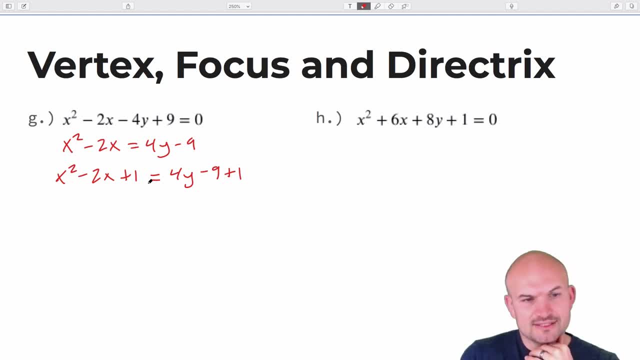 to the right-hand side. Now this goes, and now I can factor that down into a binomial: squared. Oops, that's supposed to be a one, which is what we were looking for. And then over here we have a 4y. 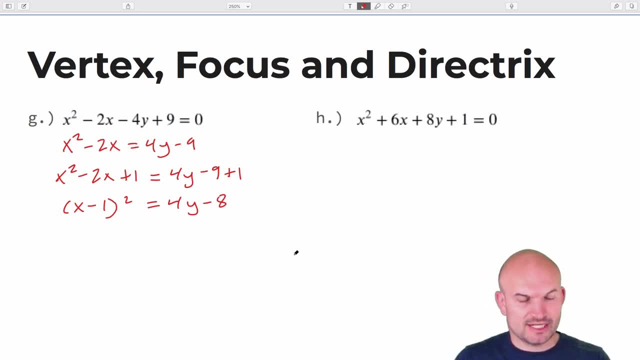 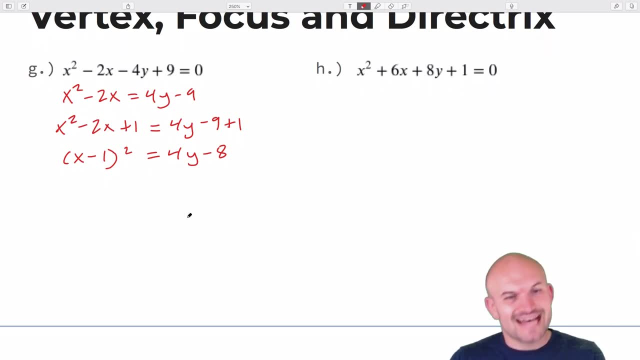 minus eight. Now, one of the reasons I wanted to do this- or I wanted to kind of cover these problems- is we don't want to write our identifier vertex in this case, If you look at the formulas, it's four p times y minus k. So in this case, what I'm going to want to do here is do x minus one quantity. 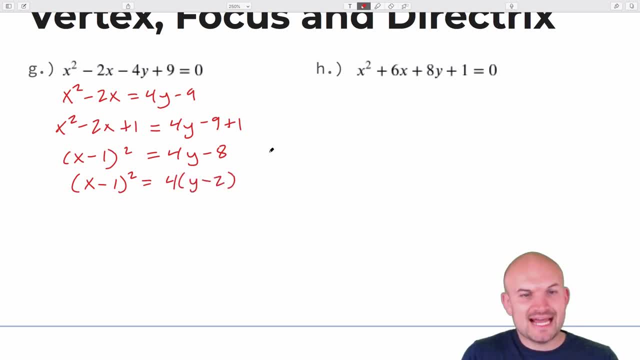 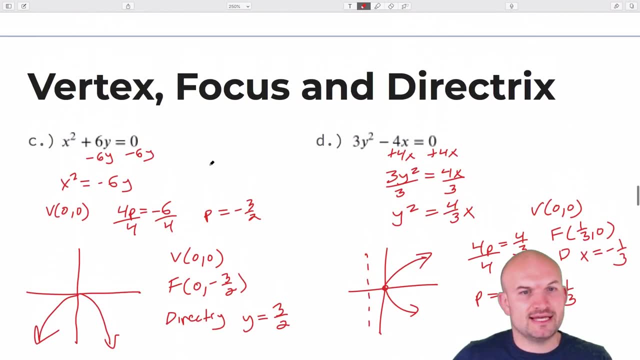 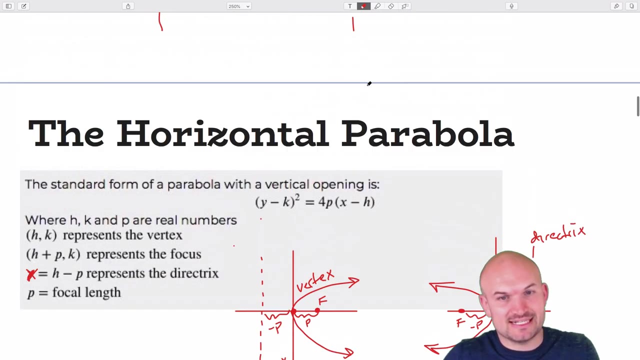 squared, I need to factor out the four, And that is the big, big step that students miss. is that factoring out the four? Okay? Because, again, look at the formulas that we did right. It is all the way up here. all the way up here. It's four p times x minus h, or it's going to be four p times y. 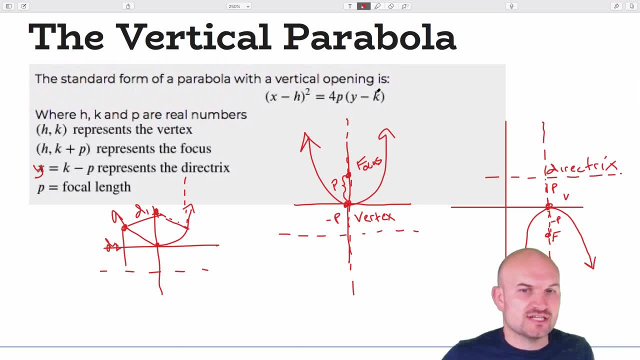 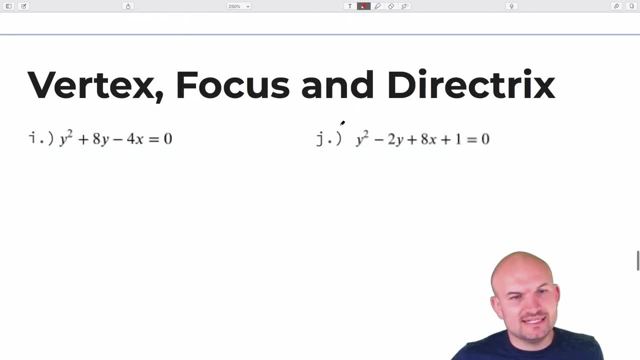 minus k. So you got to make sure you factor out, you got to make sure that coefficients of your x or your ys is going to be one, And then you can go ahead and apply the same kind of techniques that we did before here. In this case, we know that my x is squared, so it's going to open up. 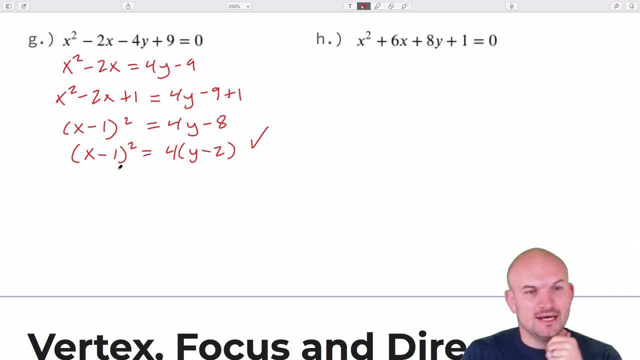 or down. We know my p is going to be positive, so it's going to open up. And now I'm just going to kind of quickly do this as long as the numbers work out. So my vertex is one comma two, My value: 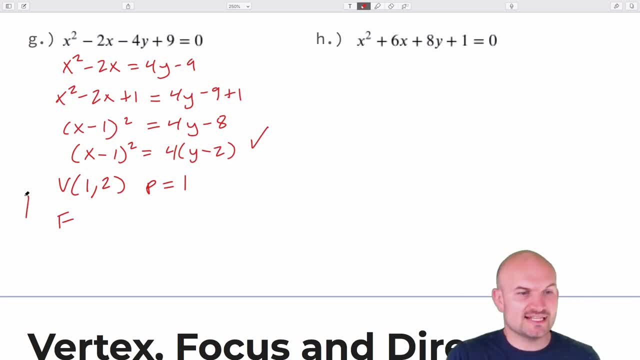 of p is going to equal one. Since I know that it's going to open up, my new vertex is going to have, I'm going to add one to the y coordinate. So that's going to be one comma three And my directrix is again going to be a horizontal line. 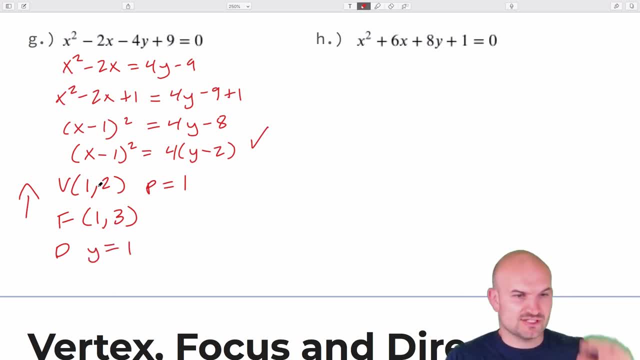 right. So that's going to be: y equals one, Because so, basically, I'm just going to take two and then I'm going to subtract one from it, And again, this is something that we have covered extensively now, So this is something that I do. I'd have the students go up to the board and do this, So 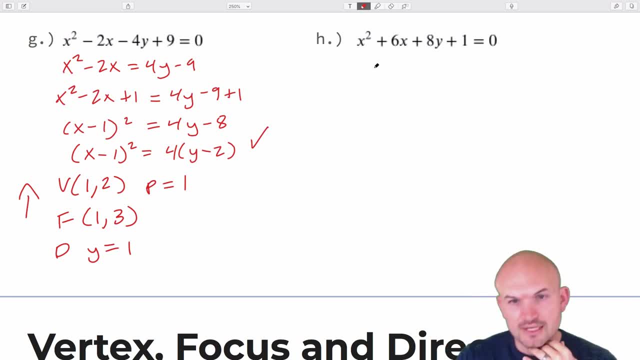 that's why I'm kind of running through these problems a little bit quicker. Same thing. First thing I'm going to do is separate the x's and the y's, So therefore this would be a negative eight minus one. Now I'm going to complete the square Again, to complete the square of the middle term. 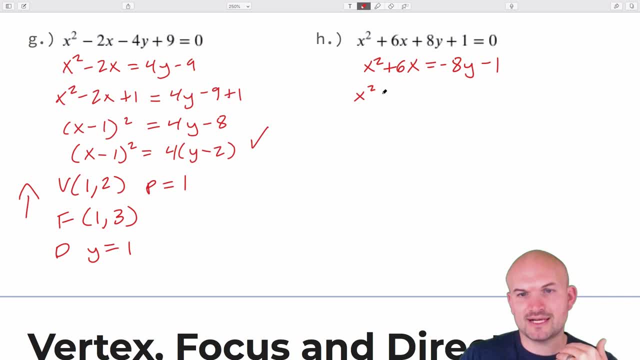 of six. you could do your b divided by two squared, or. hopefully you recognize at this point that I'm going to want to add a nine to both sides. So in this case I have a negative eight, y minus one plus nine. That can now be simplified to an x plus three, quantity squared. And then here again, 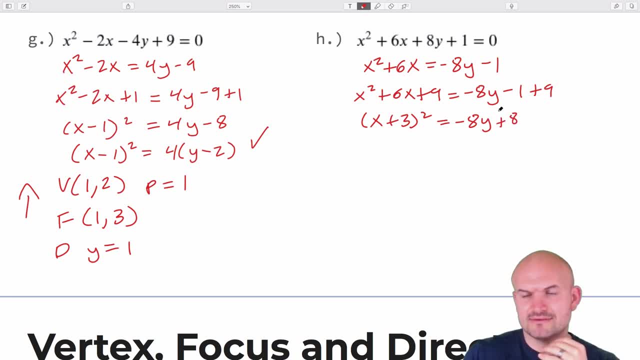 you're going to have a negative eight y plus eight. So again factor out that negative eight, right? So we get a negative eight times a y plus one. All right, Now again you can see that my x is squared, which is fine. So therefore my vertex is a negative three comma, negative one, And my p is: 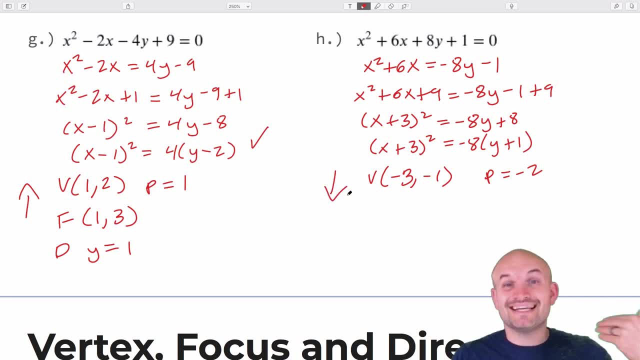 going to equal negative two. So that tells me. now my graph is going to be opening down right. So if I have my vertex here and again, sometimes it's just helpful, like again, to plot it: negative one, two, three, negative one. So there is my vertex. So my focus is going to be going down two. 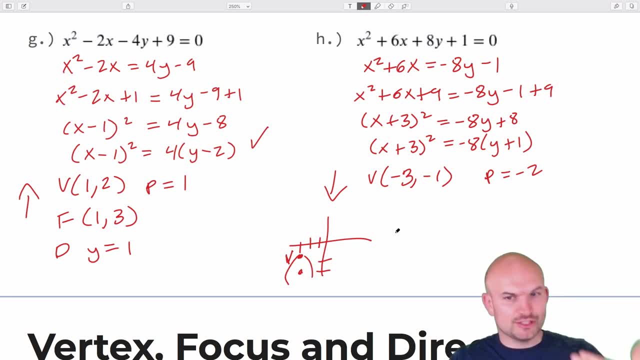 units. Sometimes just by graphing it you can identify, like, what the new focus is. But all I'm going to do is just add negative two to negative one. So therefore it's going to be negative two minus one, right, You're adding p. If you look at the formulas, I didn't do it over in this case. 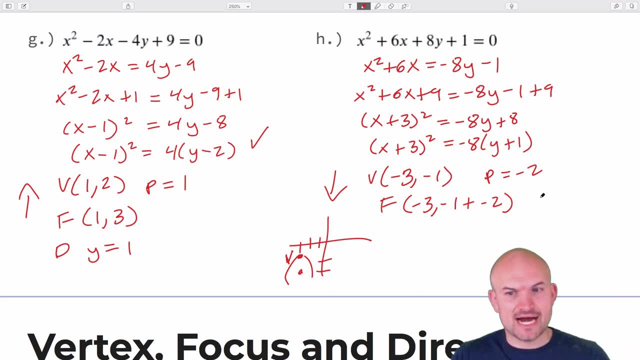 But if you add p to your y coordinate, that's going to move it down. So that's going to take us to a negative three, negative three, which again makes sense here into the context of my graph, And then for my directrix again. 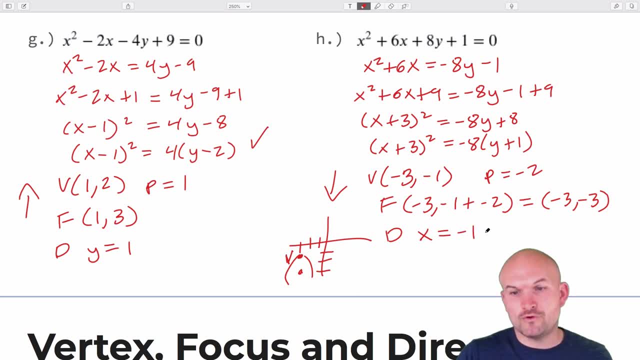 I'm going to have my x and my y coordinate. It's going to take me down to, let's say, this is going to be a vertical line. That's going to be: x equals a negative one minus a negative two, And you can see, in that case, one two that's going to give me this line here, which is going to equal a. 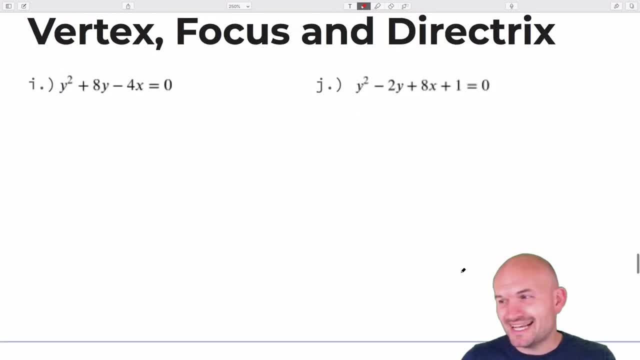 positive one. So our x equals a positive one. All right, now we just have two problems: that we were completing the square with ys, which, again, guys, is not really going to make much of a difference. x and y coordinates open up to the left and to the right. 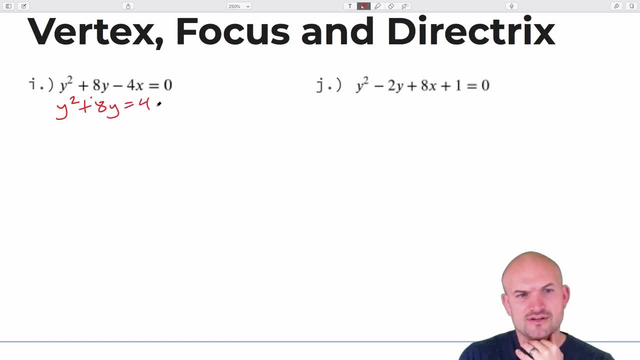 So I'll have a y squared plus 8y equals 4x. Complete the square when my middle term is 8.. So you could do 8 divided by 2, which is 4.. 4 squared is 16.. Or hopefully you already recognize that would be 8y plus 16.. 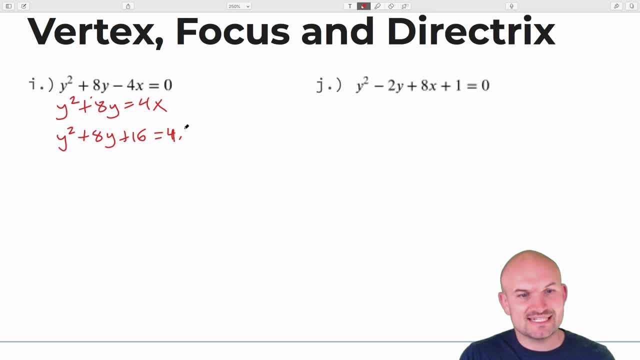 And again, just make sure you subtract or add a 16 to both sides, right, Because you got to keep that equation true. Now I can factor this out. So this becomes a y plus 4, quantity squared, And I can factor out a 4 here. 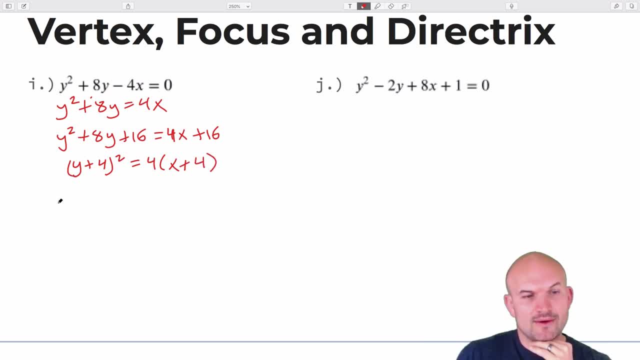 So that becomes an x plus 4.. Okay, so now we can identify my vertex. Remember, everything's switched: X is with h, y is with k. In this one it doesn't really matter, because they're both the same. 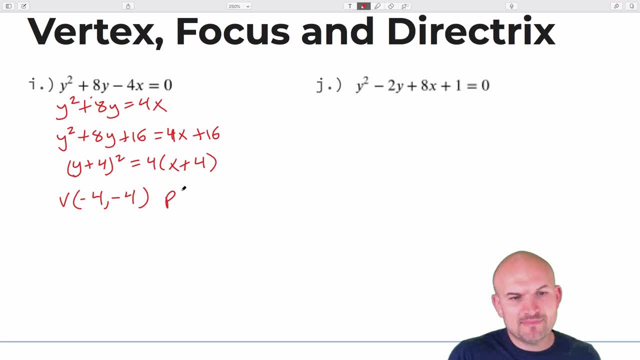 But just kind of be careful with that. And then my p is going to be 1, right 4p equals 4.. So therefore, p is equal to 1.. Since p is positive and my y is squared, I know the graph is going to open up to the right. 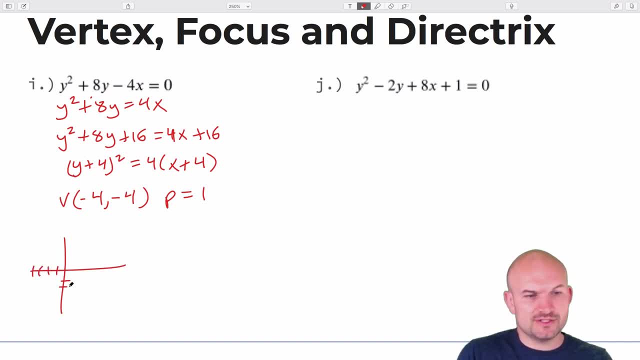 So I'm just going to go ahead and sketch this: 1., 2., 3., 4.. 1., 2., 3., 4.. Okay, and I know it's going to open up to the right. 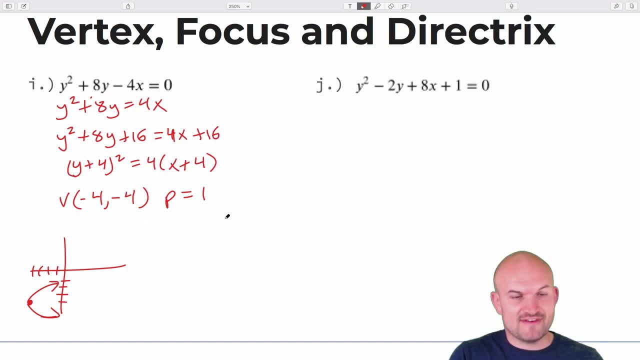 However, just kind of going with the idea here is: if I'm moving this focus to the right, make sure that you add that 1 to the x-coordinate. right, The y-coordinate is going to remain the same, But the x-coordinate is now going to be a negative 3, negative 4, which makes sense, right? 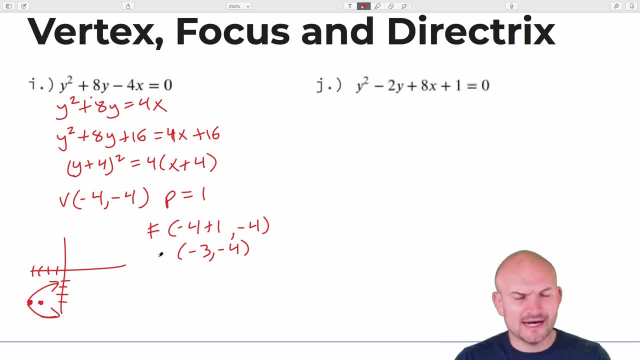 You'd have a negative 3, negative 4.. But again, you could easily just do that in your head. You don't really need to show this. So I'm just showing this work at least one time and then I'll do the other one quicker. 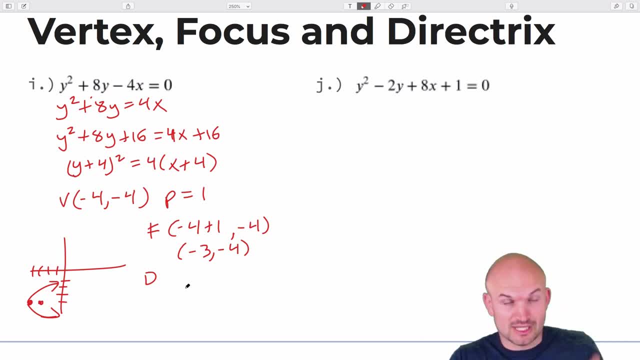 The directrix, then, is going to be that same thing. It's going to be a vertical line, though, So that's going to be: x equals a negative 4 minus 1, right, Because you're subtracting p. So in this case, negative 4 minus 1 is equal to a negative 5.. 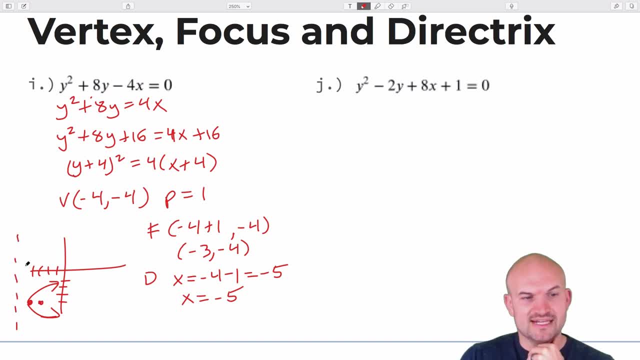 So x equals a negative 5, which again makes sense, right? You're going to have that value to the right or to the left of your vertex, All right, Last one, Let's go ahead and just again separate. 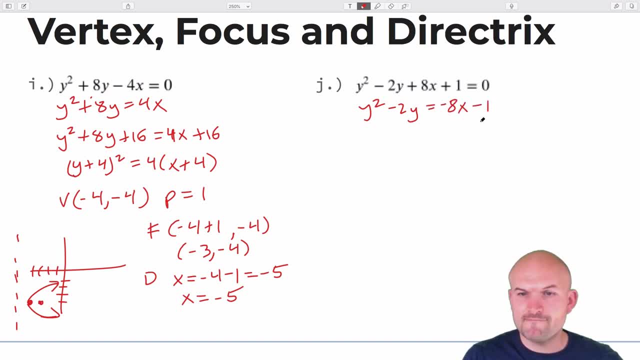 So minus 2y equals a negative 8x minus 1.. Again, you're going to want to factor out that 8.. But before we do that, though, let's complete the square right, Because I'm like, eh, that's not going to be fun to factor that out. 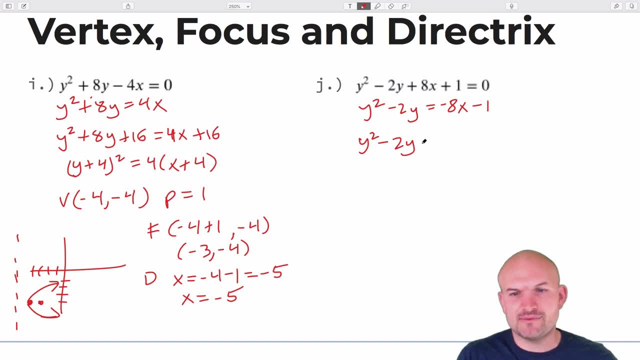 So if I go ahead and complete the square here, that's going to be a positive 1.. So therefore, in this case, if I have negative 8x minus 1 plus 1, you can see that. oh, I don't have to factor this out. 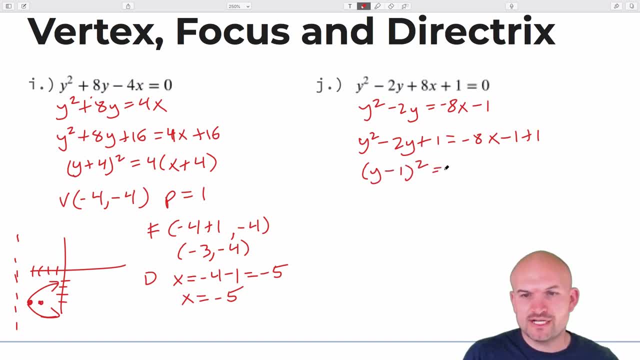 This can be. I can actually factor down into a y minus 1 quantity squared equals a negative 8x. Now again, remember that you could also rewrite this as a y minus 1 quantity squared equals a negative 8 times x minus 0.. 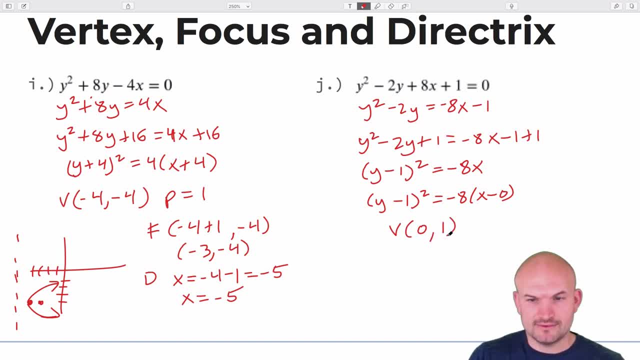 It's just sometimes important to remember your vertex. here is 0 comma 1, right. H is always with x, k is always with y. So now, in this case, we have your vertex as 0 comma 1.. We can see that p is going to be a negative 2, right. 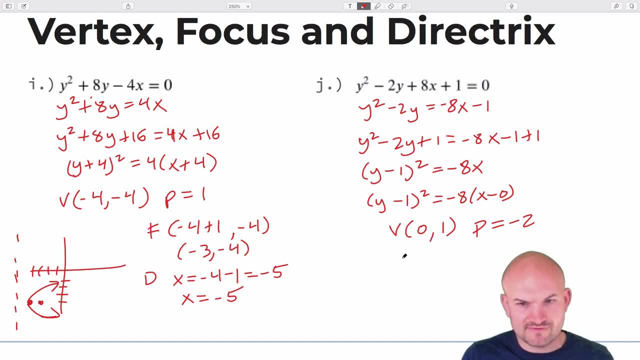 Negative, 8 equals 4p. divide by 4 on both sides, p equals negative 2.. Let's just go and sketch a graph here. Since y is squared, we know it opens up left to right. Since p is negative, we know it's going to open up to the left. 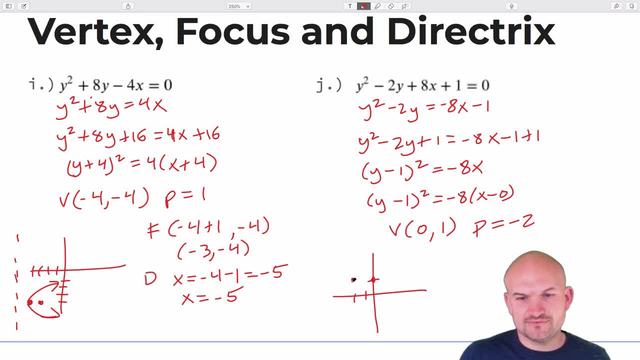 So do 0,, 1, okay, And p is negative 2.. So we know our graph is going to look something like that, And even just by sketching it right here, you can see that. oh, I already kind of found the vertex. 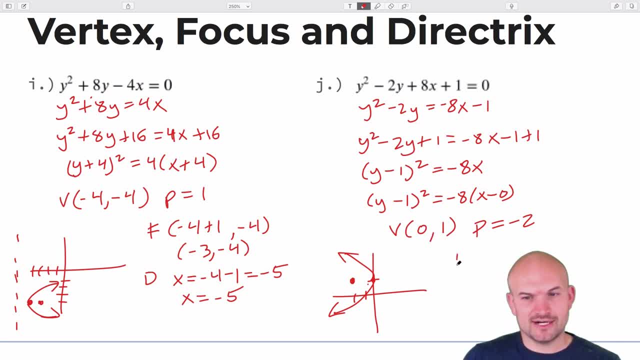 But again, like you know, you're going to add a negative 2 to the x coordinate here, which is kind of simple, That's negative. So you're going to add a negative 2, 1, which is obvious also from the graph. 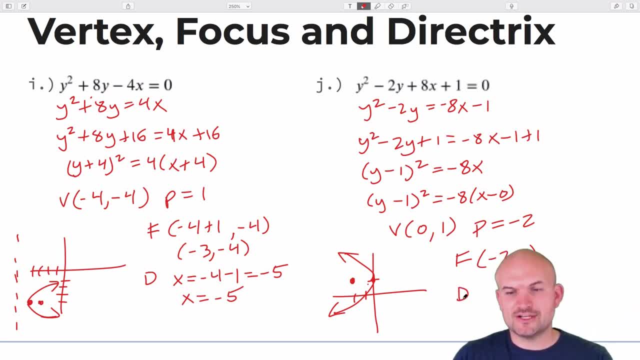 And then you're going to subtract the negative 2 or just go to the right to find the directrix. Just remember it's a vertical line, so it's going to be: x equals a positive 2.. All right, So that's basically identifying the vertex focus and the directrix. 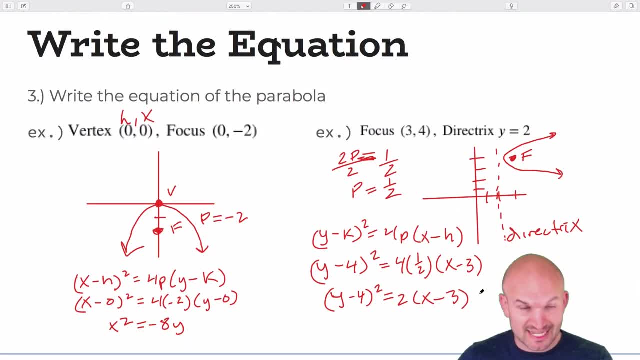 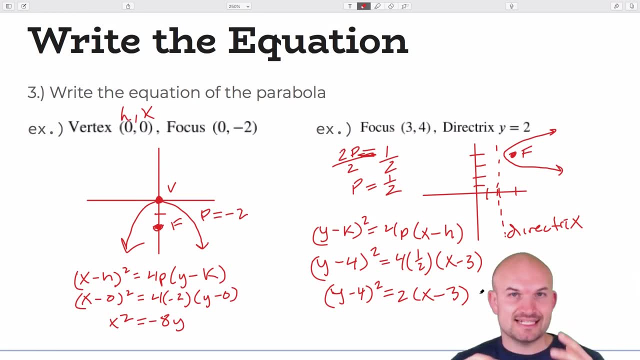 But what about if I gave you the vertex, focus and the directrix and I asked you to write the equation? Now, the one thing that I think is the the constant throughout this whole chapter is plotting the information. Whenever you're writing the equation, plot the information. 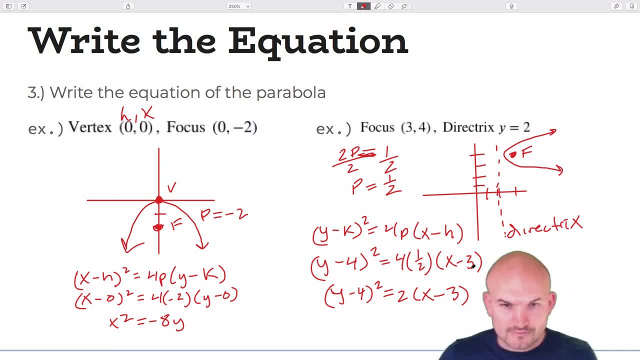 This is one of the first things that we want to do when we're trying to like understand writing the equation. I'm not going to scroll all the way back up, But even that first problem, like we understand, we have a vertex. Okay, what do we know about a vertex? 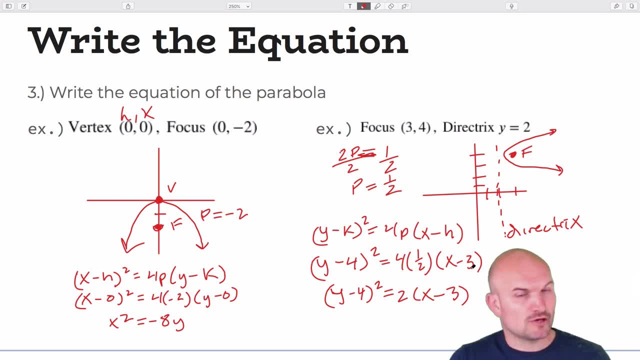 We can represent that as h and k. Oh, we have a coordinate point. How can we represent that? We can represent that as an x and y. So if you're given the vertex in the focus, plot those points on the graph. 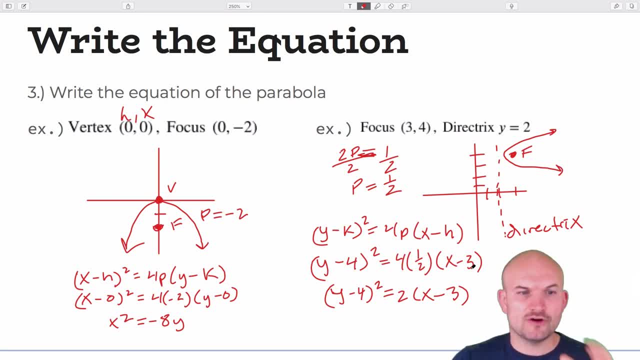 Because remember one thing that we know: we know that the vertex always opens up towards the focus. We know that the directrix is always perpendicular to the axis of symmetry. So in this case, we're given the vertex and the focus. I plot the vertex, I plot the focus. 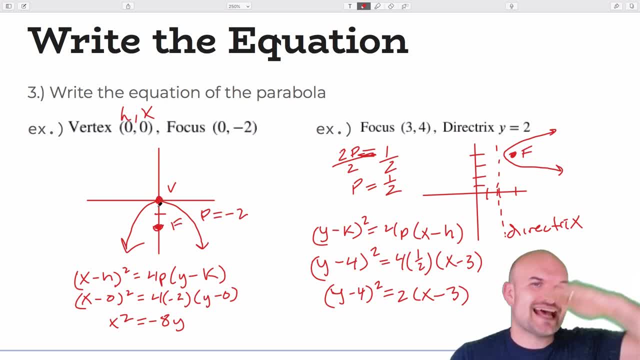 Just by that information alone, I'm able to determine that the vertex has to open down and that p is going to be negative. right, It has to be. it's going to open down. So I mean it's going to be a vertical and it's going to be a p is going to be negative. 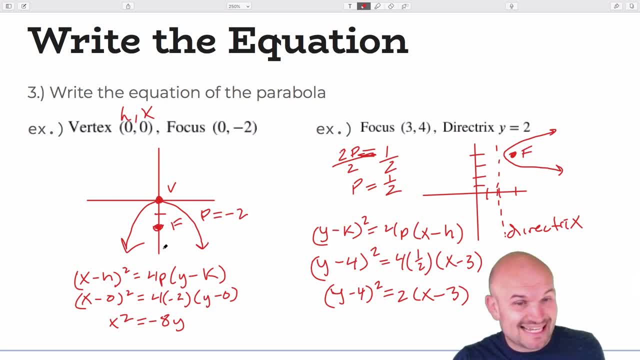 Since it's vertical. I'm going to use this equation And remember: p is the distance from the vertex to my focus. Well, since we're going down, it's going to be a negative two. So then all we do is we plug in our coordinates for our vertex, which in this case is h, k. 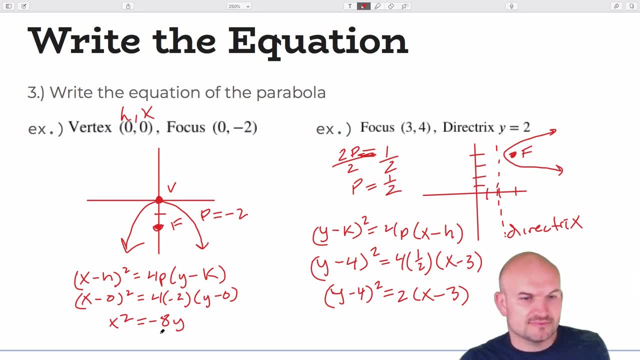 So it's going to be zero and zero And then we plug in negative two in for p, And therefore you can see we get an x squared equals negative eight y. Now next equation we have a focus is three comma four, and our directrix is: y equals negative. 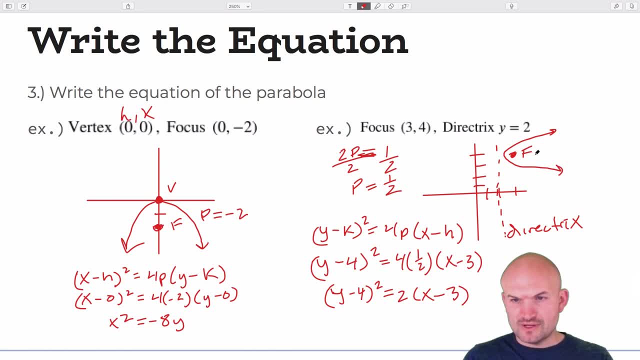 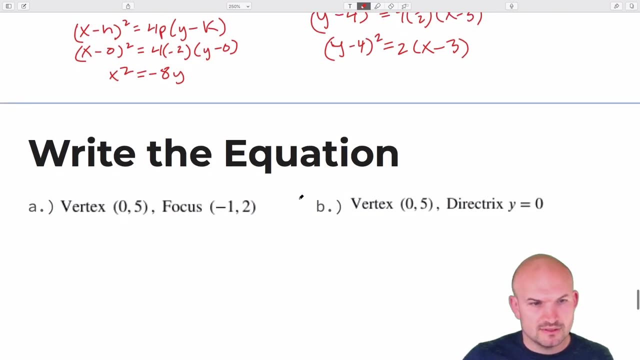 eight. So that's at y equals two Again. so I plot the focus here and I plot the directrix, which is at y equals two, which is incorrect, because I think that was supposed to be hold on a second. I think that was supposed to be x equals. actually I did not do y equals zero. 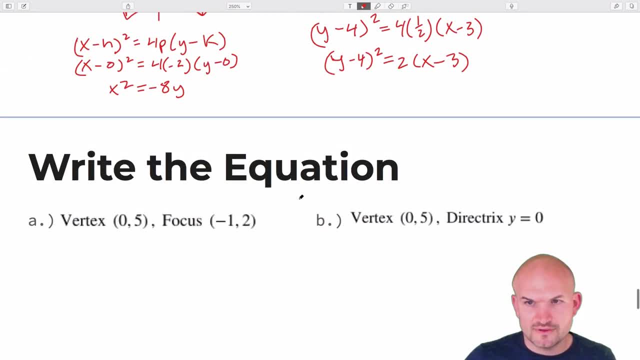 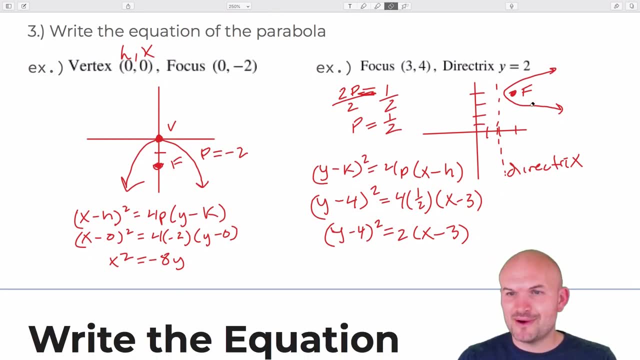 Directrix: x equals negative two. x equals negative two yy. Yeah, geez, I can't believe I did this problem wrong. Crazy me, All right, so let's go and do another problem here, because I did this wrong. 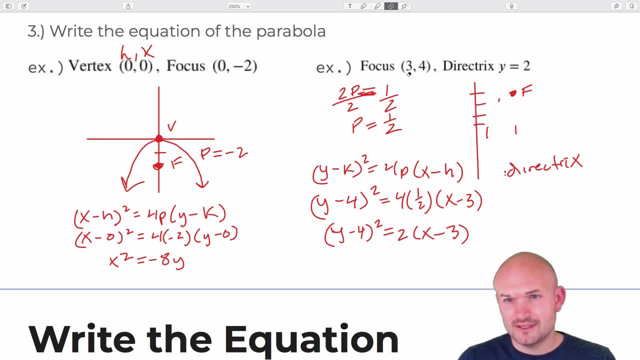 I did this wrong. That's a vertical directrix. right Vertical directrix is not correct. If your directrix is, y equals two, that's a horizontal line. So my formula is all wrong. Geez, I guess I get to highlight me making a mistake in front of you guys, but that's. 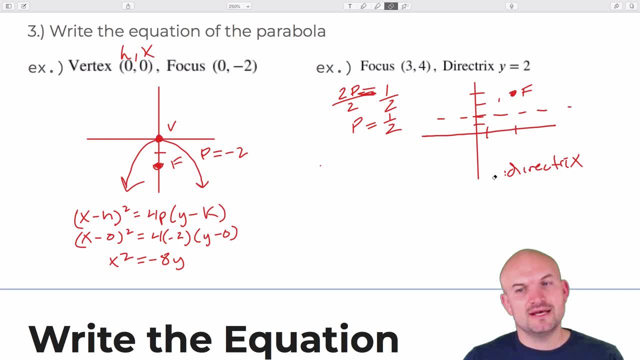 okay, because that's part of, like the slowing down process, right, And that's why I think it's so helpful to sketch the graph So you can visually see what's going on. So here's my focus, Here's my directrix. 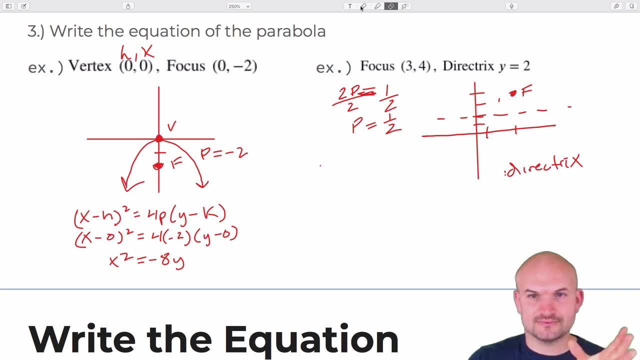 Now the important thing is you can understand the distance. okay, If here's my directrix, here's my focus. So I know that my vertex, which we need to identify, is going to be over two. My problem is, we just need to be able to figure out, like, what is the distance between my 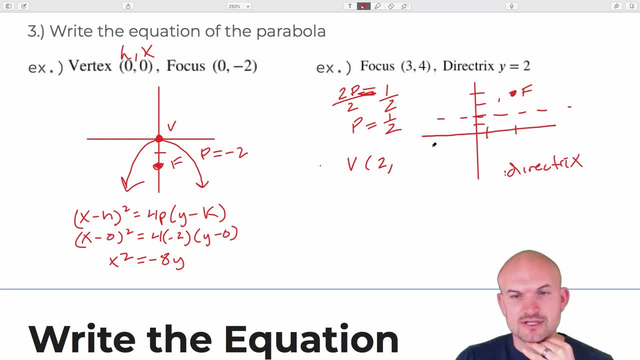 vertex and my directrix. So the problem is, you know, if we have, We have three comma four, so we're up three. So let's do this. Did I do this One? Okay, So one, two, three and that four. 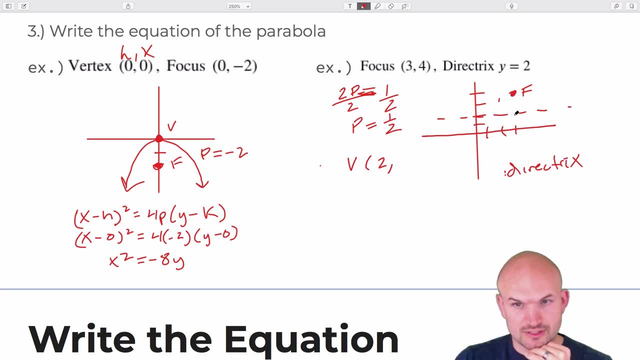 One, two, three, four, right, And my directrix is that y equals two. Oh, I wrote that. Oh man, All right, So let's just kind of go through this idea here. So I, Man, I've messed up this problem all the way. 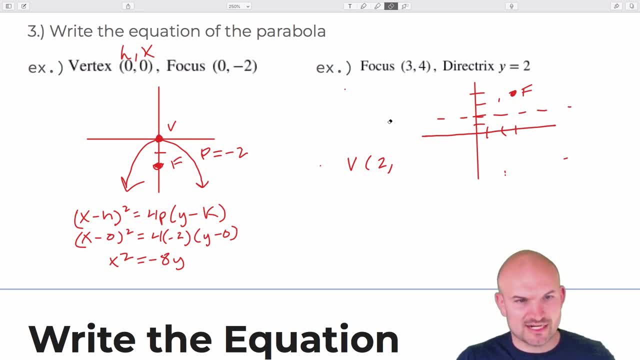 All right, So I plotted my focus and I directrix Again. what is something that we know about our vertex and directrix? And let's actually go to this equation right here, If you, This isn't something we've talked about yet. 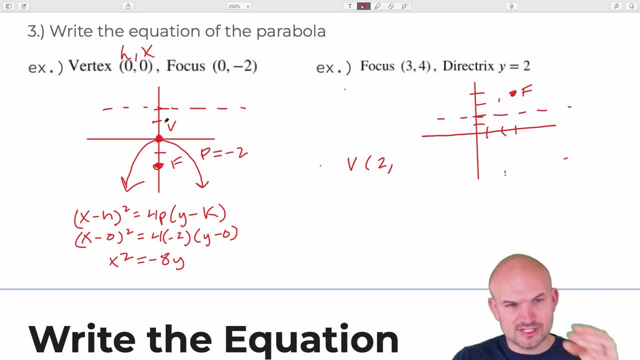 If you look at the focus and the vertex and the directrix, you understand that to go from the vertex, you know, to the focus, that's p, And then to go from the vertex to the directrix, that's opposite of p, right, 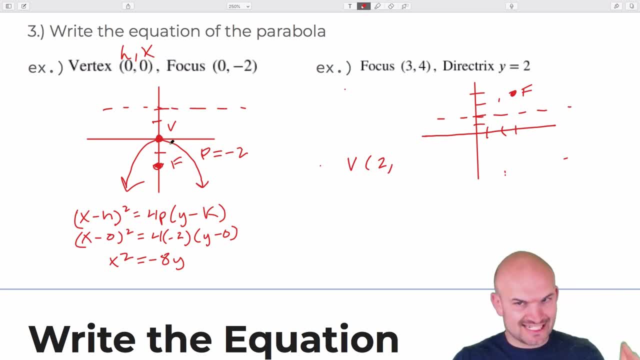 You add p subtract p, So therefore the vertex is directly in between the focus and the directrix, Right? So if I have my directrix and I have my focus, then my vertex is going to be right in the middle between them. 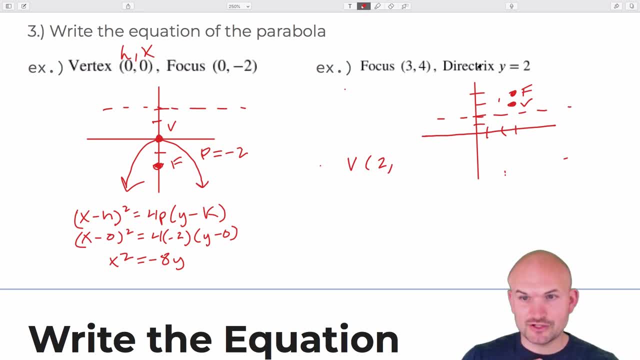 So if I have a focus at three, four and a directrix at you know, two, I know it has to be over, Like the vertex and the focus are going to lie in the same line of symmetry. But my vertex here is basically going to be at three comma three. 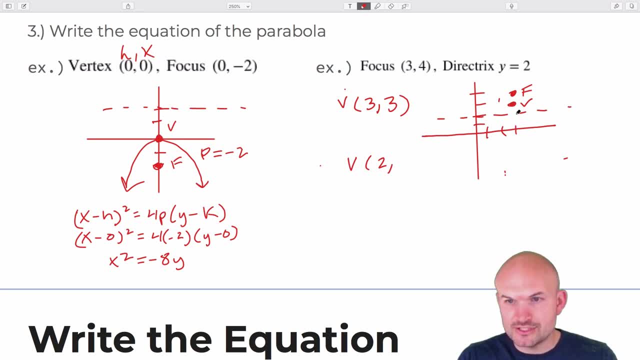 It's going to be right in between. So one, two, three, And let's go. one, two, three. It's going to be right in between the vertex And the focus, because the distance from my vertex to my focus is positive one. 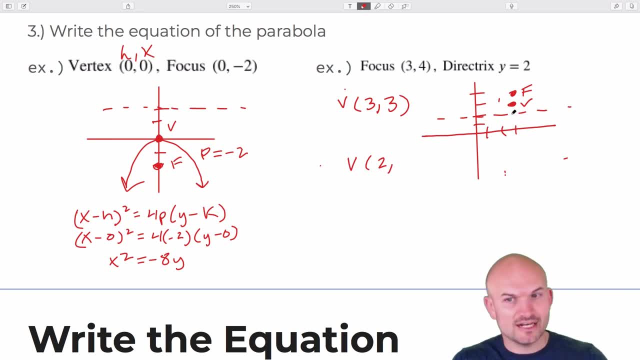 The distance from my vertex to my directrix is going to be, you know, negative one in the opposite direction, or going down one. So I don't know what I was thinking when I was doing this problem earlier, but now I have my vertex and I can say the distance from my vertex to my focus is one, but it's. 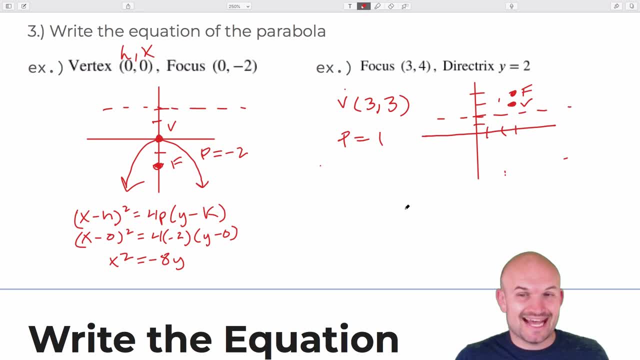 going up. So therefore p is going to be a positive one. This again, is another vertical parabola, So that's going to be x. let's see minus h. So I'm going to use the same equation: Equals four p times y minus k. okay, 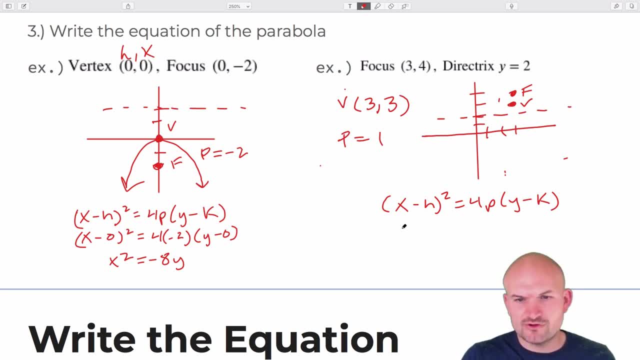 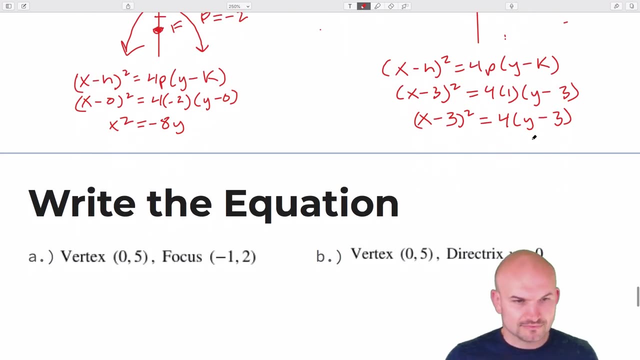 So now I'll just plug in my vertex, which is going to be: a x minus three, quantity squared equals four times one times y minus three. So I have a final answer of x minus three, quantity squared times four times y minus three. okay, 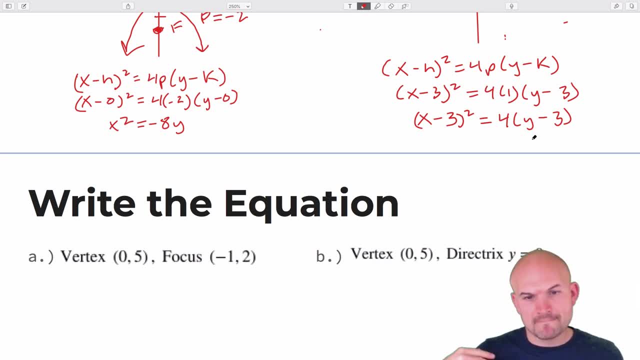 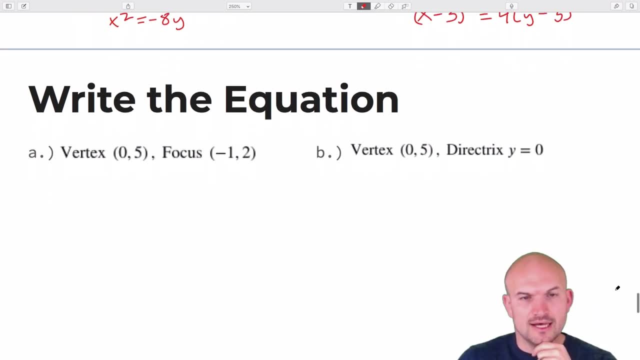 So now what I did is I just kind of gave the students last four problems again that they would work on in their groups, And then they'd go ahead and present those on the board. So let's go and take a look at the problems that my students would have had to work on. 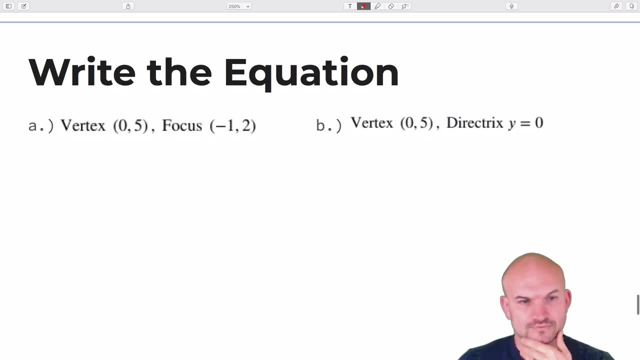 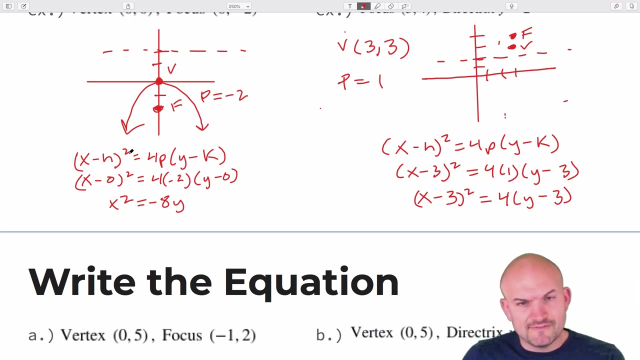 and doing the same thing. It's just writing the equation, writing the equation of the parabola in our standard form. Oh, and one thing actually, before I get into this: if you remember we did, if you remember, at the beginning, the first problem we did was writing it, and actually in standard form. 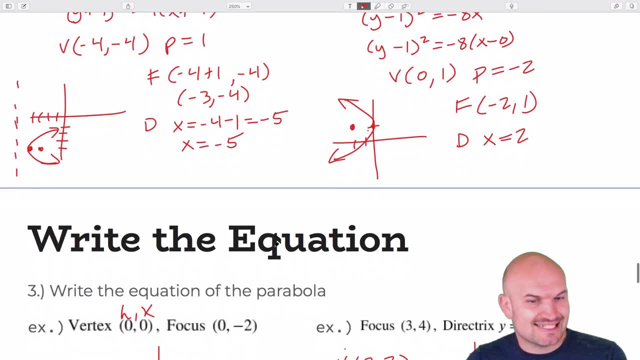 okay. So let's go ahead and take a look at the problem that we did. So let's go ahead and take a look at the problem that we did, and actually in general form. in this case, we could do that exact same thing here. 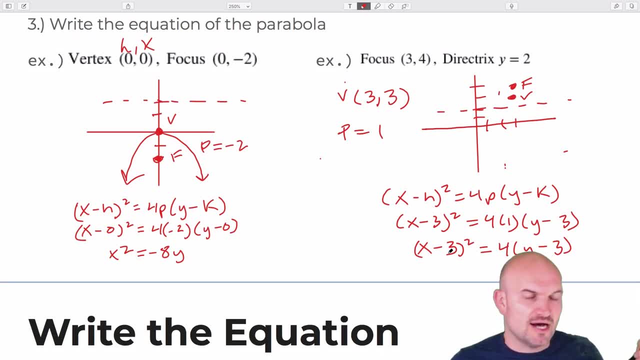 The only thing we'd need to do is we just need to expand this and then get all of our values on the same side. So that's just another thing I just wanted to recognize. I'm not- I don't spend the time with my students doing that, but it is something that I want. 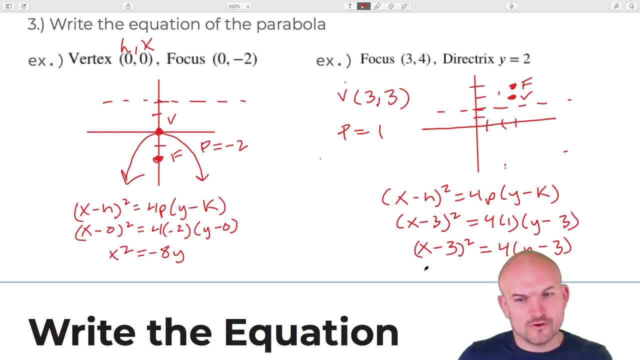 to make sure that they're aware of. If they need to identify it in general form, they would just expand it and then get all the terms to the same side. All right, So again, first thing we're going to want to do is plot the points. 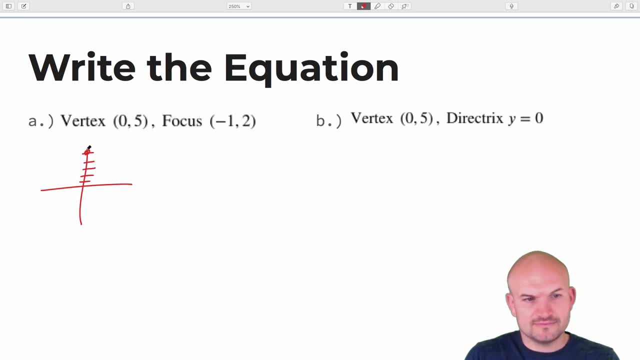 So I have: vertex is 0,, 5,, 1, 2,, 3,, 4, 5.. And my focus is at negative 1, 2.. That's not supposed to be. that's going to be negative 2,. ah geez, how did I not check? 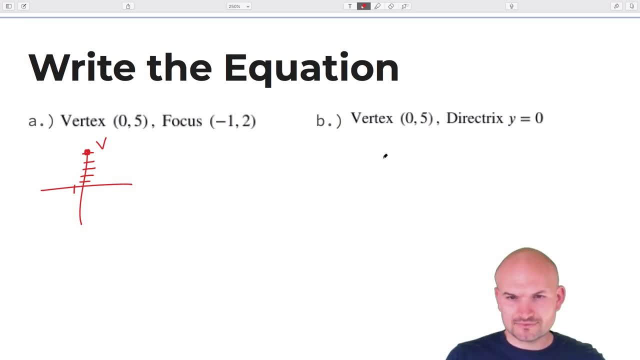 that out. Um, let's skip it and we'll come back to that one because I'll- uh, I'll fit I. there's a typo there and I don't know if it was supposed to be um a 2 or a 5, but if that's actually, 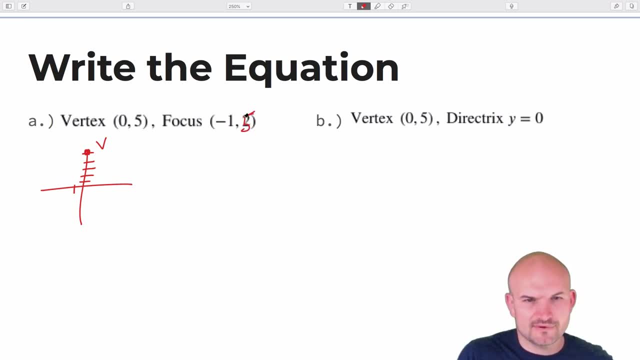 if that's supposed to be negative 2,, let's just do negative 2, 5 and I'll come back and fix that. So if this is going to be a negative 1, 5, there's my focus, Okay. 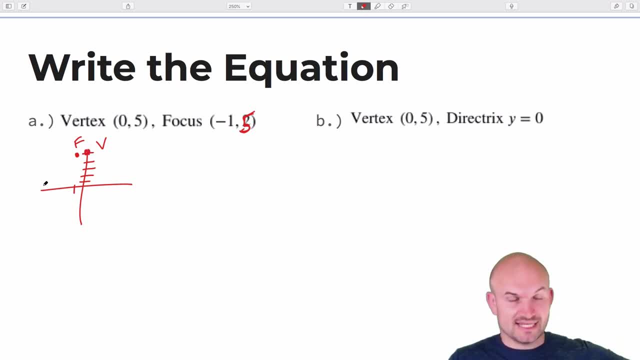 So now you can see that my vertex is going to be opening these up horizontally And since we're going to the left, P needs to be negative, All right. So, um, my formula here is: Y minus K, quantity squared equals 4P times X minus H. So again, 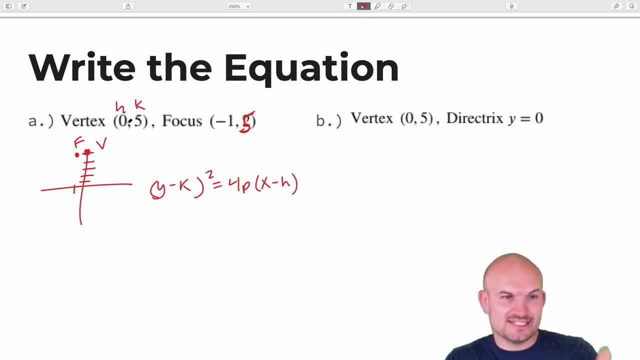 this is my H and this is my K right, And the distance here from my vertex to my focus is one. But again, since it's going to the left, it's going to be a negative. So this will be Y minus K, So it's going to be Y minus 5. quantity squared equals 4 times. 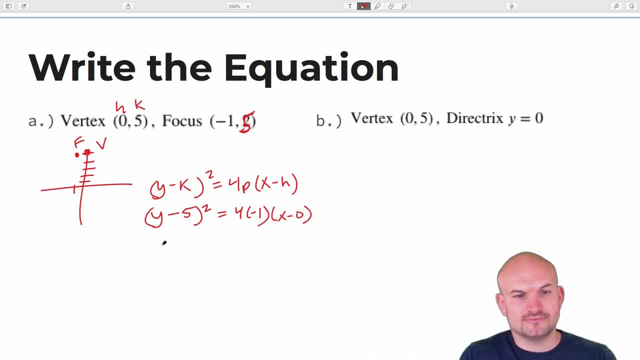 negative 1 times X minus 0.. So therefore I'd have Y minus 5, quantity squared equals a negative 4X Um. and next equation, Y is equal to 0.. Next equation we're going to have again another vertex at 0 comma, 5, 1,, 2,, 3,, 4, 5.. 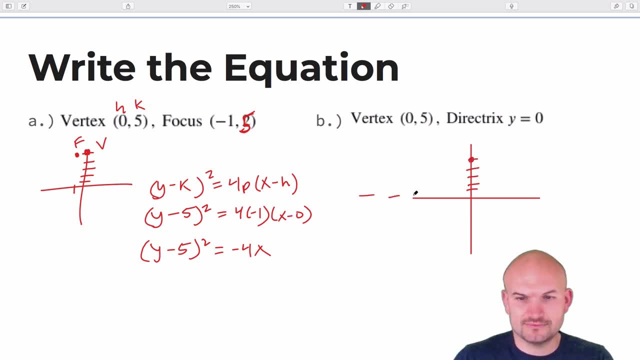 But in this case my directrix is at 0, or Y equals 0.. Okay, So there's my vertex and there's my directrix. That means my focus now is going to be: or again, remember the distance from the vertex. 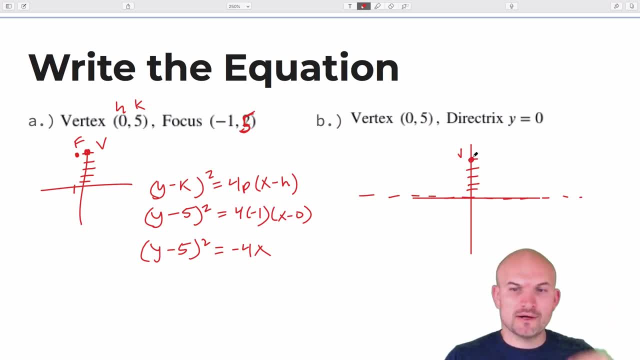 to the directrix is opposite of P right. So therefore, my focus is going to be up here. Well, how far should it be? Well, again, the distance from the vertex to the directrix is the same as the distance from the vertex to the focus. 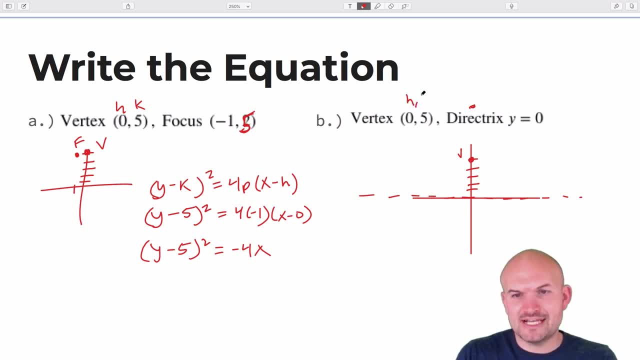 It's just an opposite directions. So this is going to be my H and my K. This is going to be my focus, which is going to be equal to 5, right, So my P is going to equal 5 in this case. 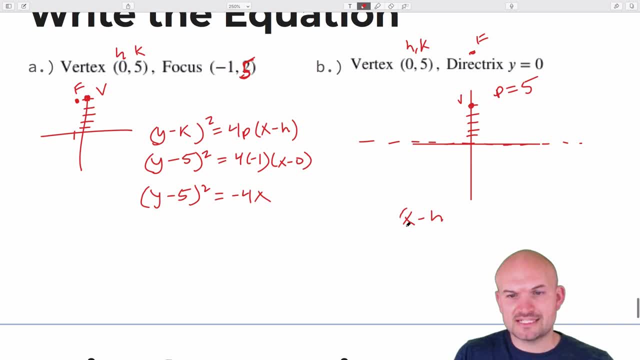 Again, this is a vertical parabola. So using the formula X minus H, quantity squared is equal to 4P times Y minus K. Again, I'm not sure why I use the same H and K in this case, but I did. 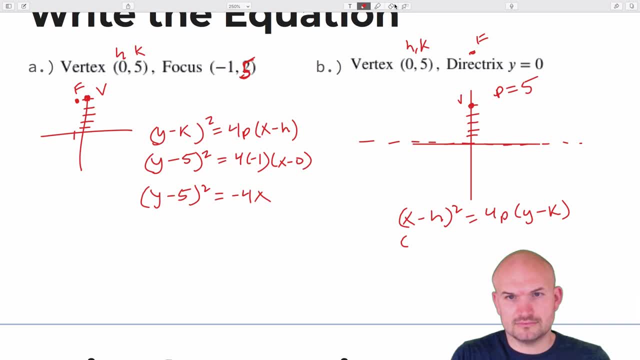 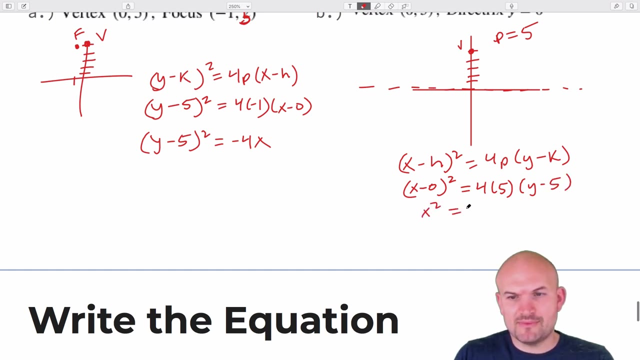 So we'll do X. So we'll do X minus 0. quantity squared equals a 4 times 5 times a Y minus 5.. And again, one thing I always want you to remember: you can always go back and check your work, right. 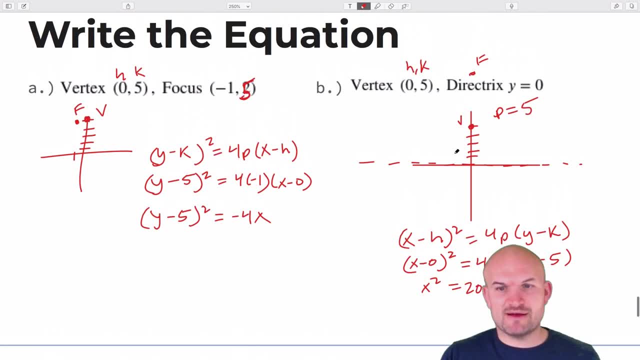 Like: all right, here's my vertex parabola. That's what I graphed. I should have a X should be squared right And my P should be positive. Yes, Here my parabola is opening up to the left. 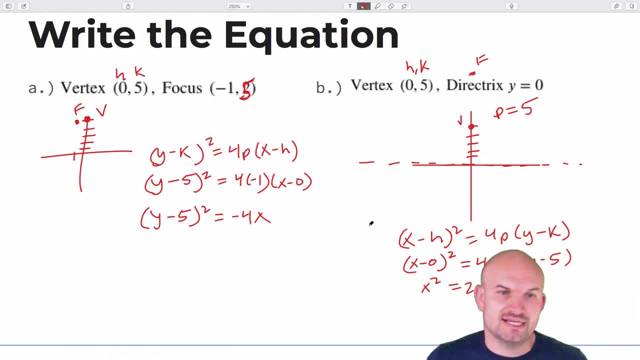 So, therefore, Y should be squared and my P should be negative. All right, So I'm going to do Y minus 5.. I'm going to do Y minus 5.. All right, So let's do that. So I'm going to do Y minus 5, which, again, you can see, is going to be correct. 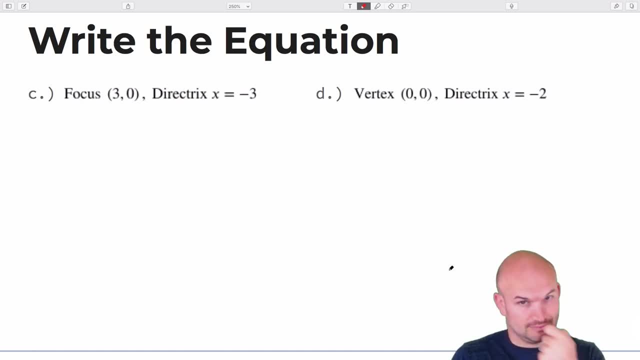 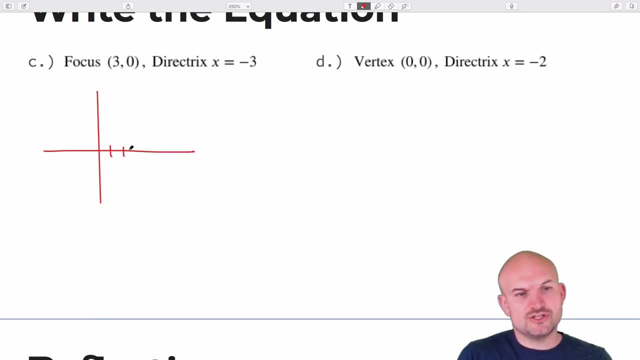 The next one, again, is my focus and my directrix. So in this case again, just plot the information. So we have 1,, 2,, 3, and then we have a directrix: at X equals negative 3,, 1,, 2,, 3.. 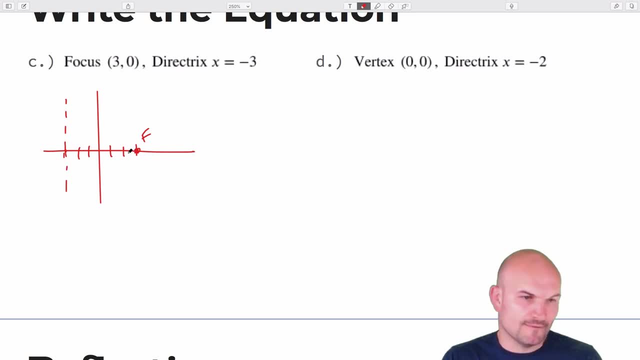 So that's my focus. Now, how should we understand the orientation? Well, remember, if the directrix is a couple of things to keep in mind. first of all, So the directrix, remember, is perpendicular to the axis of symmetry. 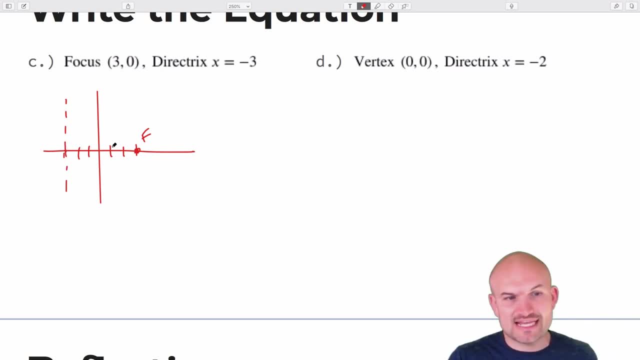 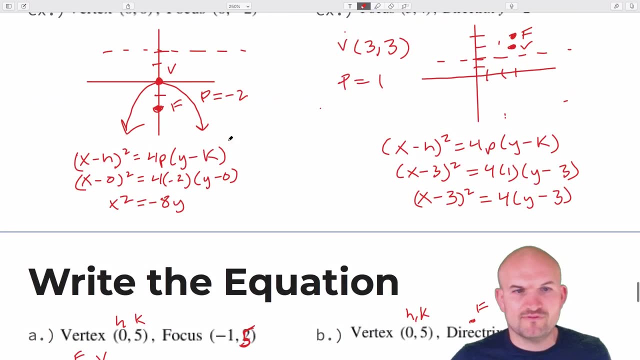 Also, the focus and the vertex lie on the same axis of symmetry, So the line of symmetry needs to go through the focus, And that's not one thing I've talked about before which is important for us to understand, though. The line of symmetry, the vertex and the focus go through the line of symmetry. 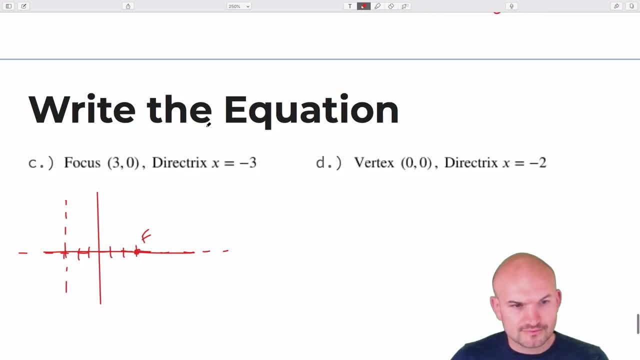 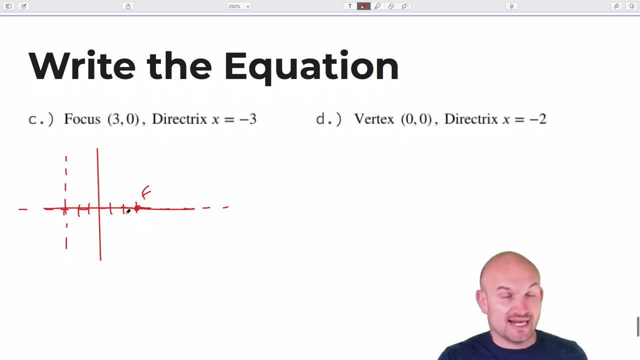 And remember that's perpendicular to the directrix. So if I know my line of symmetry or my axis of symmetry is horizontal, that means my parabola is going to open up right And it always opens up towards the focus. So therefore I know it's going to be a horizontal parabola. 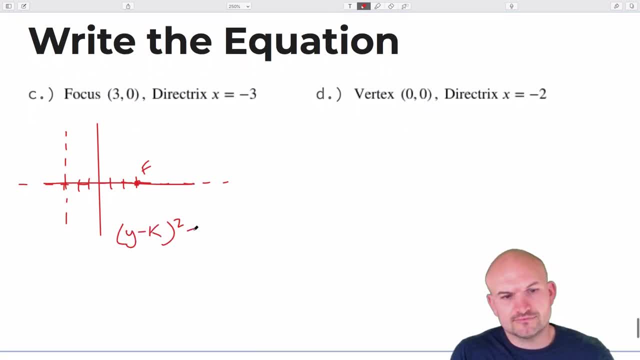 So, immediately, I'm just going to write down the general formula: Oops, x minus h. OK, so I know it has to be a horizontal. Now the next thing again is I need to figure out the vertex. Well, again, what I can do is the distance from the directrix. 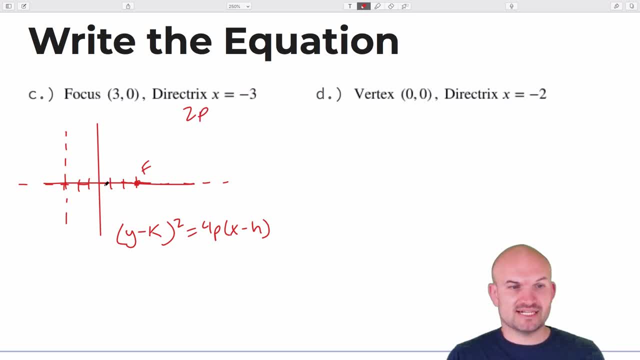 So the distance from the vertex to the focus is 2p, right? Because, remember, the distance from the vertex to the focus is p, and then distance from the vertex to the directrix is opposite of p. So if I just figured out this distance, which ends up being 6,, you could count or you could. 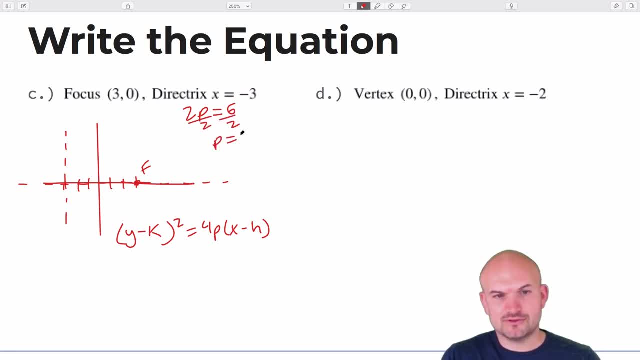 just look at these values then you could just say: all right, p is equal to 3.. That means the distance from my vertex to my focus is 3.. So where should this midpoint be? And again, if you have some problems, if you have a problem where? 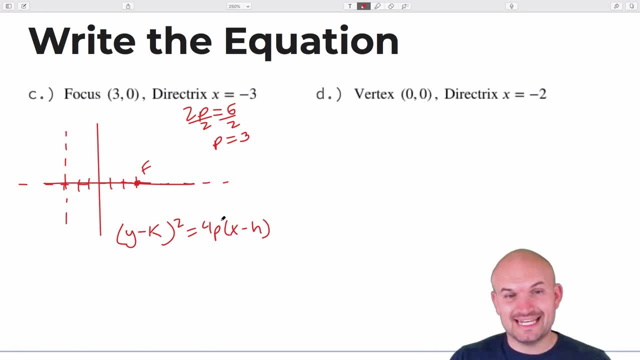 You know where it's, not at the origin. if you remember what we did in our what you need to know section, you could find the midpoint of your kind of like those two points, or find that middle point there. Just important to understand that they're going to lie on that axis of symmetry. 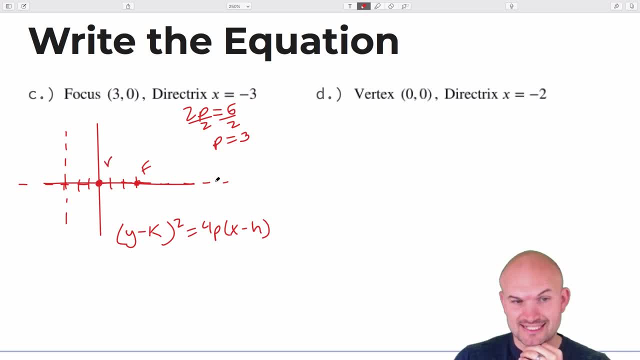 So, in this case, though we can see, my vertex is going to be right there, because it has to lie on that same axis, symmetry, And again, that makes sense here. So my origin, or my vertex, is going to be at 0, 0.. 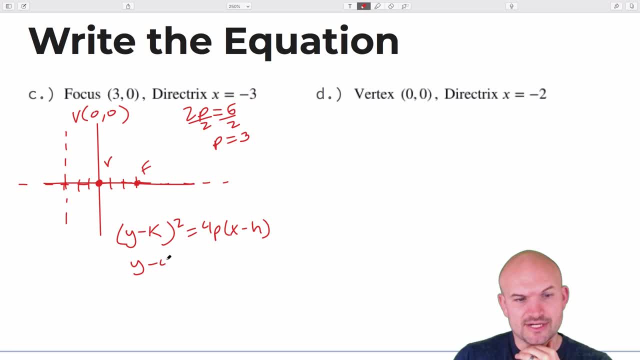 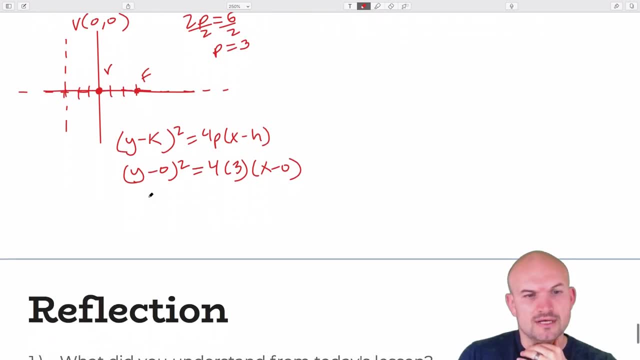 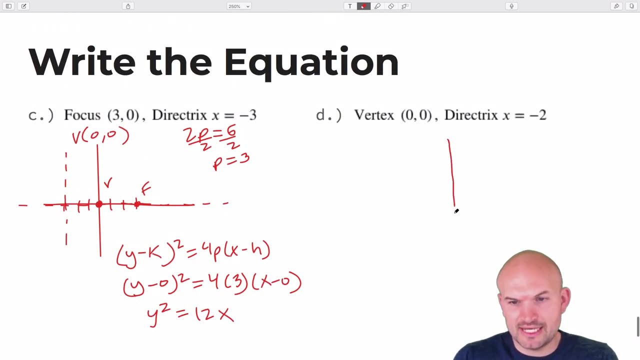 All right. so in this case I'm going to have y Minus 0, quantity squared equals 4 times 3 times x minus 0. So we'll have y squared equals 12 times x. All right, and then the last problem, ladies and gentlemen, is again going to be a problem. 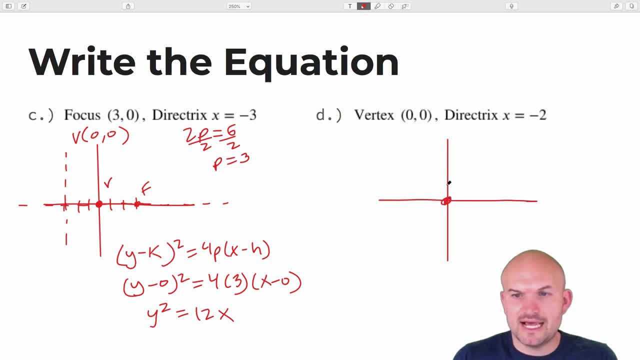 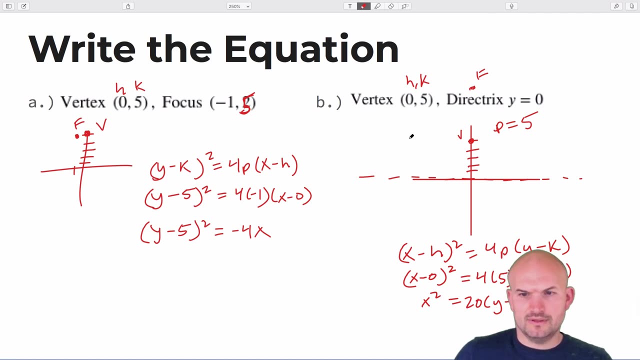 where we have the vertex is at 0, 0.. And then we have a directrix at x equals negative 2.. And did I really want a directrix at negative 2?? No, Let's do x squared, y squared, negative. 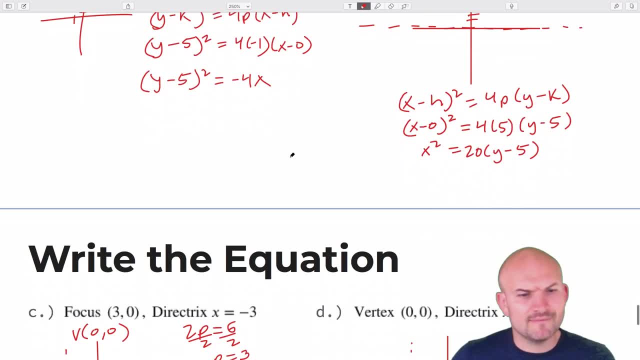 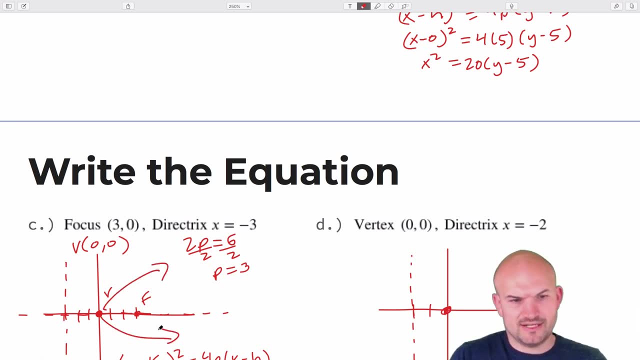 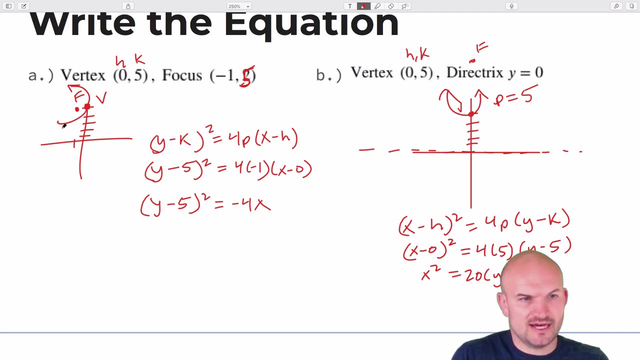 I guess that's probably what I did want. Let's see, Let's change this up here. So here we're going, positive, positive. Here we're going positive, positive to the left, to the left. So I'm going to want to have a problem. that's going. 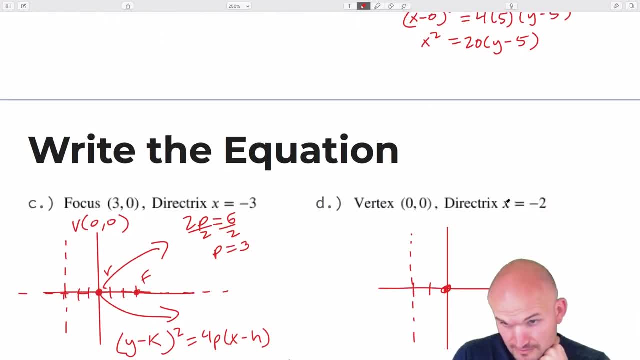 Down. So let's just actually make this y equals 2.. So I'll go ahead and change that into my notes. But it looks like when I changed that first problem that kind of messed everything up here. So if I want y to equal positive 2, now that will be my first problem that's going to open down. 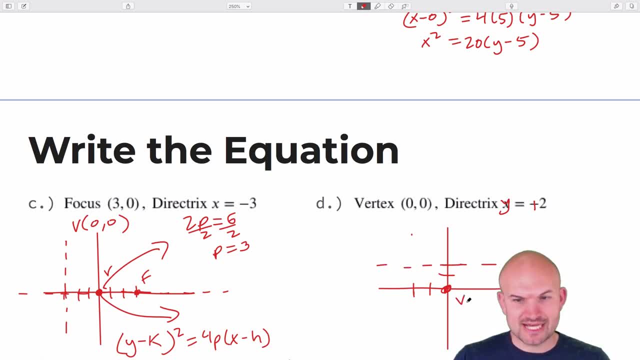 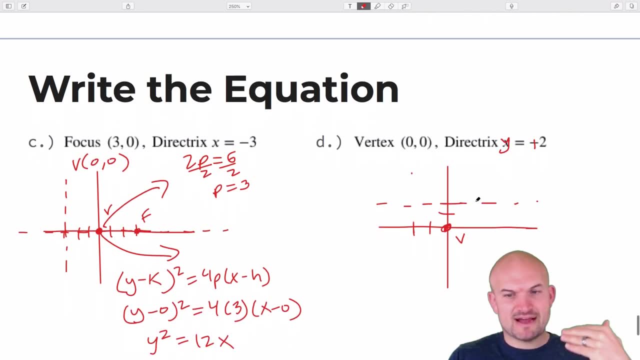 So I'll have y equals 2, which is going to look like this: This will be my vertex. And again we have vertex to the directrix. Now, again, that's going to be a positive 2,, right? So the important thing is, I know that my focus then needs to be somewhere down here. 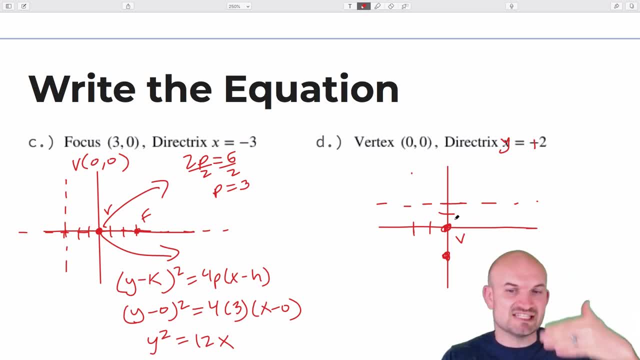 Well, if my distance from my vertex to my focus is 2, that means the distance from my vertex to my- I'm sorry, the distance to my vertex to my directrix is positive 2.. That means the distance from my vertex to my directrix is going to be a negative 2.. 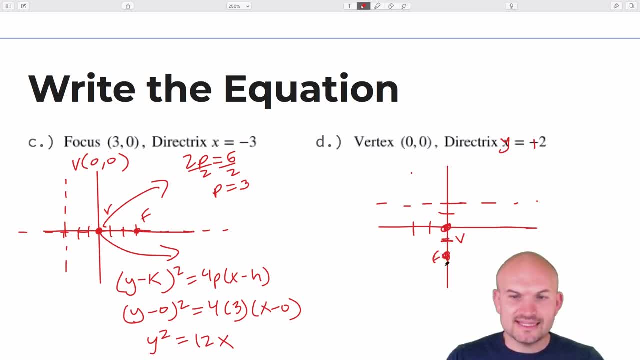 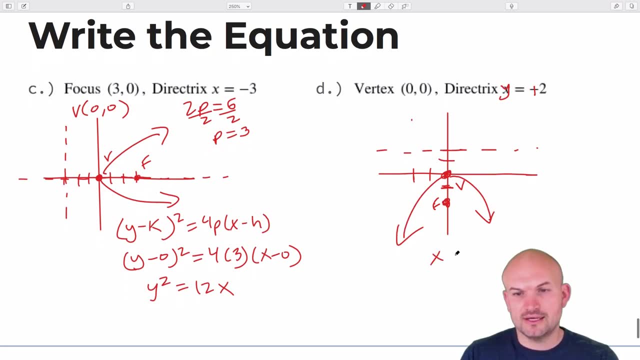 So I'm going to go down 2 units in this case. That's going to be my focus. So again, I know my parabola is going to open down, So I'm going to use the formula x minus h. Squared equals 4p times y minus k. 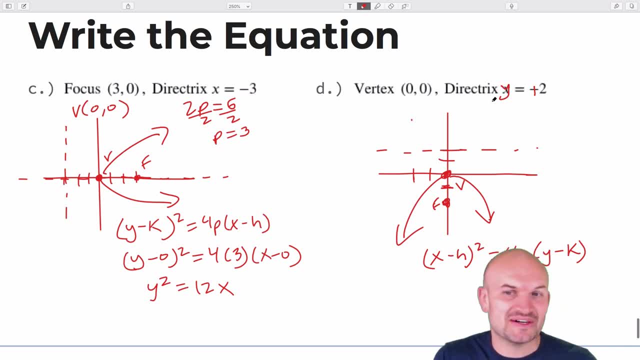 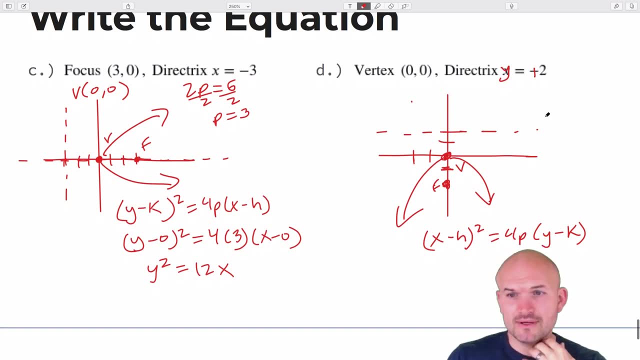 And this is why it's kind of important that I like to go through these problems in my class first. So therefore I kind of get out all those little wrinkles. My vertex is going to be at 0, 0.. And in this case we can see p, since it's going is 2.. 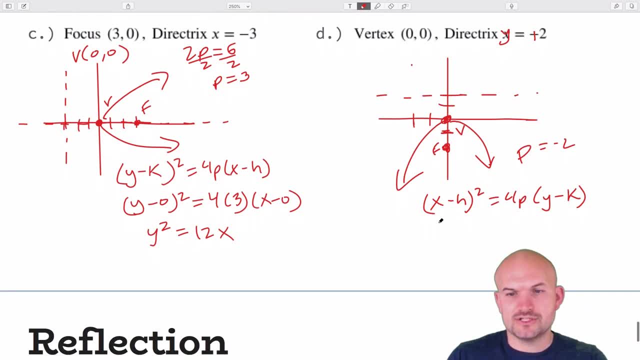 But since it's going down, it's going to be a negative 2.. So, therefore, I'll have a x minus 0.. Coin squared equals 4 times a negative, 2 times y minus 0. So I have an x. squared equals negative 8 times y. 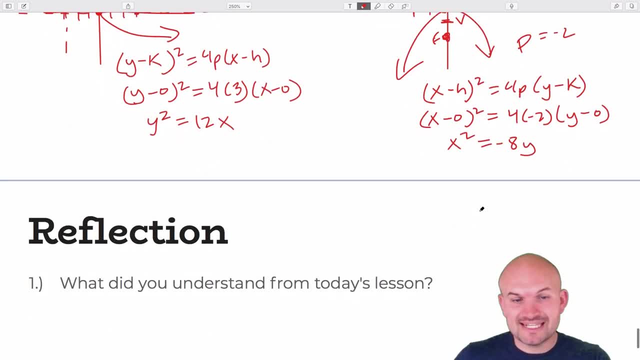 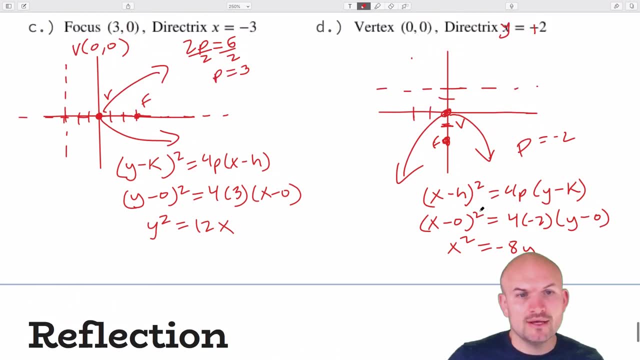 And there you go, ladies and gentlemen. That is basically it as far as our process. So if you have any kind of questions or some understandings, make sure you go ahead and add them down below. But really just kind of recap. 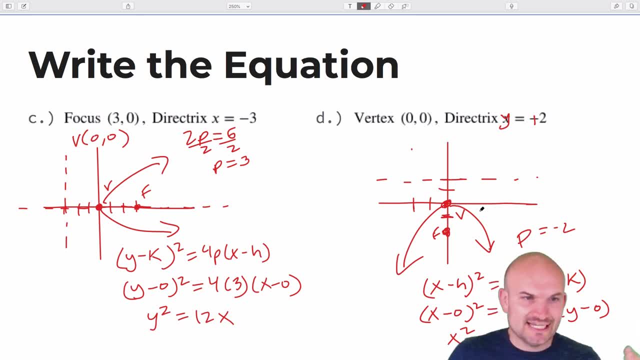 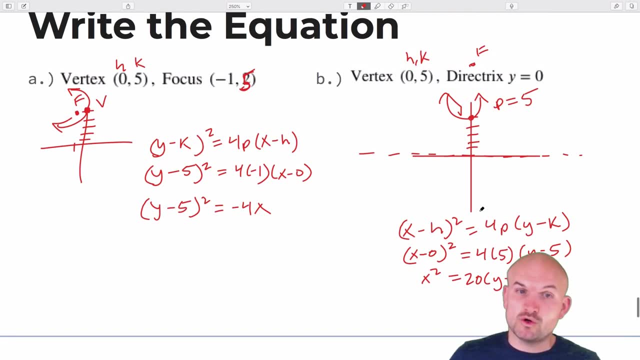 When you're given information, plot it and identify the vertex and the value of p. And remember p is the distance from our vertex to our focus, It's our focal length And it can be positive or negative depending on the directions. And then